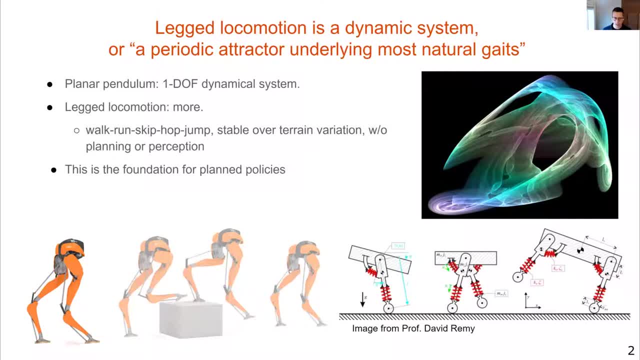 of every talk. but um, legged locomotion is a dynamical system and the way i view this is, um i don't know, analogous to a pendulum. a pendulum is an interesting corner of dynamics. there's no software control on it. it keeps time the way it is. uh, legged locomotion on the lower right here i 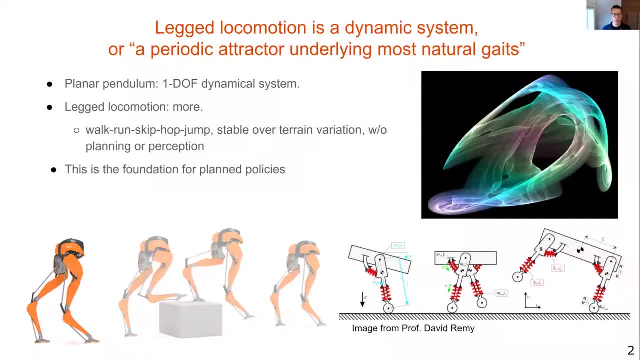 have a image from david remy's work where he showed that spring mass systems can reproduce every single natural gate. uh, that exists um, bipedal, quadrupedal, etc. uh, and that's, that's quite a coincidence, right? um, it's not really a proof necessarily that all legged 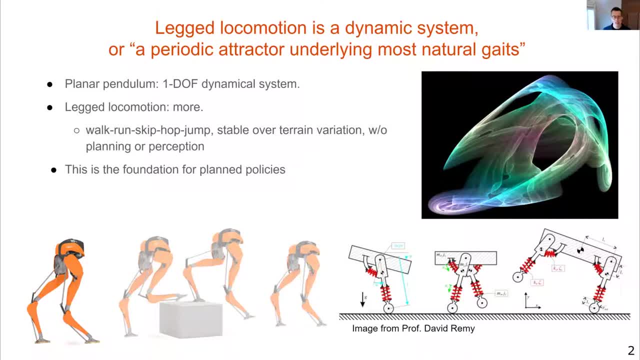 locomotion is based on this, but it's quite a coincidence, uh- and this is sort of enough for me to really believe in that. uh, i think of legged locomotion, um, maybe this periodic attractor where i don't know how many degrees of freedom there are in it- seven, nine, but it's got kind of. 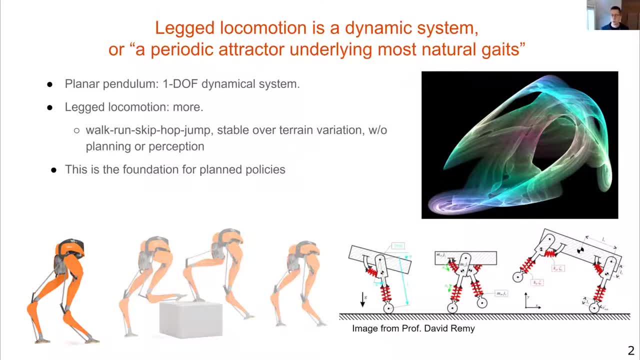 some cycles that it likes to come back to, which makes it very robust if you implement it. well. we found this with uh, with some of our early tests and with atrius. once you kind of settle in on this spring mass behavior, it can just absorb all kinds of disturbances in the world with really no 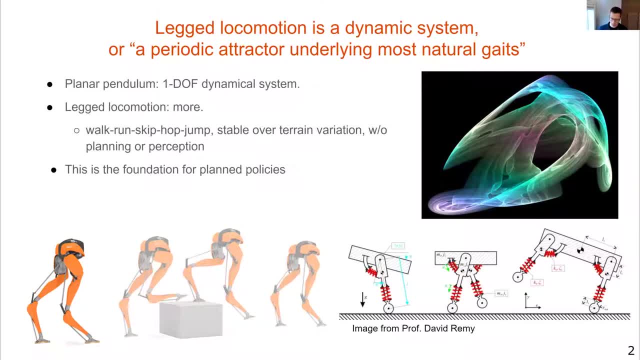 control input, um, no, perception and sensing and then thinking about it. but you do have to get kind of the dynamics right. you have to settle on the right dynamical system and we have approximations of what that is and if we're able to get, you know, some kind of spring mass system, that's pretty close. 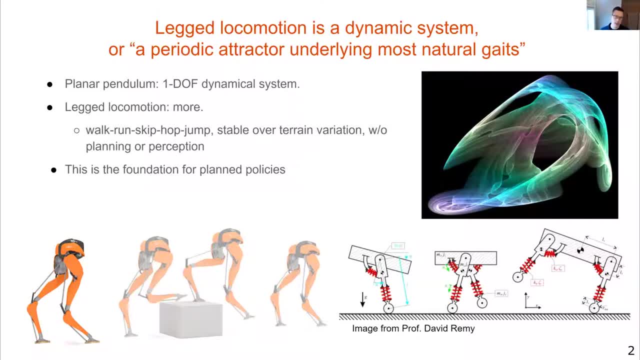 we don't have a complete description of it, but that's why we think of maybe, maybe learning this system- uh, learning a representation of this system. if we're able to put in the right cost functions and the right constraints, we kind of know what the answer is. we know how the system moves, we know what. 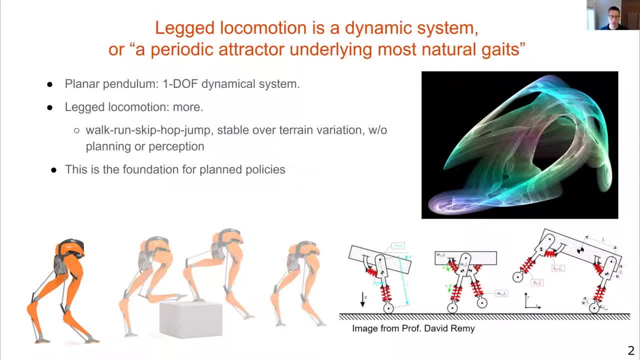 how it should respond to disturbances. we know a lot to describe what it should do, but representing it is is very challenging kind of the direction that I'm looking at this. It's very different from saying I know I want to put one foot in front of the other or I just want to control this to be stable. I'm having a. 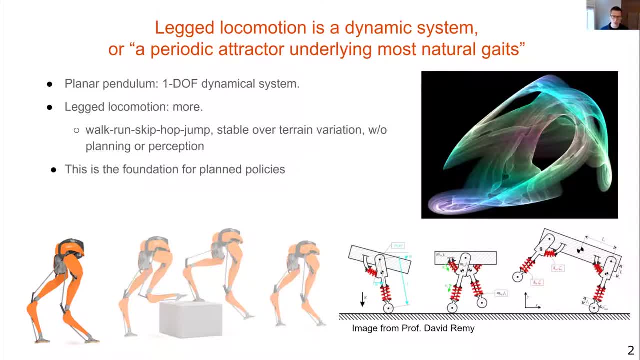 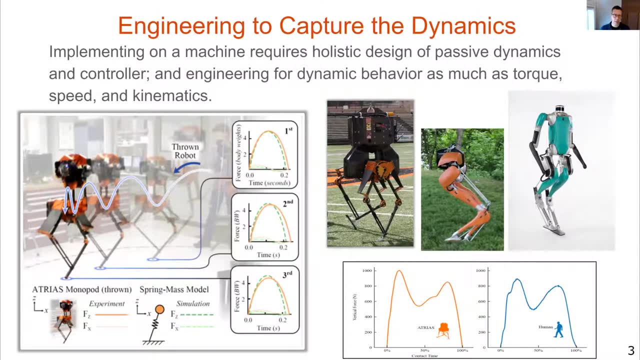 definition for stable. I'm really trying to discover a way to represent this periodic attractor. I guess I mentioned it a little bit, but the first robots we were doing were really focused on understanding this spring mass model, which was a representation from biology. 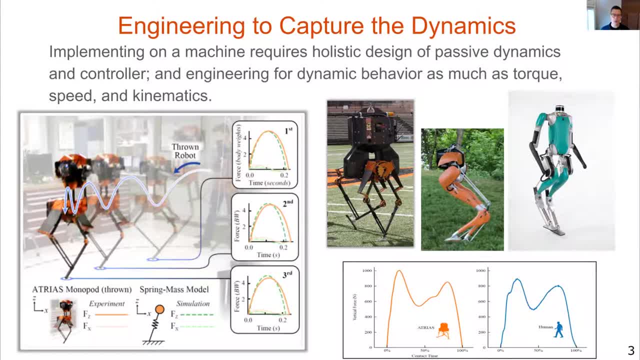 and then implementing that on a machine to really capture the dynamics. In the lower right here you can see the ground reaction forces of Atrius. compared to a human, You can see they're awfully close. That was our force plate, my graduate student, Christian. 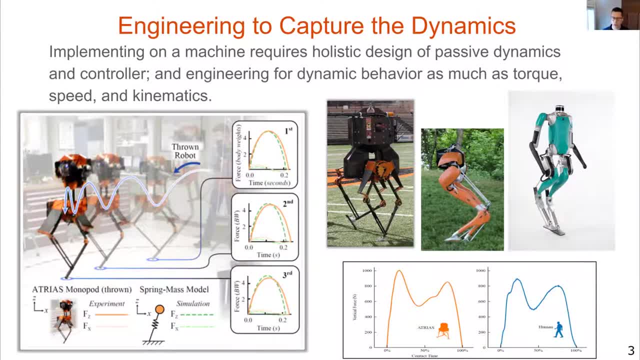 Hubicki walking across the force plate in blue and Atrius walking across the same force plate in orange. Our controller was just a heuristic set of controllers. It was not special. It was tuned in a little bit Once we had it working in the lab for the first time and then we took it outside for the first. 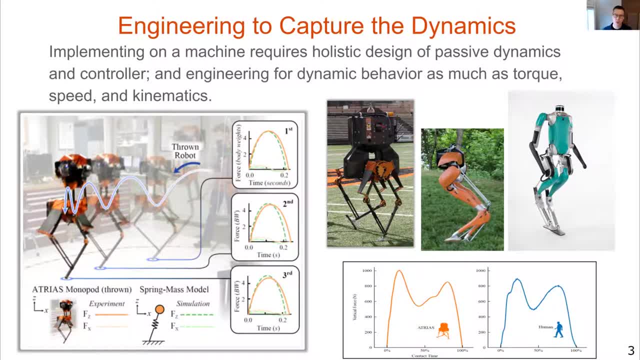 day we spent an hour or two using up the battery, just walking up and down hills and over hillocks and bumps in the grass and over all kinds of things. It was very stable because we were utilizing these kinds of spring mass dynamics that are inherently robust to the world. 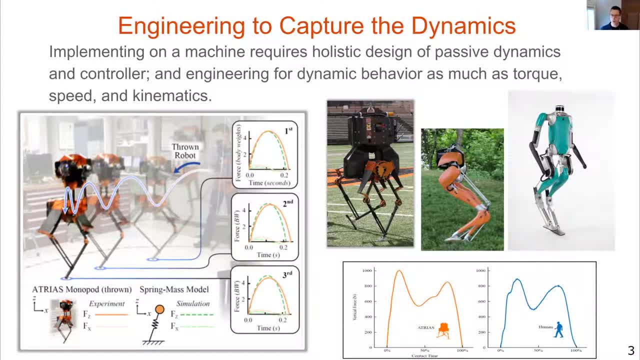 The way we built that. you have to design the machine for it. We understand the behavior you want. We designed the machine to create that behavior. We designed our controllers around that machine, around that behavior. It's very holistic. You have to design the whole system up and down. 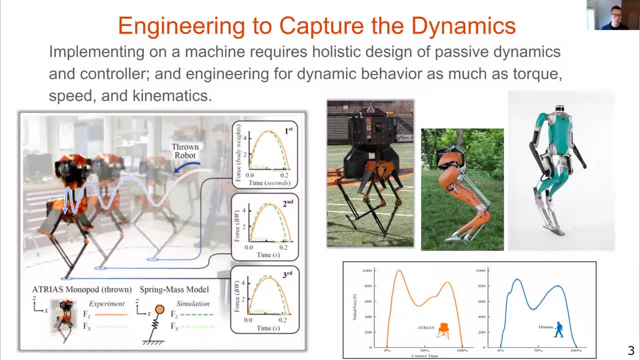 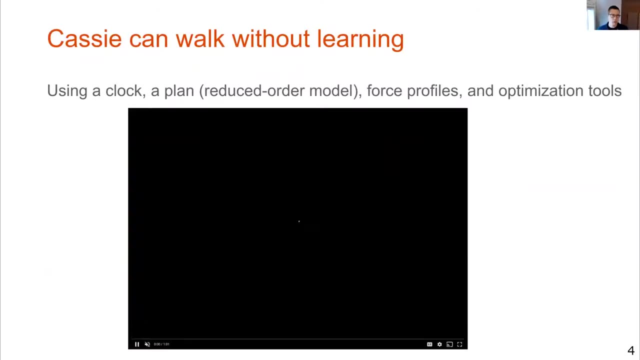 for this behavior, for this dynamical phenomenon. We're doing that also for CASI, for Digit, for all of our robots. Our controls are just getting a lot more sophisticated than they started out with on Atrius. CASI can walk without any sort of learning. of course We're using 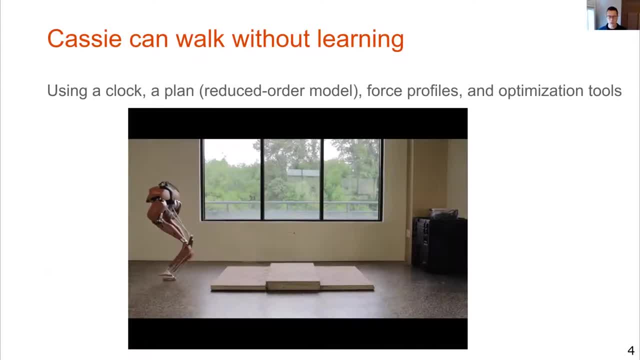 basically a reducer. It's a reduced-order model. In this case, I think it's a linear inverted pendulum for horizontal foot placement, plus a little bit of a heuristic for what the z-axis should do. We're commanding forces on the ground based on that reduced-order model and a clock to. 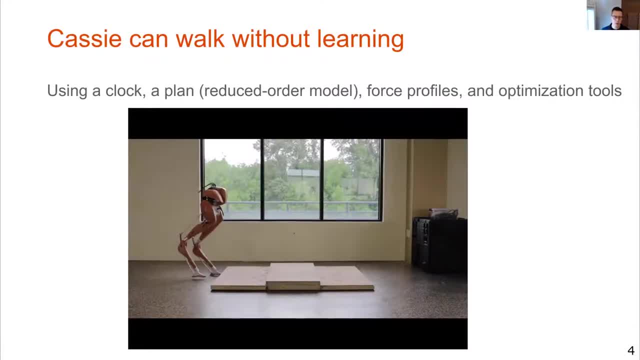 determine what the footsteps are, and then some optimization tools that basically try to get this fairly complex inertial system to behave close to what the reduced-order model is commanding it to do. That kind of describes out a control hierarchy We've got, of course. 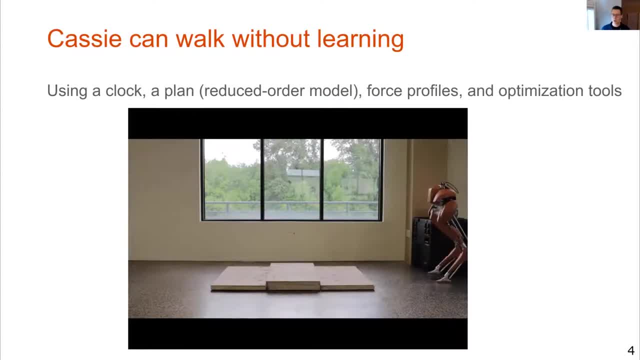 the hardware system which is designed to walk and run. It's got all the inertia's in the right places. We've chosen the links carefully. We've eliminated antagonistic work. We've added physical compliance to absorb the impacts with the ground. Then we have super low-level controls. 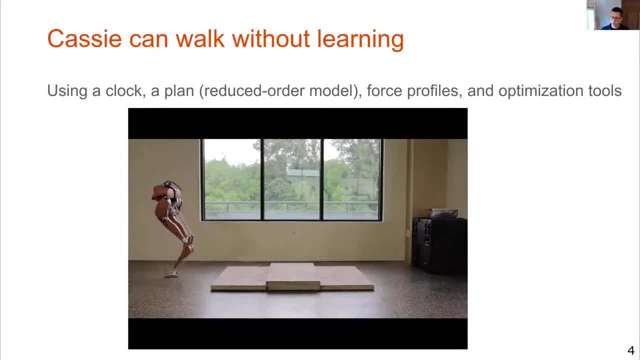 like inverse kinematics, where we're just committing torques to individual joints and relating that to task space, where you want the end effector and what forces you want to apply, And then above that is the reduced-order model and above that would be planners and 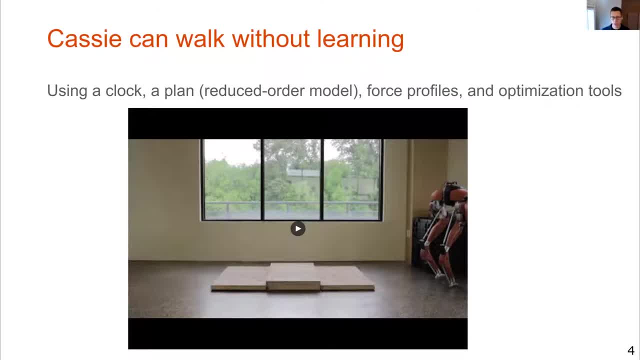 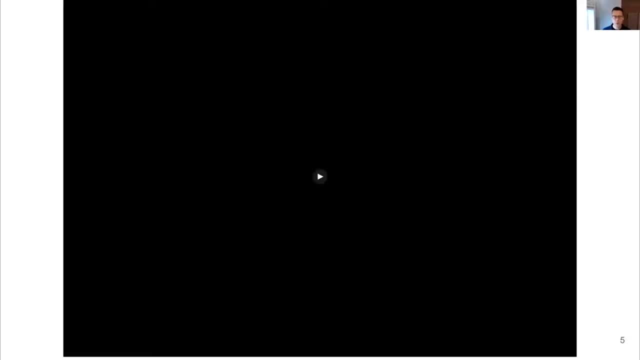 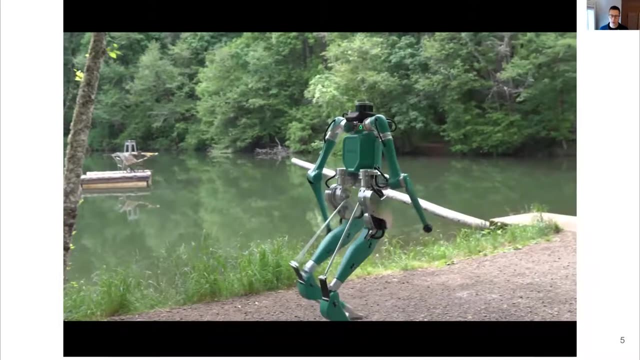 things. In this case there's no perception, There's no idea of where the stairs are or anything like that. That would be higher levels on the hierarchy, But there's a whole control hierarchy. Here's Digit. This is the same exact control, but now on Digit And now the optimizer. 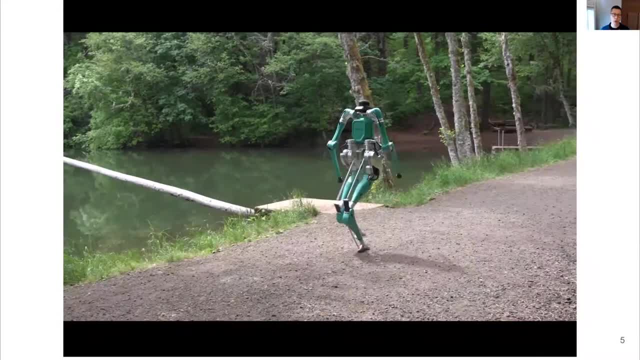 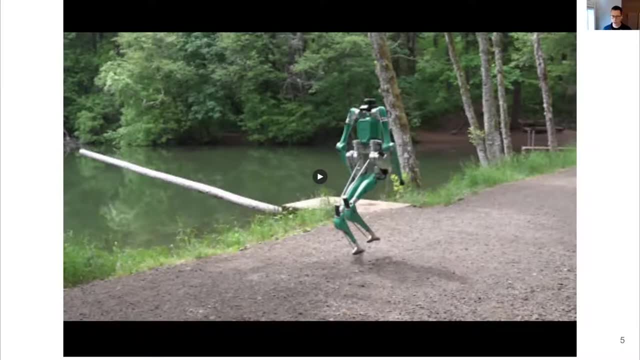 can do things like swing the arms to deal with inertia. We find one of the big failure modes actually of CASI or Atrius walking is that the robot will twist, And so we have a couple of different ways to do control authority. One now is we have the feet so that you can apply some. 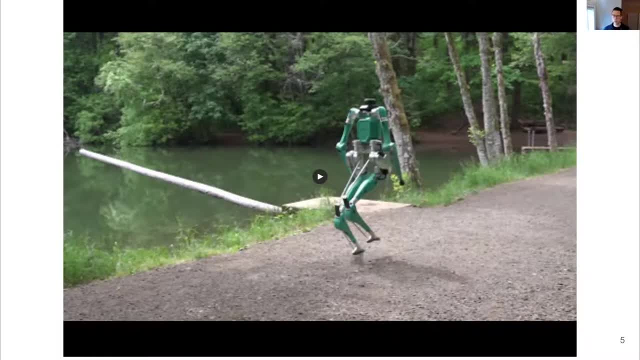 torque to the ground And we have the arm swing which allows you to. when the robot gets pushed, it swings its arms to have inertial actuation for the control of yaw. So we're starting to increase the things we can do. but it's the same control hierarchy, It's the same kind of reduced-order. 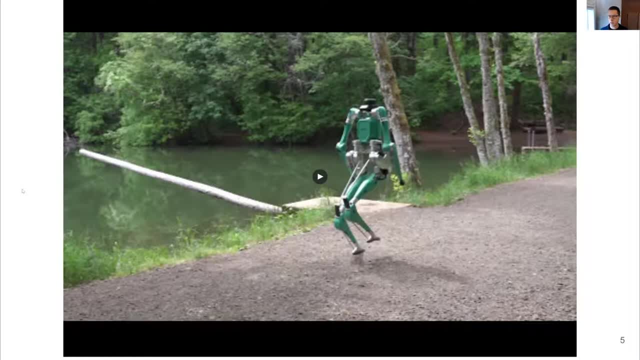 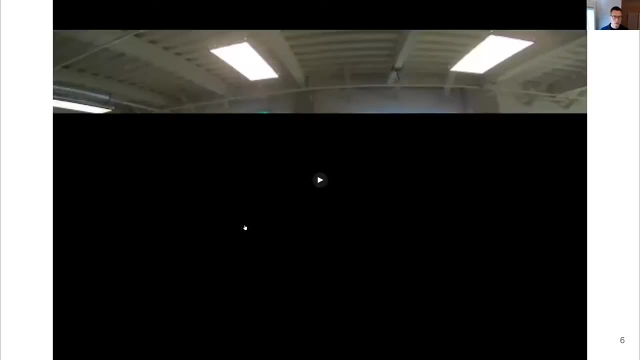 model the same optimizers choosing doing. By the way, if anybody has any questions, especially clarification as I speak, please, I welcome them. Just jump in and let me know Now, with the control hierarchy that I was talking about, when you then start to add on. 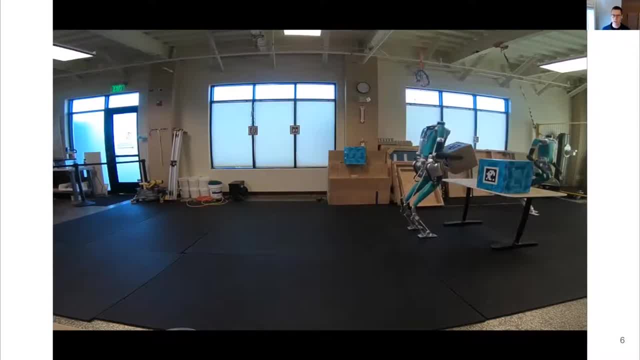 doing things in the world you can Here- now we have some perception. that's identifying the fiducials on the boxes and on the walls so that the robot knows where it is in the world And then sending on fairly simple commands for direction and velocity. 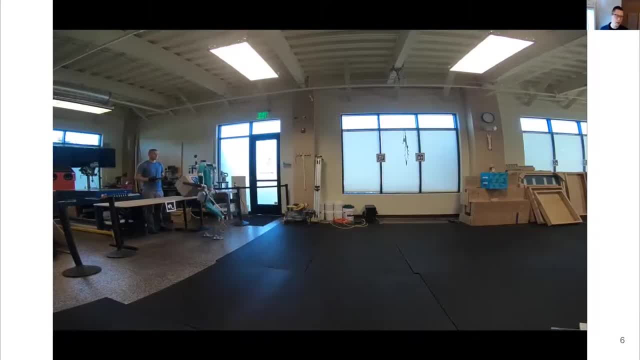 And then still working with the reduced-order model and then the QP optimizer, that's, In this case, when it's holding the box. now it can use the box inertia to swing back and forth to control the yaw and other things about the dynamics of the gate. 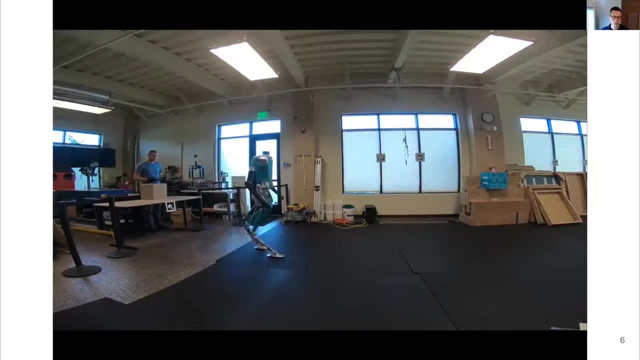 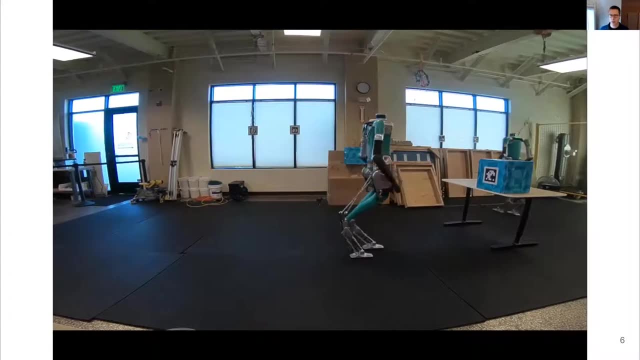 to try and get it kind of close to what the reduced-order model is asking it to do. So this kind of control hierarchy, I think, is inherent. You're going to have to have this for robots, whether or not you're going to use learning or model predictive control or whatever. 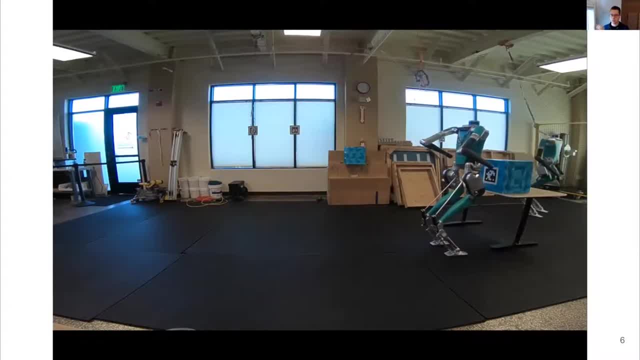 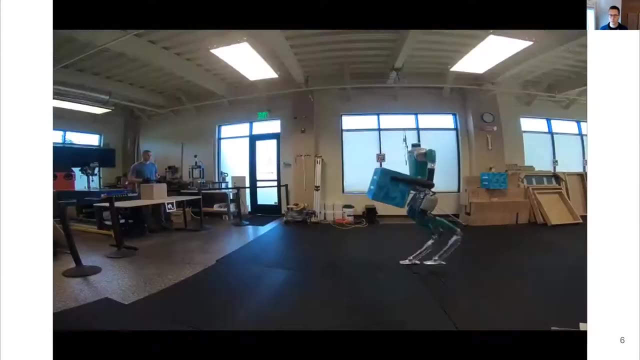 it is That's going to be pieces of the control hierarchy, And especially learning, is kind of a black box. So you want to have a small black box where you're very confident what it's going to do for the entire set of inputs that you would ever give it and have it be pieces of the control. 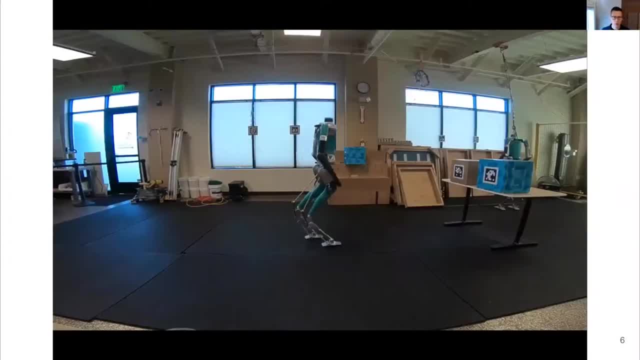 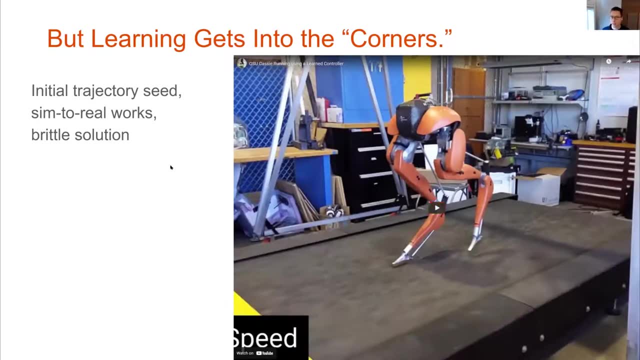 hierarchy. Okay, So the real benefit of learning is that it gets into the corners of the dynamics. I talked about how we're using this reduced-order model. Well, that really limits kind of what the machine can do. The steps are maybe a little bit short. They're not utilizing Certainly. 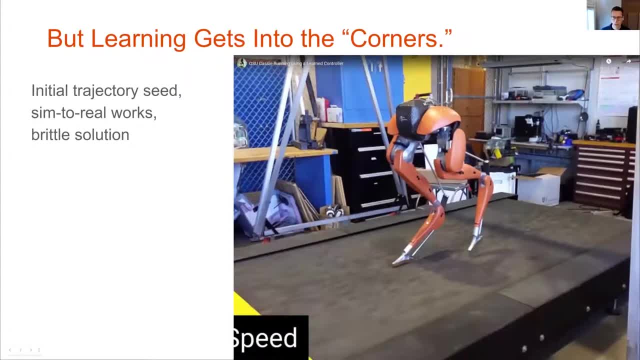 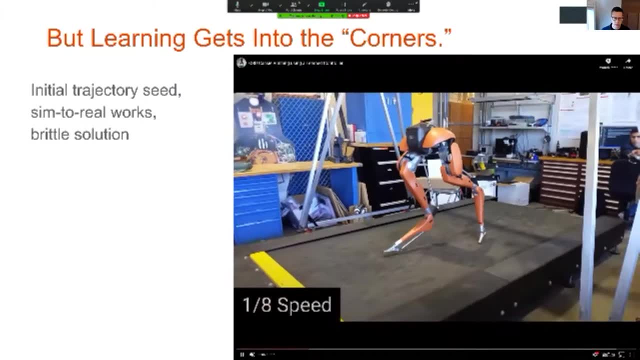 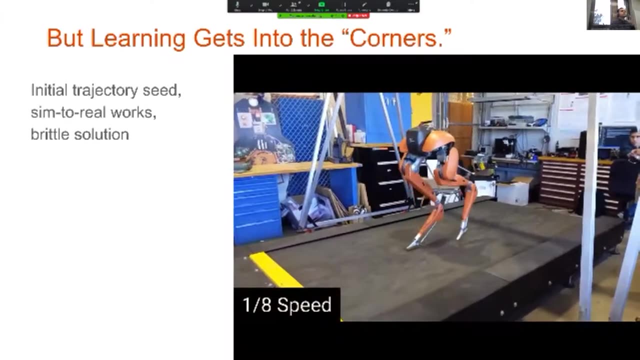 not utilizing the full dynamics of the robot, And so if you watch this gate, By the way, now I'll optimize for video clip. Did that improve the video a little bit? Yes, it did Great. So here you can see that the robot is landing with its feet, kind of pointed out. 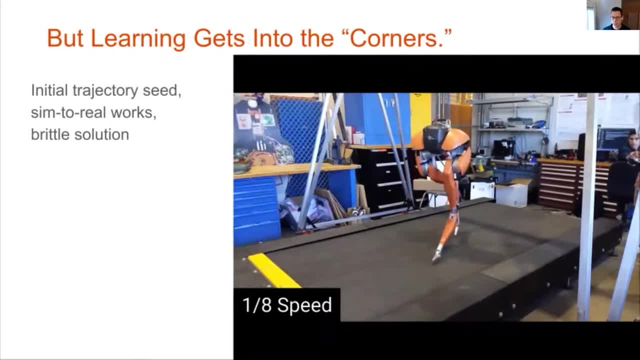 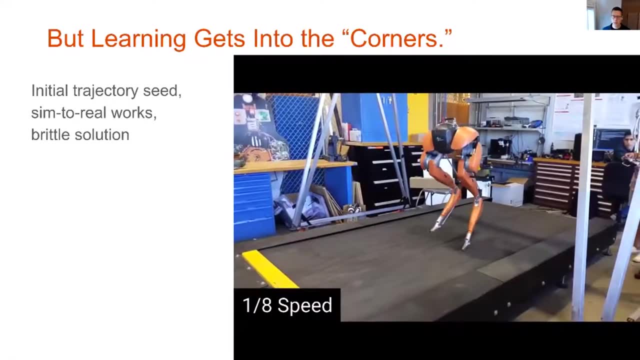 and twisting them in as it goes. And that's because Cassie here has no inertial actuation Right. It can't swing its arms, And when it swings that leg forward it really wants to twist the body. And that's really hard to get up to high speed, But with 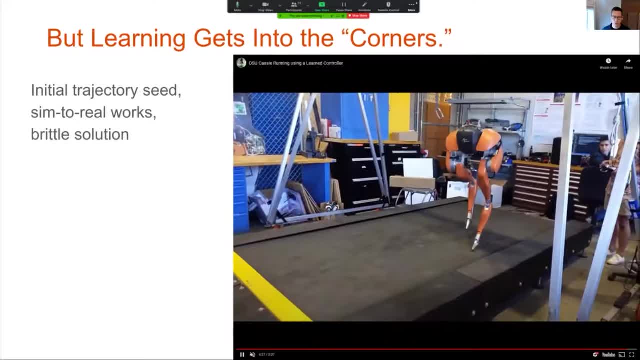 the learning system. Cassie has more of that and more flexibility. She can do that weird stride right And she can sort of take the long way up to the top of the robot And then she can try to keep and it actually learned to do some interesting stuff with the leg: to twist the leg as it swings. 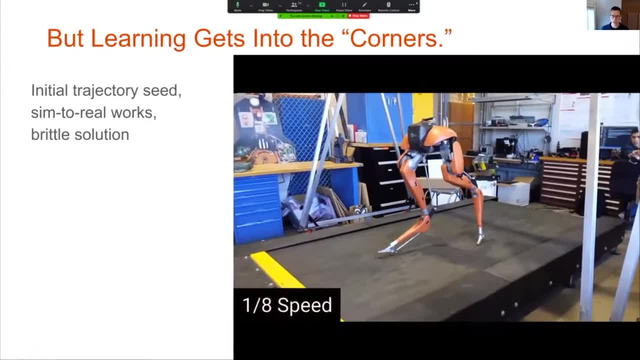 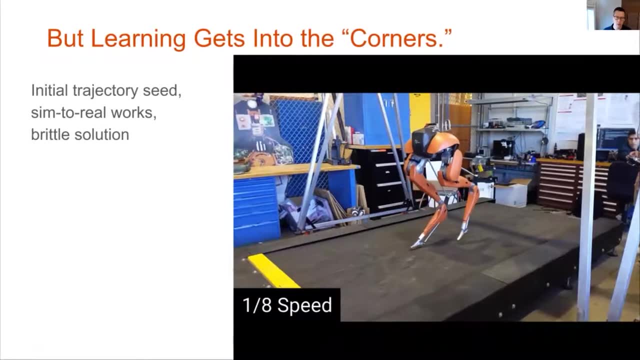 the leg out to twist it out, step on the ground and then twist it inwards as it goes And those kinds of coupling things. that's just an example of something that's very hard to do with a reduced order model or some simplification of the system or write it down as an equation, But it can be. 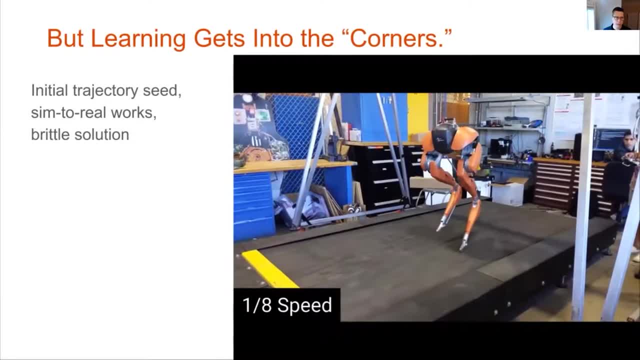 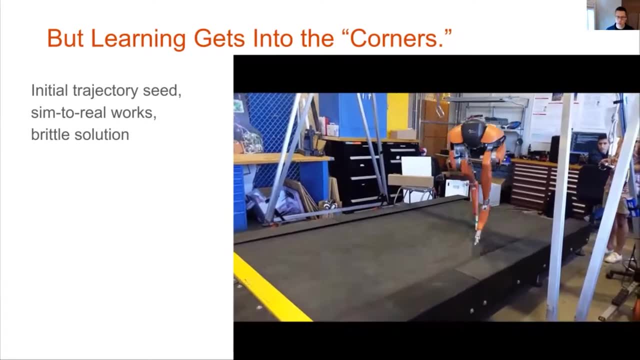 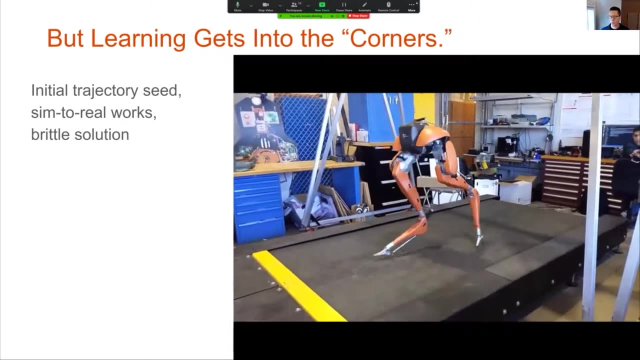 represented as a neural net when we're learning it. Now the problem here is: this is really brittle. We had this going pretty well on a treadmill but taking it outside to go run. we were on just a regular road And just the crown of the road. 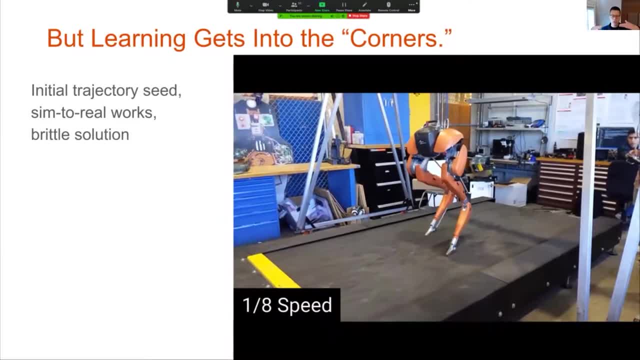 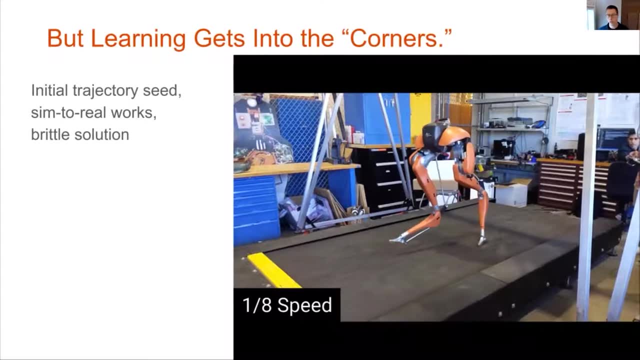 which is very, very slight. the slope of the road towards the edges was enough to completely destabilize this behavior. It couldn't handle ground that was slightly off of flat Because we hadn't trained it with that. So there's a lot to figure out with getting. 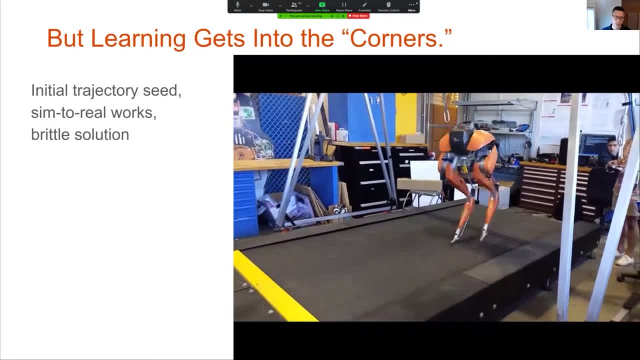 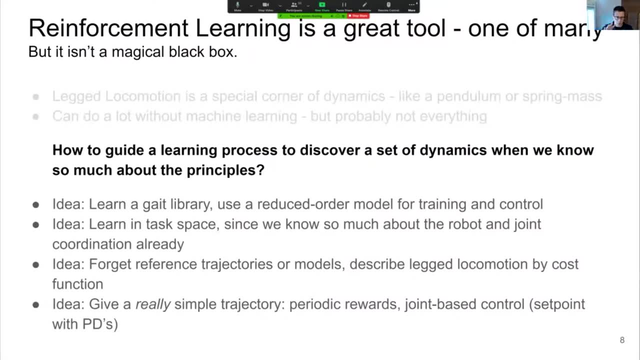 learning and doing the sim to real and making it robust to the kinds of disturbances it's going to see. So I think that the take-home message of the whole talk here is that reinforcement learning is a great tool, but it's not a magic black box. It's like there's a lot of tools to build up the whole. 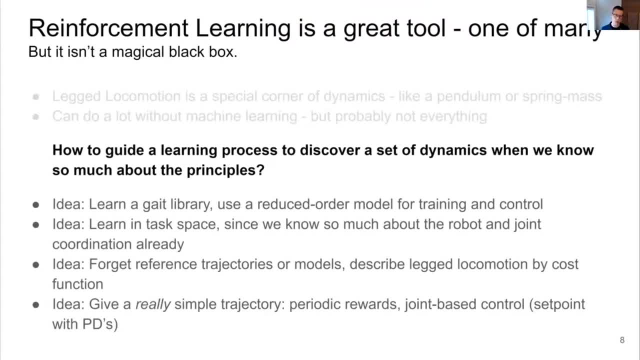 control hierarchy for a robot And you can insert learning here and there and there to really improve things. And the question now, the research question for us, is: how do you guide the learning process to discover the dynamics when you already know so much about what you want? 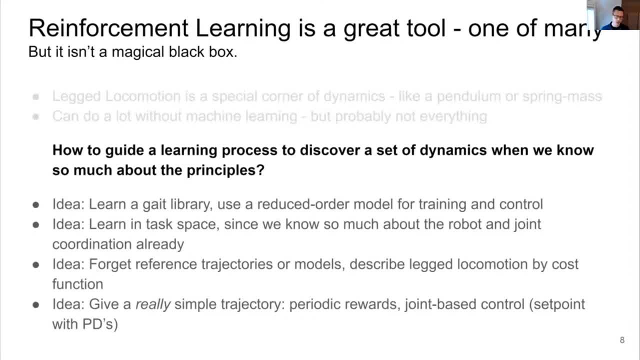 We don't want to use learning. you know, the worst case scenario really for controlling this thing or for using machine learning is to say, okay, you set up the whole problem, you set up all the constraints, and then it spits out a solution And you say, well, that must be the optimal solution. 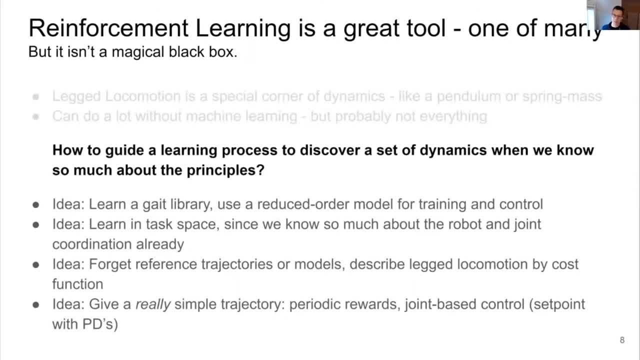 That's what it came up with. I don't quite understand why, But that seems like it works. Instead, we kind of take a very scientific approach to it, where we like biomechanics, but like biomechanics do when observing an animal and trying to understand. 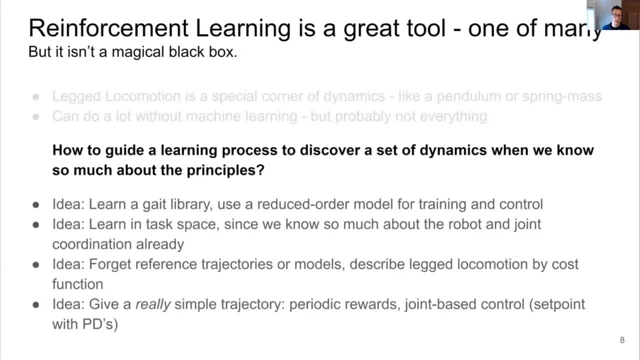 what they do and how they do and why they're doing it and what the principles are. You know, that's how we look at the results, But we already kind of know what the results should be based on: biomechanics studies based on first principles of liquid locomotion. 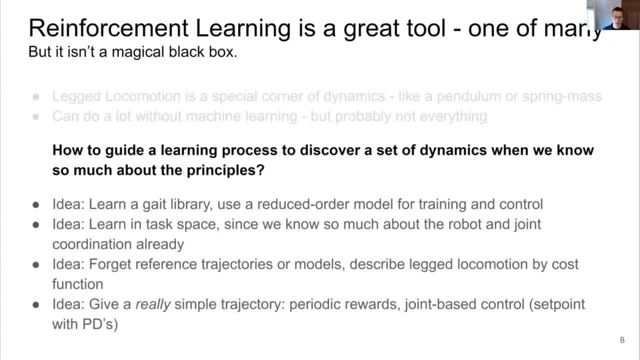 And so you know, we try to take a very small problem for the learning process, know exactly what the answer should be, but the difficulty is in representing it with models, and so the the learning process then allows us to represent it well in a weird non-linear way. so a couple of ideas, and i'll go through them. is you know first. okay. 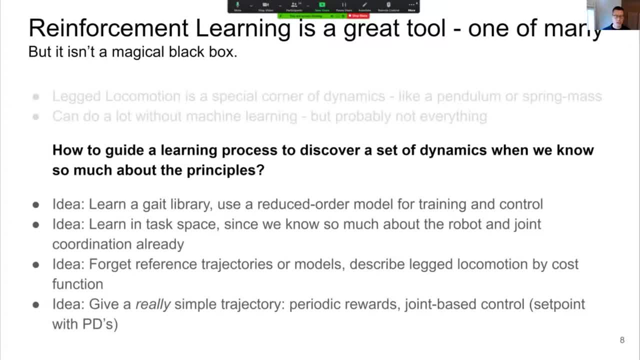 learn a gate library and then a reduced order model is kind of an input to that. you know gate library, but you've learned how to take the reduced order model as input and then put it on the robot, get into the corners of the dynamics. another idea is, instead of relearning, all of your inverse. 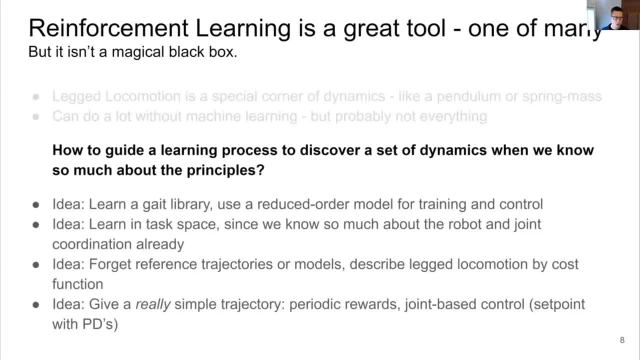 kinematics and inverse dynamics and things like that that we already kind of know about the robot- facts and information that we already know. don't make the system relearn all that. instead, learn in task space and then still use your inverse kinematics and your estimator that that work. 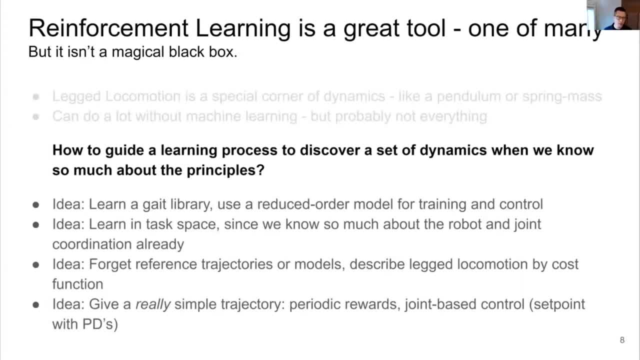 using other methods. another idea is: you know, reference trajectories and inputs can be problematic or can provide either too much or too little information, so let's instead try to give it like a really simple, um, just careful cost functions in what we do and see if we can come up with it that way. and then another one is: you give it a really 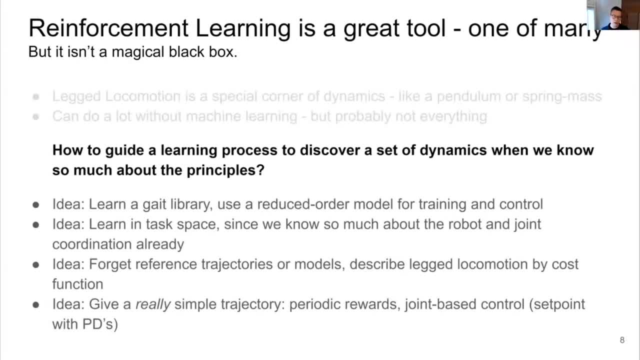 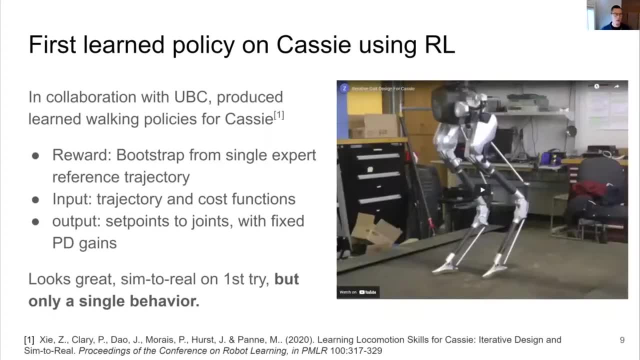 simple trajectory which is basically just a clock, input very little information about it and see what happens there. so i'll go through those, those ideas here. okay, so this is the very first learned policy on cathie, on using reinforcement learning, and this is a collaboration with Michael van de Pan and students at the University of British Columbia and produced some of the 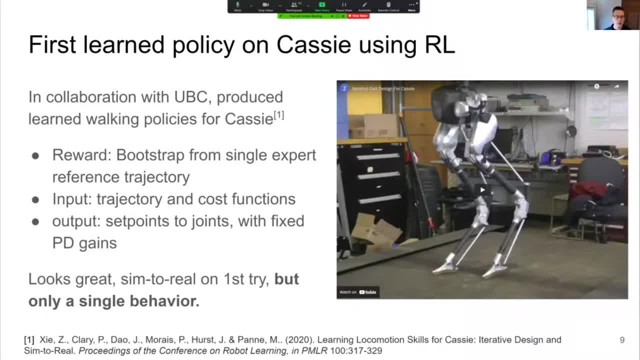 first walking policies that were learned for Cathy, And then what we did first was take the walking gates that we had developed and engineered by hand, use the trajectories and the outputs from that, which were physically realistic right, Which is important If you start with a trajectory. 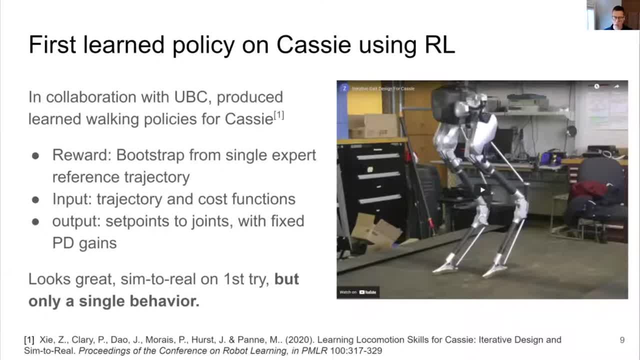 that the robot. that wouldn't physically allow the robot to walk and then try to learn from that. it's not a very good seed, But we started with trajectories that do already work. So the learning system then already has a reward for it because it's working And if the robot falls, because it's 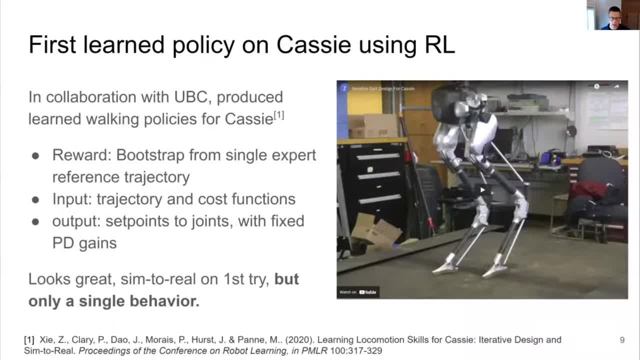 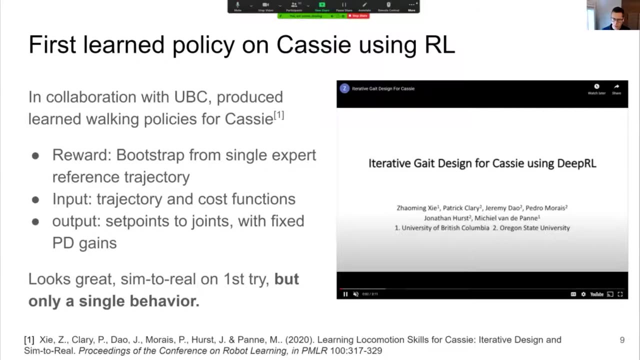 changed the policy a little bit then of course it veers from that direction. That allows us to kind of stretch the initial working controller to change the speed and a few other things, And so here I'll show that video. Give it a moment. 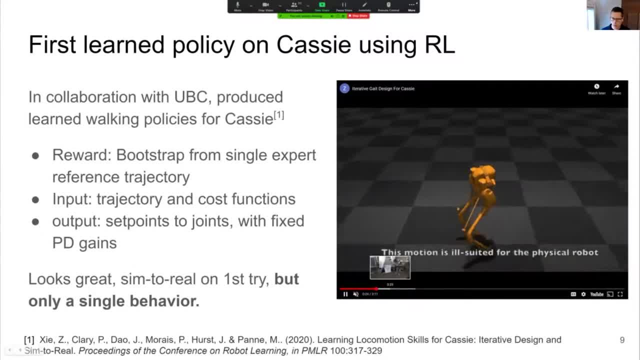 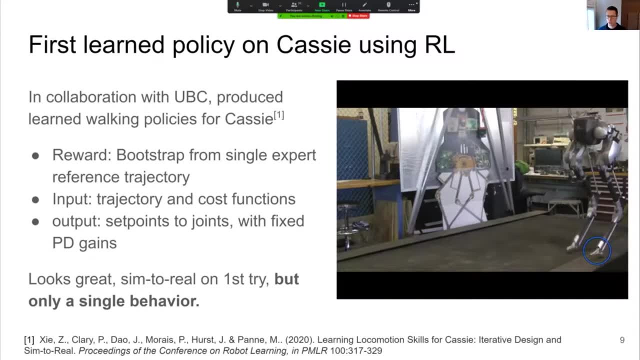 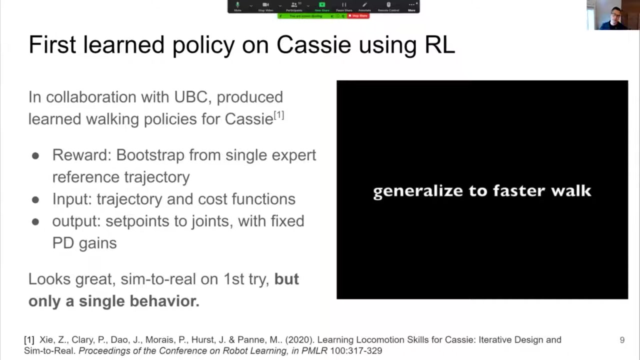 Here we go. You know kind of works And it's reasonably robust to some kinds of disturbances as well, But it was really interesting to see what it was trying to do and what it was sensitive to. The thing that was really exciting about this is that it worked on the robot. 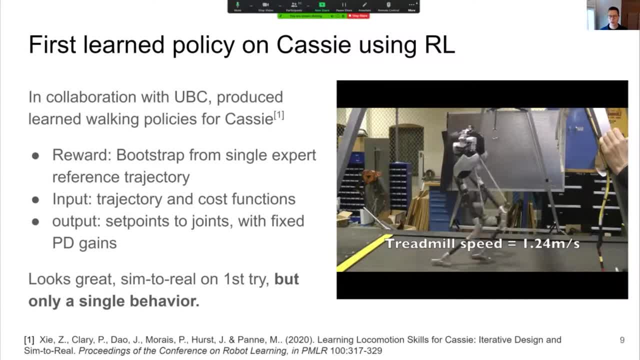 You know there's a lot of differences here. You can see it's got a bit of a limp, for example. That limp doesn't exist in simulation. Probably the left leg has a little more damping in its transmission than the right leg, or something. 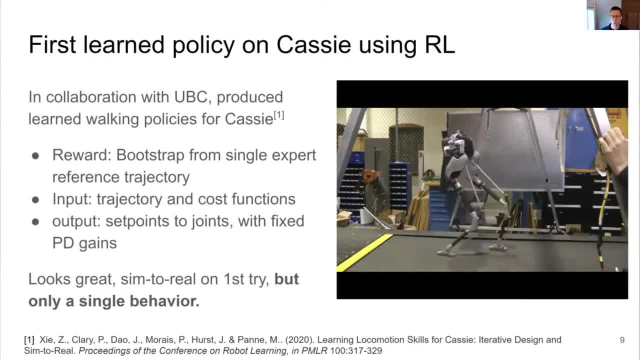 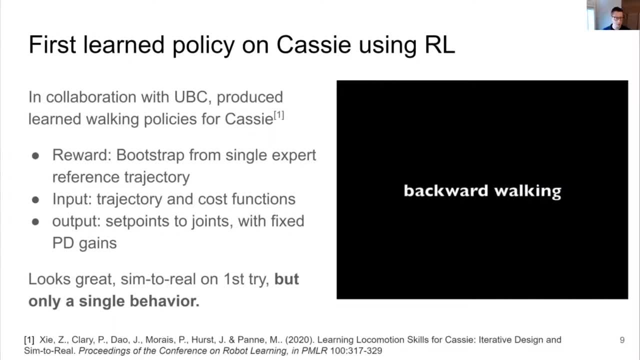 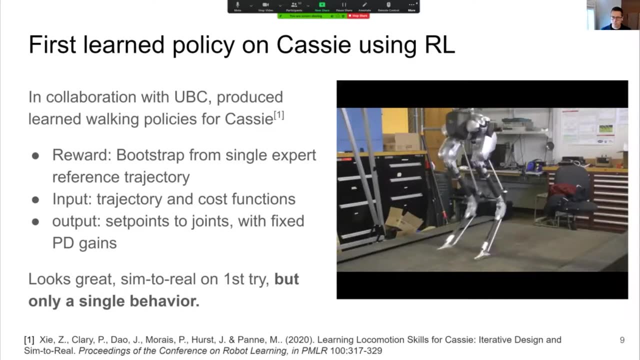 like that that causes this. There's all kinds of variations that happen in the real world that don't show up in the simulation, which, if your policy isn't robust to it, is going to really mess with it. Okay, Okay, So the next step was: 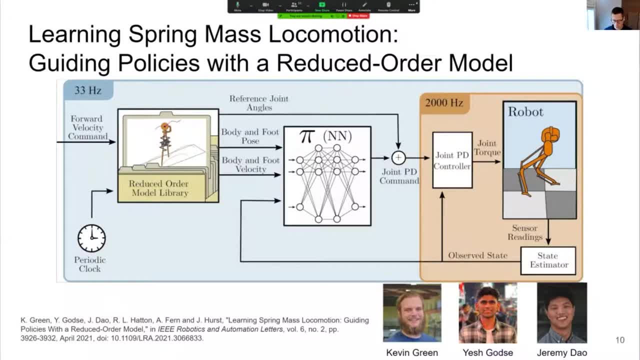 to start guiding our policies using a reduced order model. Now this mirrors pretty much exactly the way I described the control hierarchy at the beginning. We said we have some reduced order model and then we use an optimizer and inverse dynamics and so on on the machine to implement what the reduced order model is trying to do. 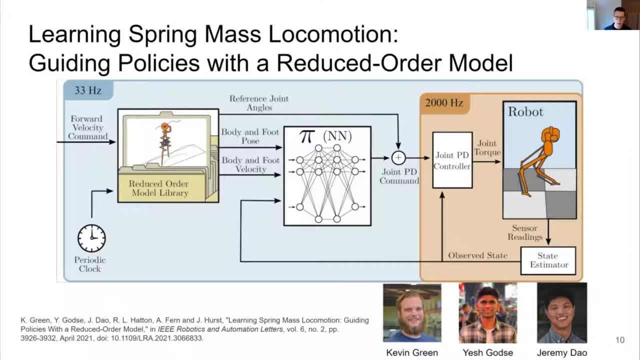 But the other thing we can do is learn a policy where- and this is an important distinction- the policy on the output of the robot is not going to try to reproduce exactly what the reduced order model is doing. Instead, the reduced order model is one input, along with the state of the robot and other things. 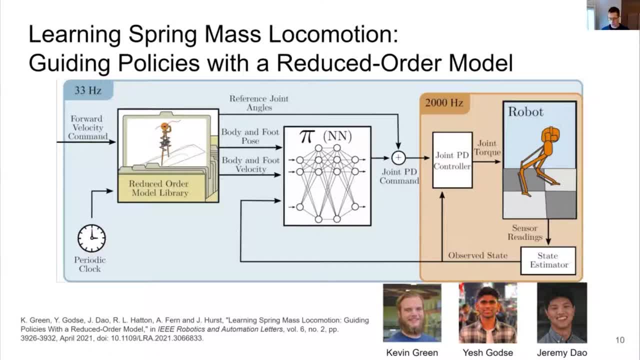 into the neural net to create the policy on the machine. So there may be a bit of discrepancy basically between what the reduced order model is doing and what the robot is actually doing, and that's okay, And so this is kind of the mini-controller. 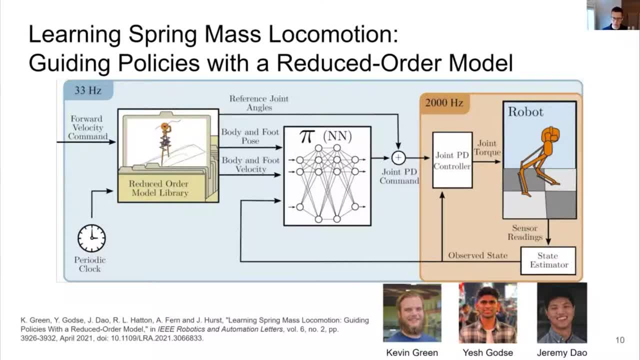 The control hierarchy that we set up, missing a bunch of the pieces, but this is the research. focus was to understand this piece of it. The robot itself and all the really low level stuff happens at two kilohertz And then the decisions about what's the plan, basically. 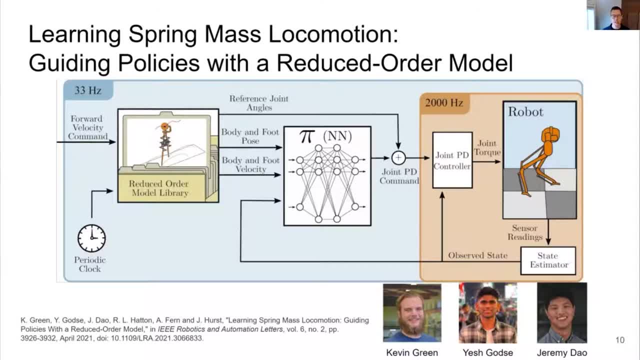 What gate are we doing? What spring mass gate are we doing? Updates at about 33 hertz And you can see that the inputs here are forward velocity command and a periodic periodic Clock input as well, And this worked pretty well. 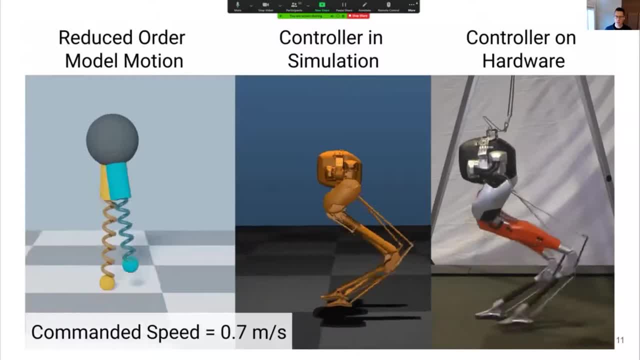 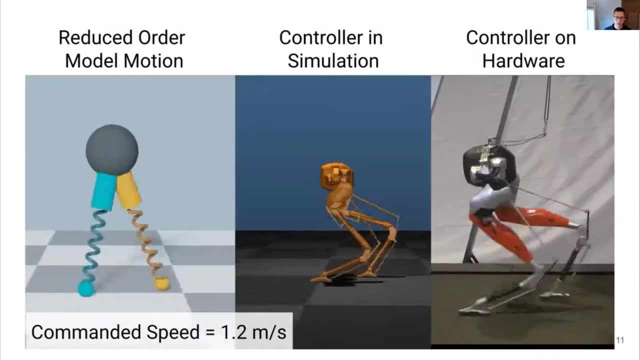 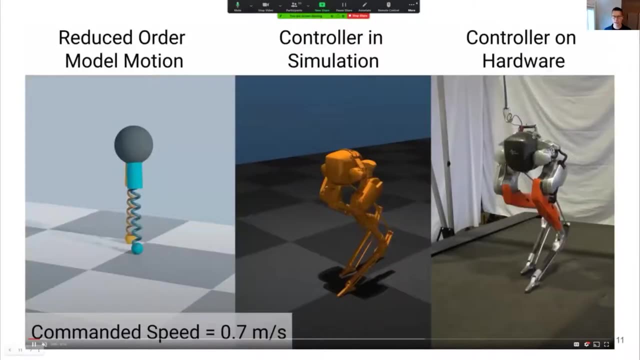 There have been a lot of different attempts at basically making a piece of hardware behave like a spring mass system or some similar reduced order model, And the challenge of course is if your hardware isn't very close dynamically to the actual dynamics of your reduced order model, it's really hard to get it to match. 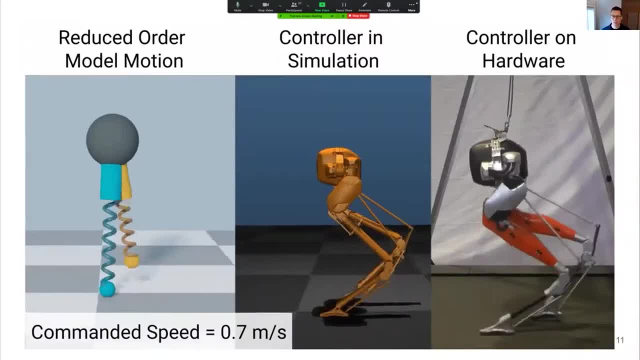 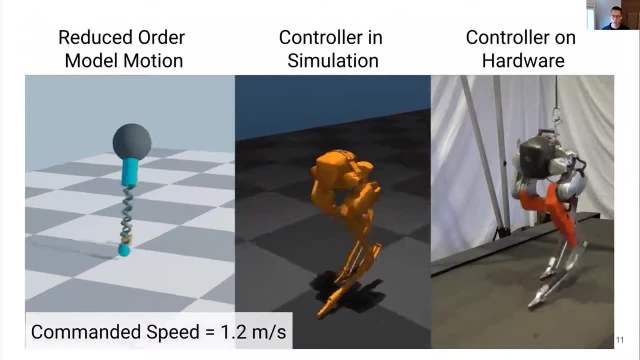 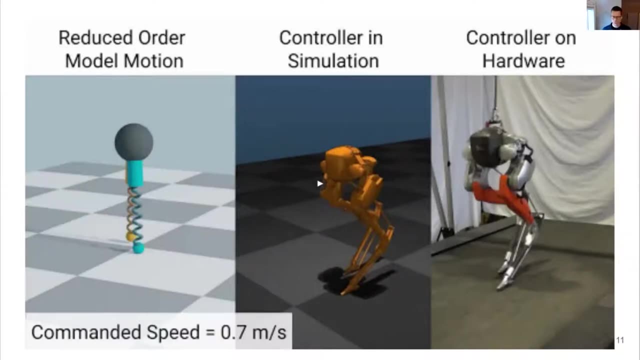 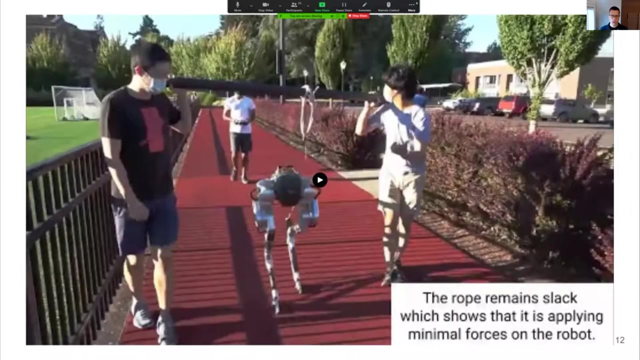 In this case it's pretty close. You know we've worked pretty hard to make this hardware be able to represent this kind of spring mass approximation, But then the learning system was able to really really do a nice job there, And so then we took it outside. 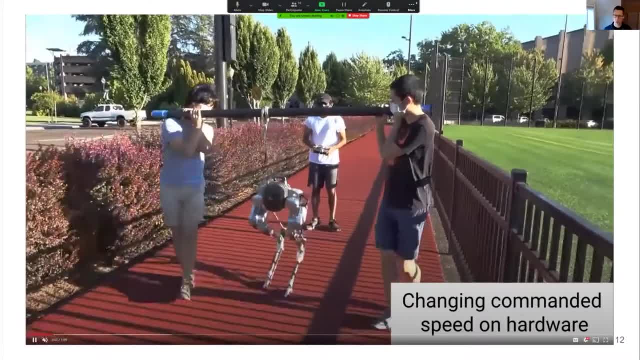 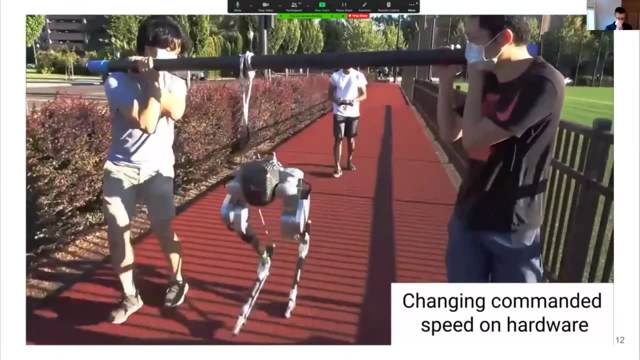 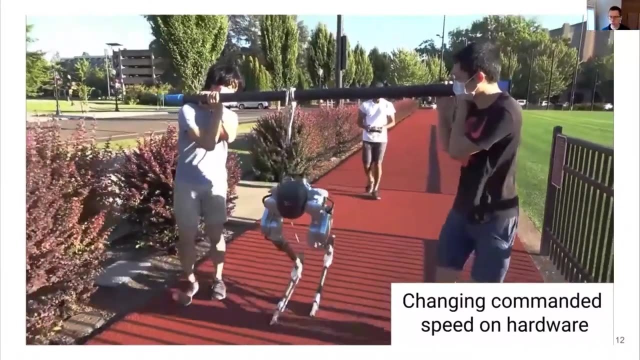 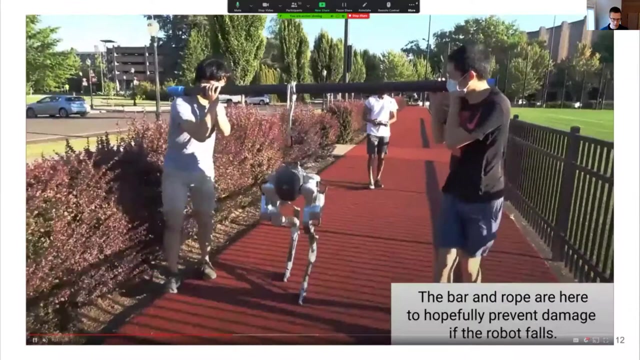 And we can gradually change the speed and reasonably robust to the real-world kind of stuff. And this is just the running track outside in the intramural fields on Oregon State campus And I guess I want to point out that the little rope here to the pole is always slack. 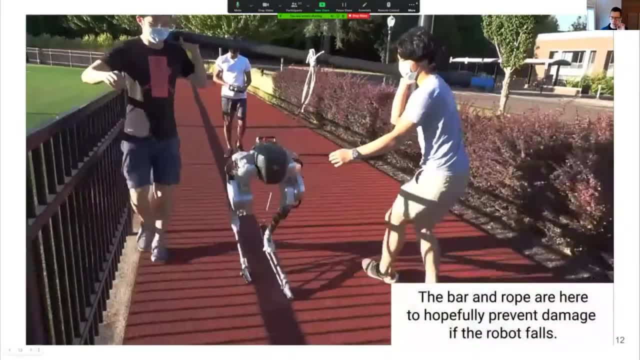 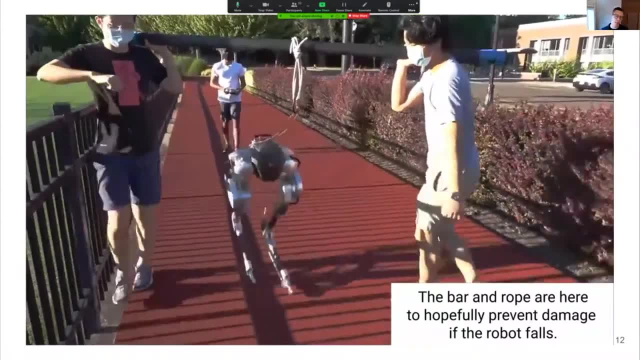 So the robot is not being helped out. It's not being helped or assisted by the students in any of this. In fact, it's usually that they tug on the rope a little bit while they're walking and pull the robot one way or the other. 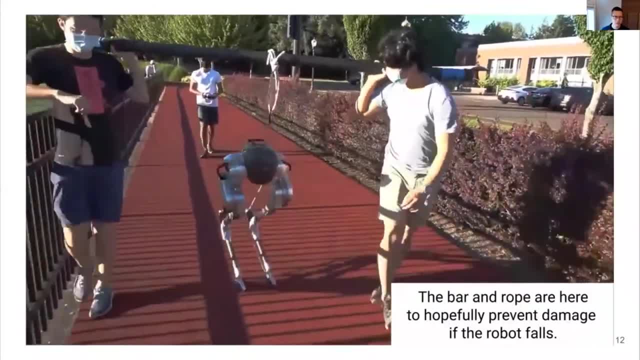 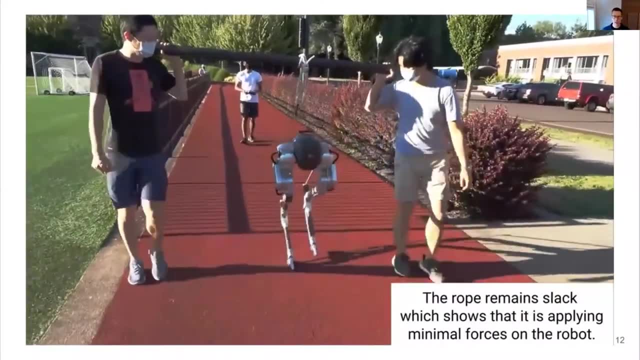 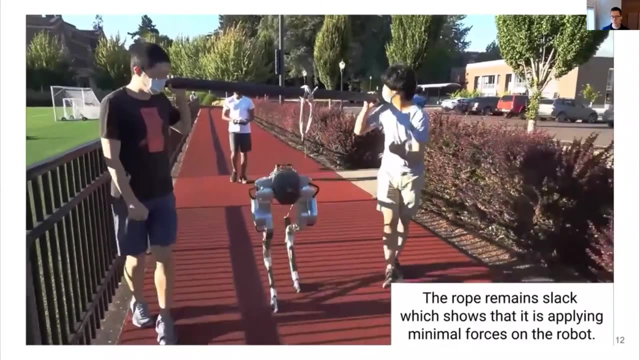 So it causes disturbances more than anything. Now, the whole idea here is: if we can do one gate, then we can have a library of 50 gates. With a spring mass model. we can even have a continuum and then implement a planner on it. 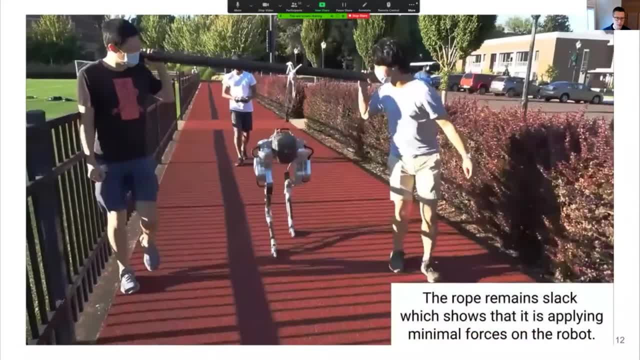 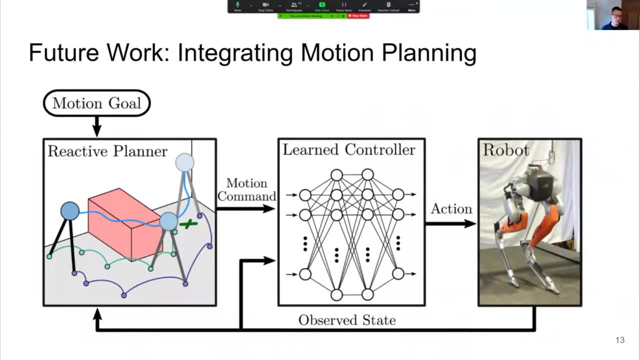 And that's a really promising path forward. And there it is. So some kind of reactive planner where you have a representation of the world in your simulation. You know where the obstacles are. Say, you want to deal with stairs, We can definitely plan using a spring mass model: real dynamic behaviors around an environment. 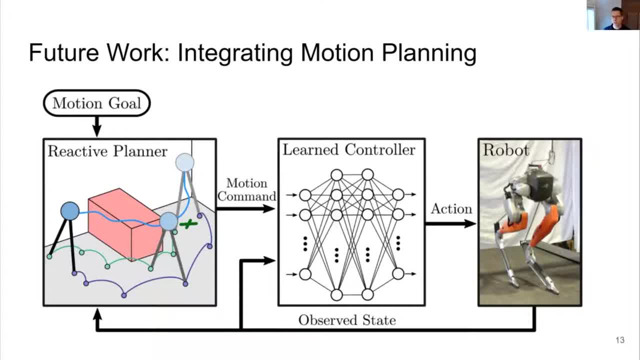 That's much, much easier with a reduced-order system than it is with a full-order robot. Translating basically from that reduced-order model to the robot through a learned controller is an approach that feels very promising. Okay, so another idea here. 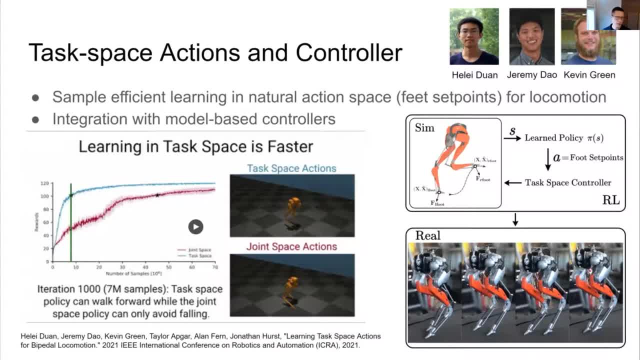 I mentioned that we already have pretty good inverse kinematics and inverse dynamics. Why learn that You want to make the learning problem as small and straightforward and easy as possible and have it only learn the things that you really can't represent any other way? 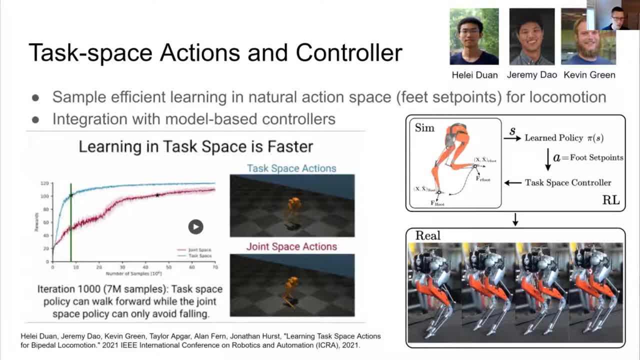 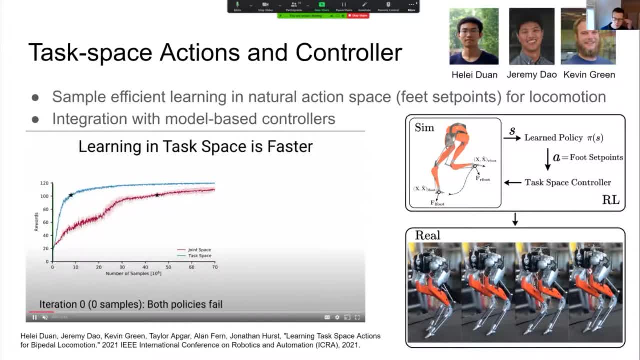 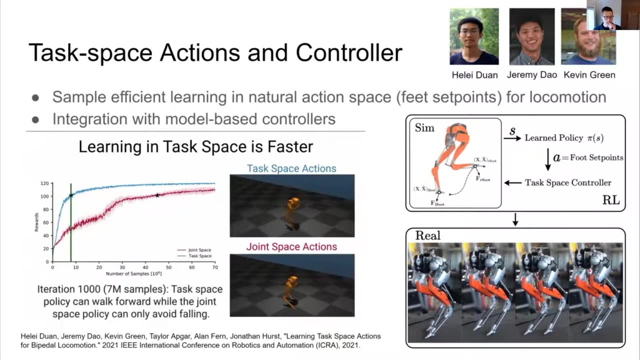 In this case we do know the inverse kinematics, So it is much faster to learn in task space. It also had a better result in the end. So learning is starting to get kind of long, starting to take a few days and things like that. 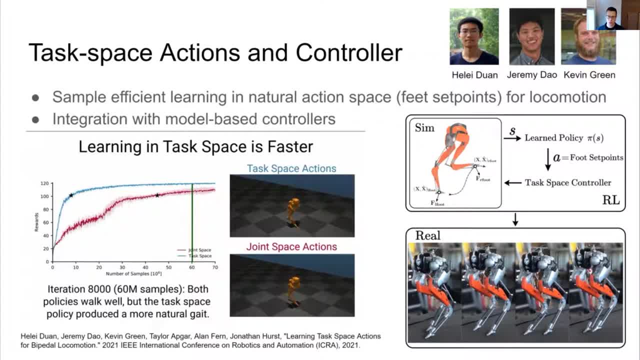 which is tough when you've made a little mistake and you want to see the results of your code Plus as we start to increase the degrees of freedom and we start to you know- this is on CASI- Once we have arms, perception, hands, other things that we're trying to do and we're trying to use. 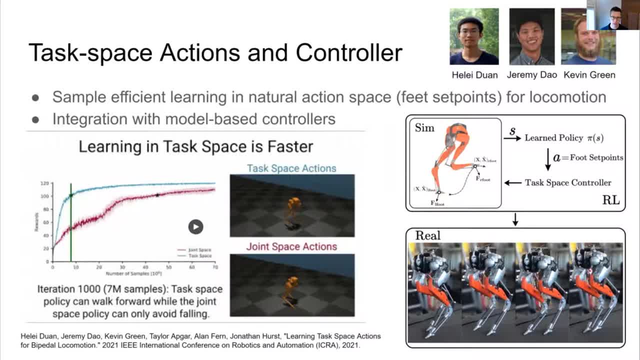 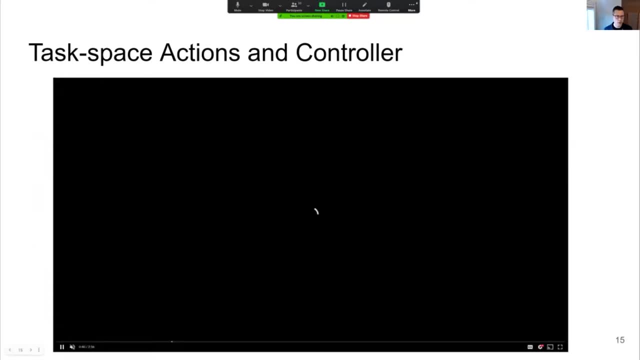 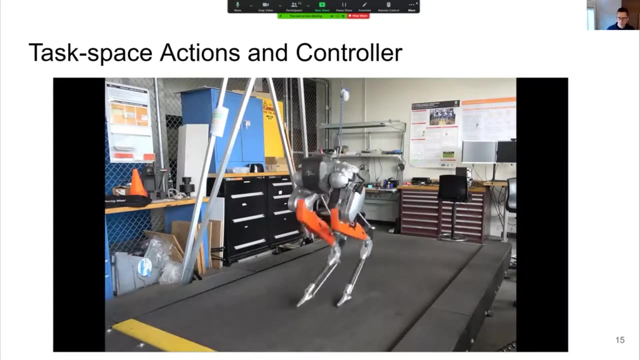 learning with it as well. we're going to want to figure out how to learn just pieces of the problem which this is doing. Okay, So here's some results from learning in task space and then controlling it up at different speeds. Now this has a pretty bouncy gate which I don't know. it doesn't have to. 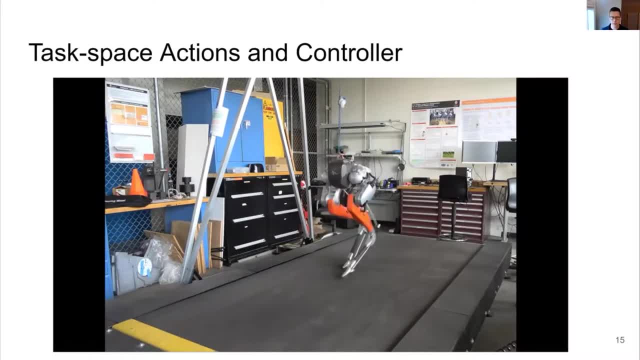 A lot of times, when we have a spring mass behavior as our model, we're going to have a spring mass behavior. It kind of ends up this way. I don't know, maybe a little bit more than it should, But it does work. 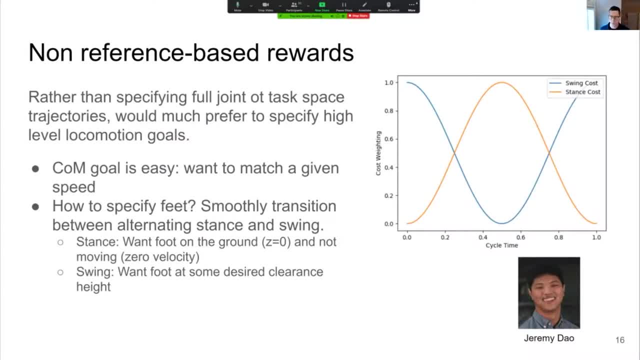 Okay, Now this idea is saying: okay, I'm not sure about having a clock, I'm not sure about having trajectories that I want to give it. I you know, it's just a matter of time, Okay, So philosophically it's really challenging. 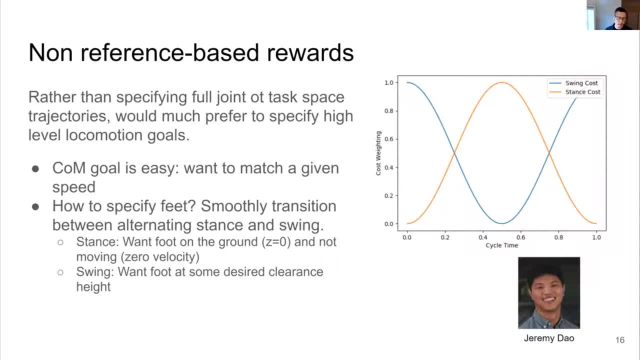 I don't like the idea of feeding trajectories to the machine because, ultimately, if all you're doing is controlling a robot arm in space, then a trajectory makes sense. But we're trying to control, we're trying to create a set of dynamics. 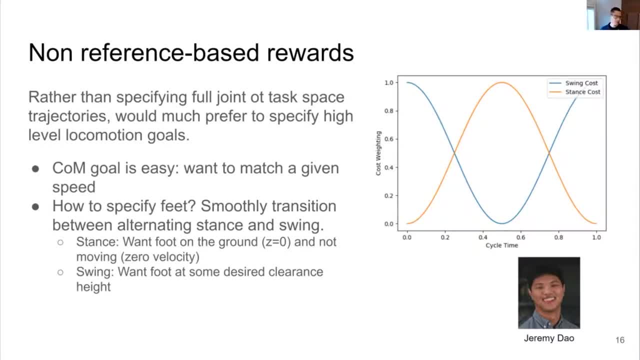 We're trying to describe ahead of time basically how the robot is going to behave when it encounters unexpectedly the ground surface, Because you don't necessarily know when your foot is going to strike the ground. But you want your whole control system and the machine. 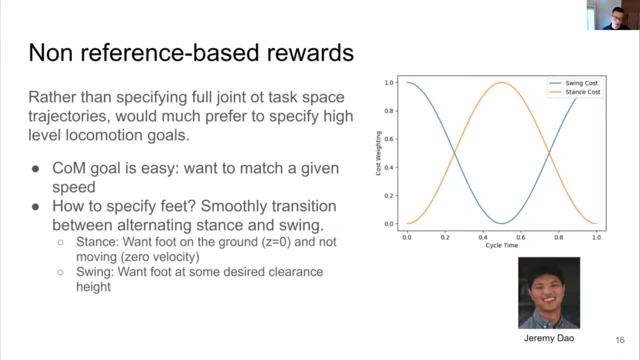 to respond appropriately when it does strike the ground. So giving it a trajectory as an input kind of implies a very specific ground contact point in time, which is not good for robustness because it's going to vary a lot when the system is actually existing in the real world. 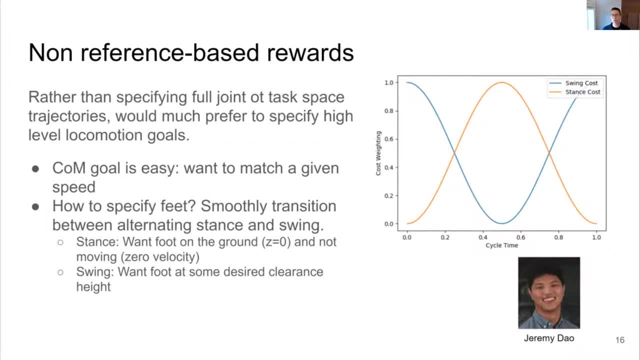 Another way to think about it is that position trajectories are one symptom of many, including forces and accelerations and so on, that your machine is going to experience while it is interacting with the world, And so the end goal is really not the trajectory. 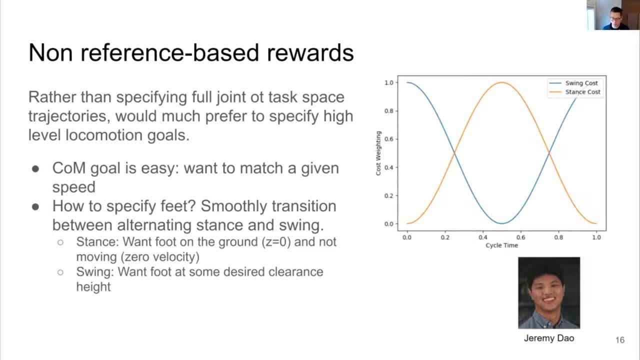 That's not what we're trying to achieve. What we're trying to achieve is the dynamical phenomenon of legged locomotion, And you know if you're looking at a video of a particular period of time in which something is walking or running. 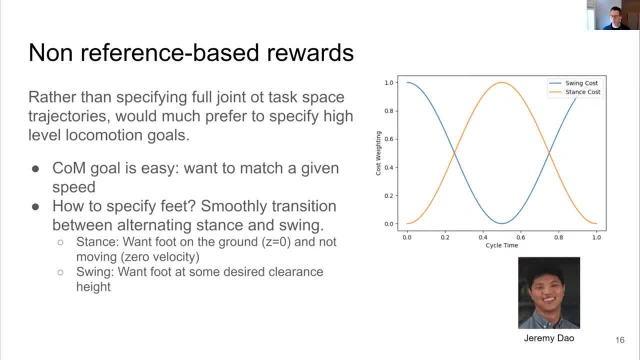 then you can say, yes, there's a trajectory that it followed as a result of its dynamics and its interactions with the world, But it doesn't mean that you want to replicate that trajectory, Because a different time and a different terrain and a different speed is going to give you a 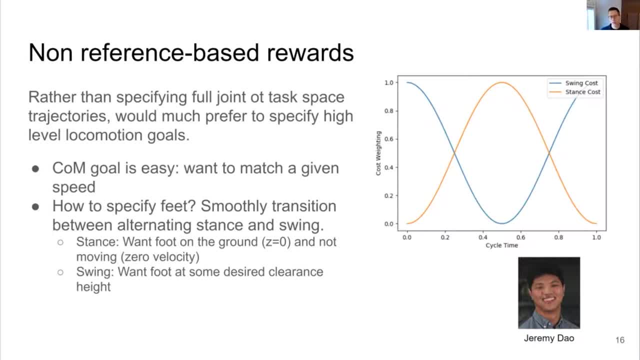 different resulting trajectory. So we want to eliminate trajectories from our input for controlling the system And instead really be careful to think about. what are the high-level locomotion goals, Things like we know that the forces are going to go from zero up to high and down. 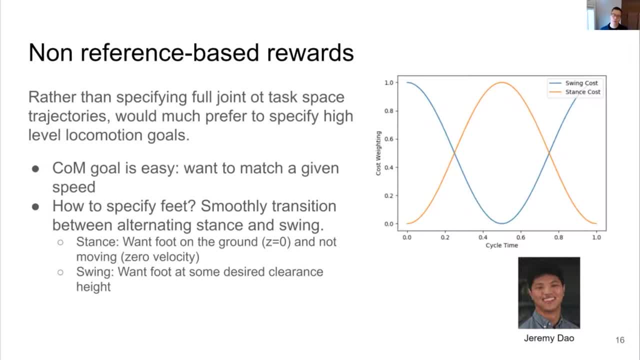 We know that we care a lot about peak forces. We don't want to have force spikes. You know we care about a forward velocity, We care about a certain ordering of when the feet are on the ground and which one is on the ground when. 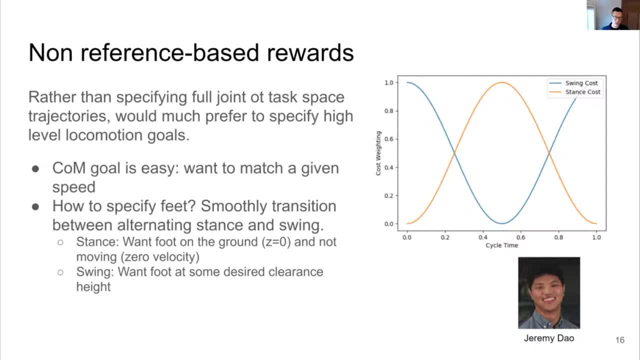 And so trying to write down the list and define what is legged locomotion has been kind of the big challenge behind everything we're doing. I kind of started out saying, well, it's based on the spring mass model, But it's not. 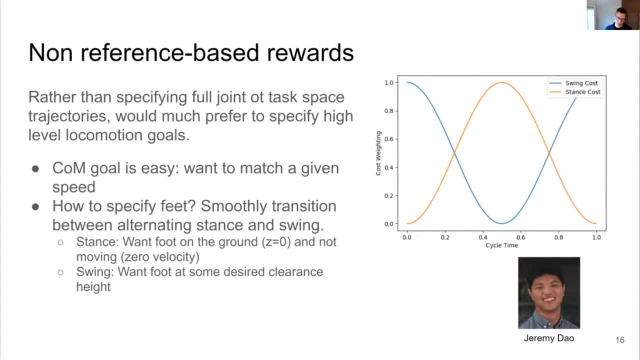 It's just that the spring mass model is also exhibits most of the features that we want from legged locomotion, And this may be 75% correct, But there's a lot about it. that's why would we use a linear spring in a leg, for example? 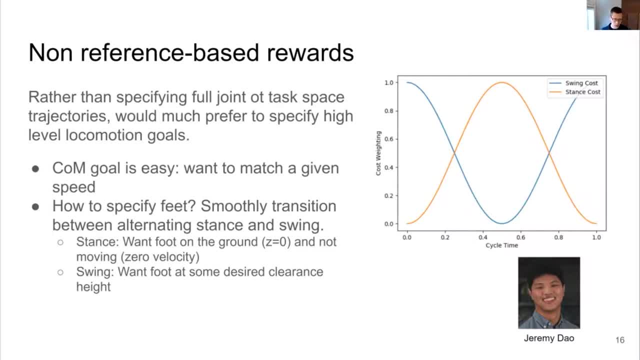 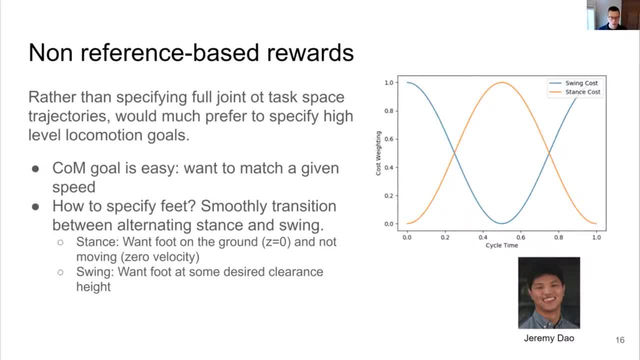 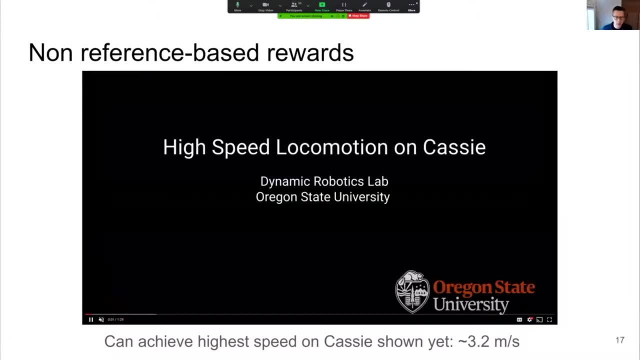 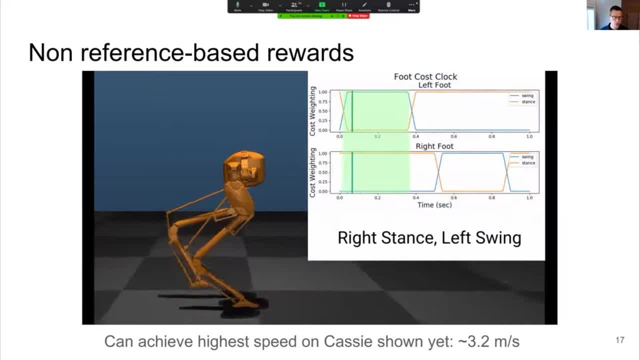 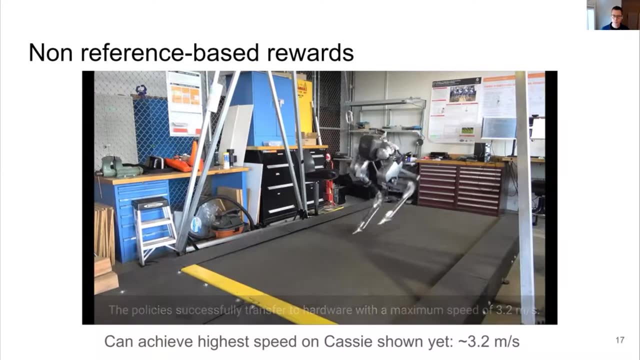 I think this is also the fastest biped robot So far That I'm aware of. But if anybody knows of a different one or a faster one, I hope you'll let me know today. So let's see, We're dialing up the speed a little bit. 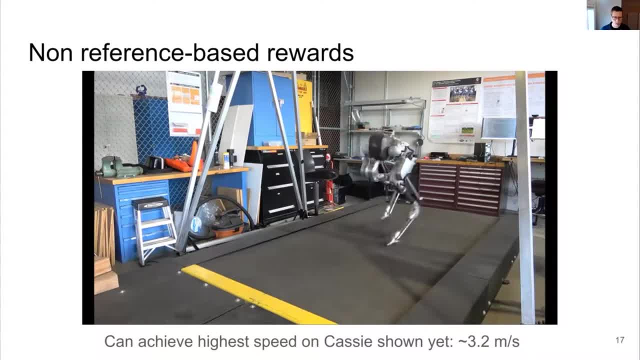 And you know the research system. they've got to dial up the speed on the treadmill and keep that aligned with the speed of the robot as well. It fell off the back of the treadmill or ran to the front of it quite a few times in doing this. 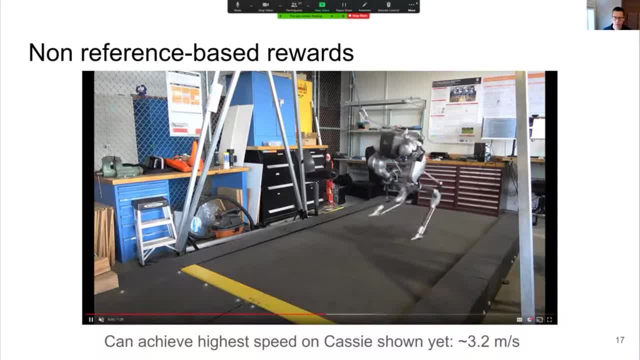 testing. Okay, So we're going to try and get a look at this. So we're going to try to get a look at this. Is that a? How does the video look at your end? Is it? Is it reasonably smooth or is it a little bit choppy? 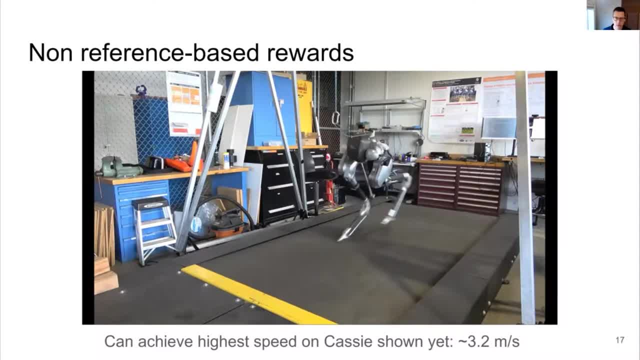 I can try and share YouTube abyss. Okay, It's good. The thing I like about this is once it starts to settle into a gait like right here: kind of looks plausible, like something that an animal might look like. It's getting close to something that feels good, feels reasonably natural. 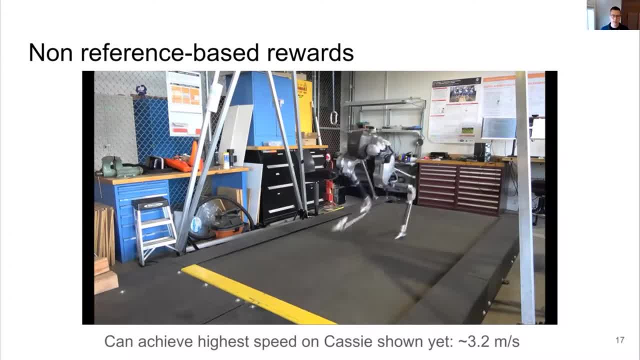 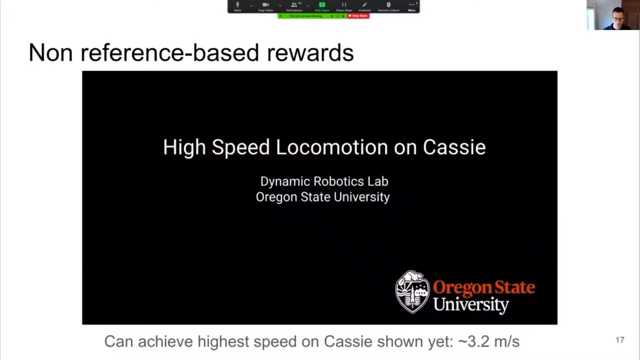 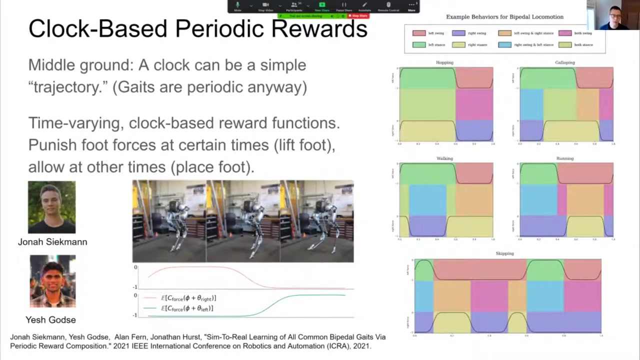 Yeah, So that's pretty exciting to me. The question is, how robust is it? It does fall All right. Now the next thing that we aimed to do was kind of choose this middle ground where we're giving it a trajectory, but it's not really a trajectory. 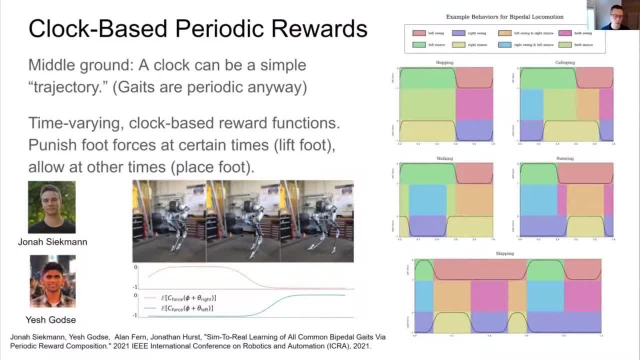 We're just telling it which We're telling it: the duty factor of when- When the foot should be on the ground and when it shouldn't, And we're not requiring it to have the foot on the ground or forcing it to put the foot. 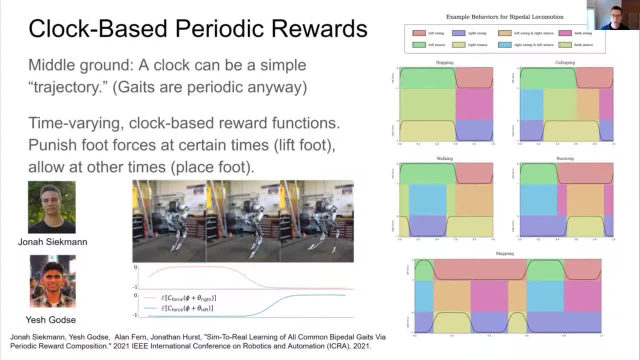 on the ground. It's just changing the reward function. It's saying that for this segment of the gait, you get your rewards for having your foot in the air, And for this segment of the gait, you have higher rewards if your foot is applying forces. 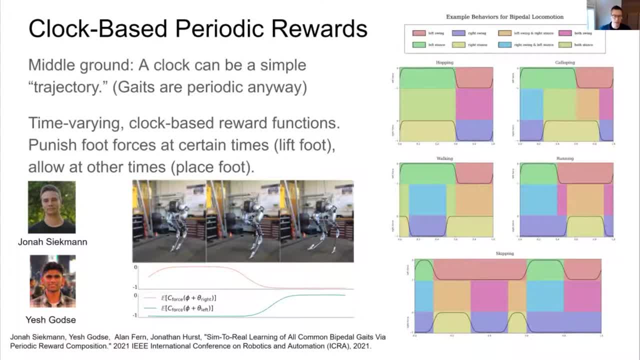 on the ground And that allows the system to kind of finesse it and to make some choices. And you can see too that it's not a discrete change, It's a gradual transition from you prefer to be in the air to preferring to be on the ground. 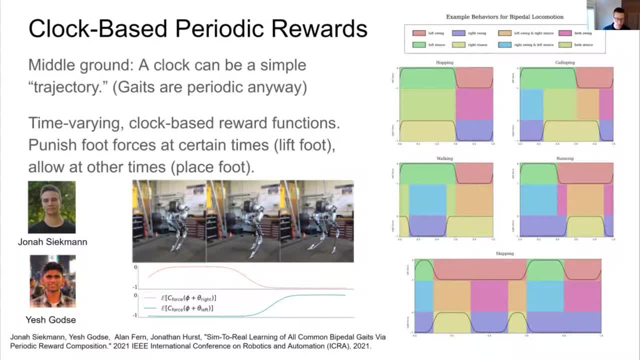 So that really enables the system, especially if you do a little bit of dynamics, randomization in your learning, in your training process, to be robust to uncertainties about when the foot actually arrives on the ground And that also allows us to change the ordering pretty quickly of which foot is on the ground. 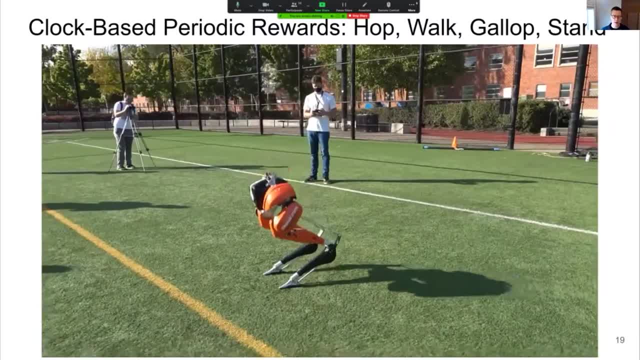 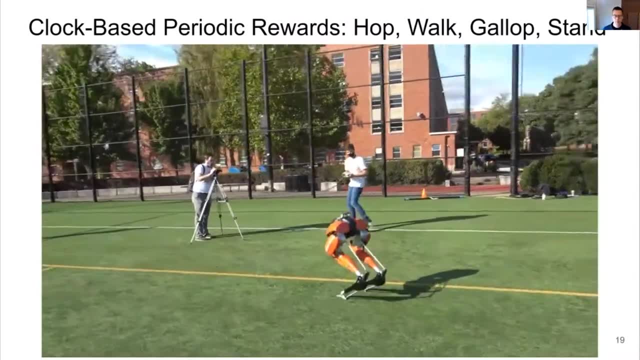 And so here we are, rewarding it for having both feet on the ground at the same time and both feet in the air at the same time, And we're able to come up with a nice hopping gait And then we can transition it. You press the button and say, OK, actually I want now the walking gait. 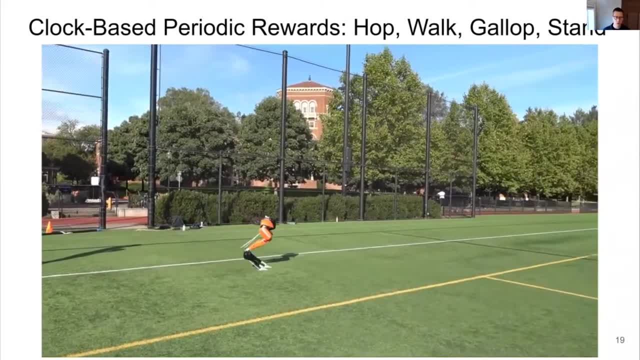 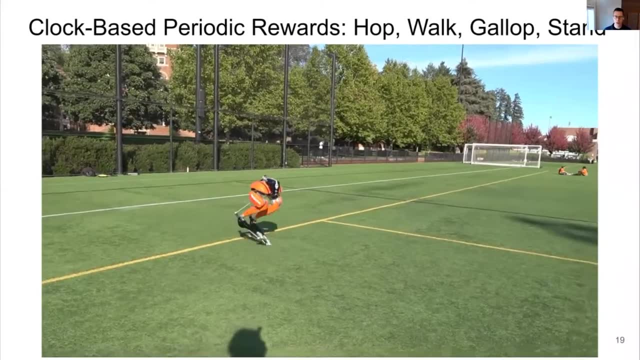 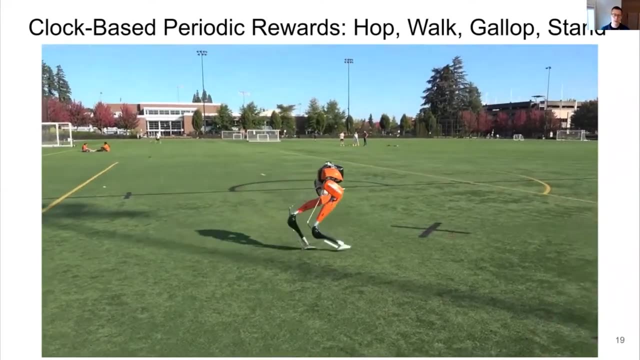 And it transitions to a different ordered walking gait or a hopping gait And back to a stand as well, And you can see this, This. It's hard to predict which of these ideas is going to work really well. This one worked really well. 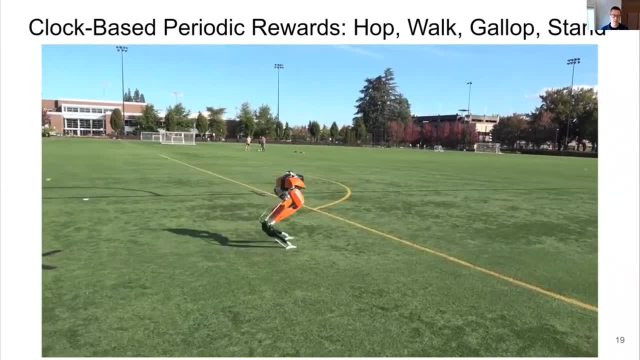 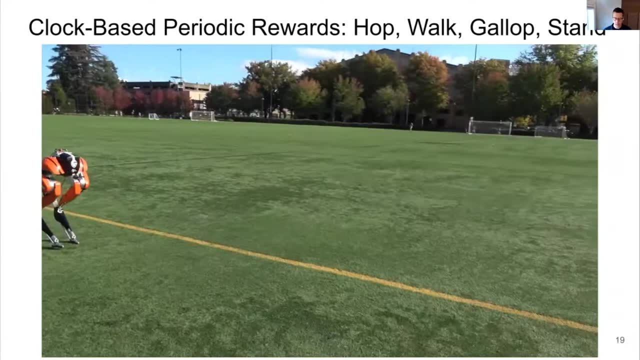 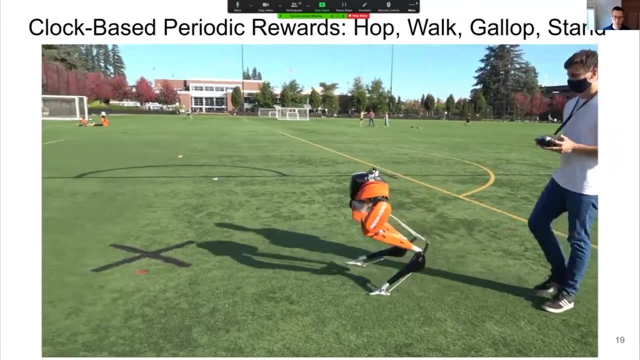 It was like enough guidance for the system and enough dynamics, randomization in what we did to be pretty robust in the world. Now we used a variant of this controller just a couple of weeks ago actually to run a 5K, a full 5K foot race on campus. 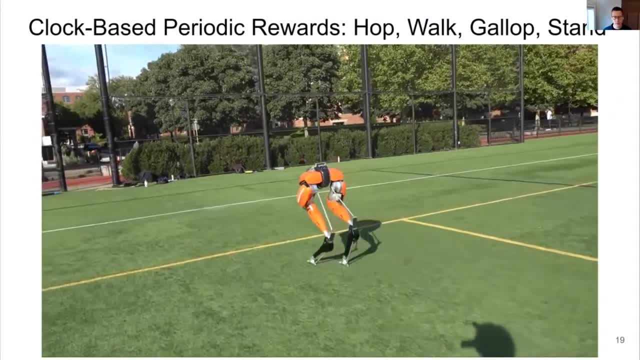 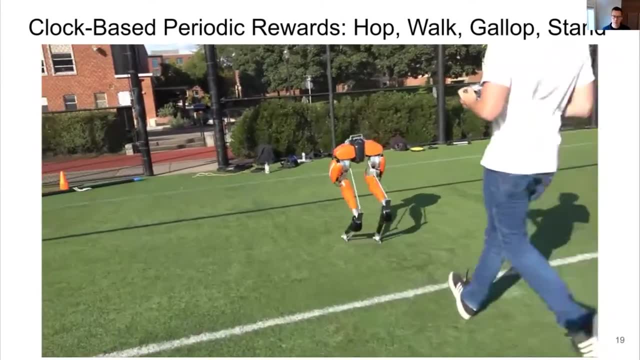 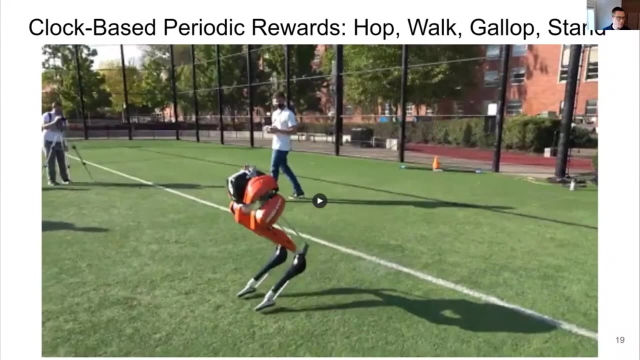 We filmed it. We haven't yet edited that together, But one battery charge all the way across campus and over some curbs and things like that and back, and about a 45 minute rate. So a light jogging speed for a human. Oh, we got a good skipping gait too. 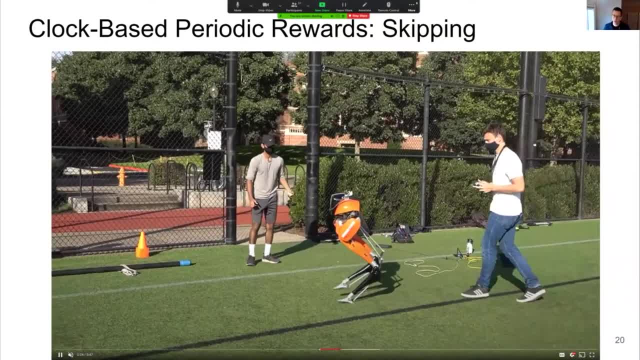 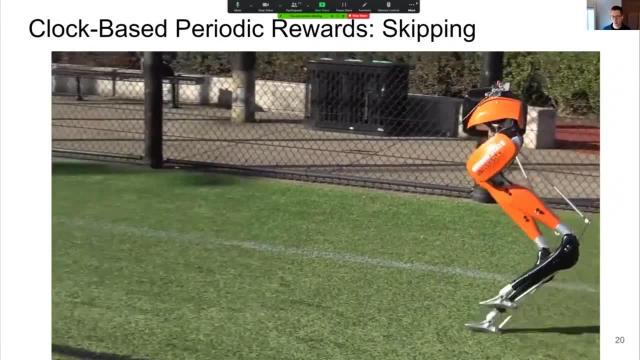 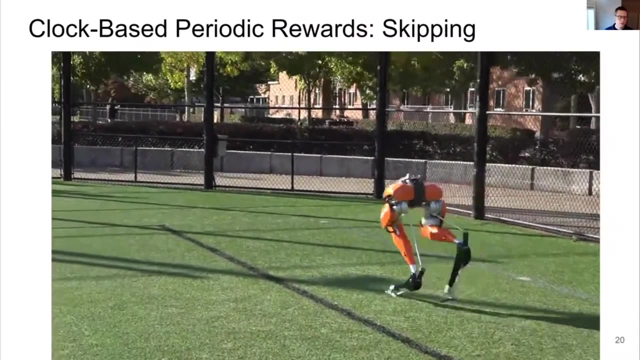 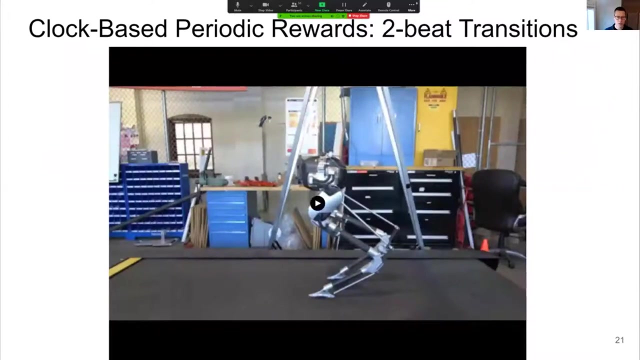 Let's see. if we show that here Now, why would we want a robot to skip? I know No good reason. I guess it looks kind of happy. But it is a nice illustration of what you can learn on a robot. So this is just a close up of showing the transitions between the duty factors. 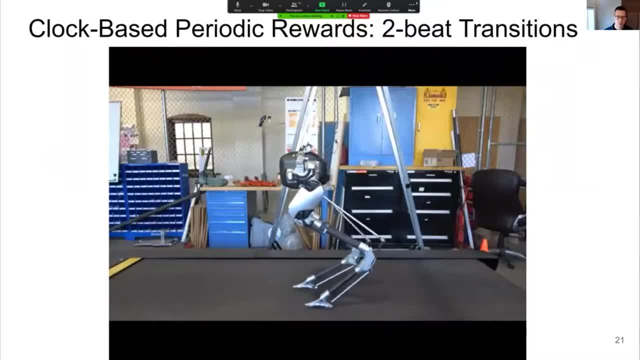 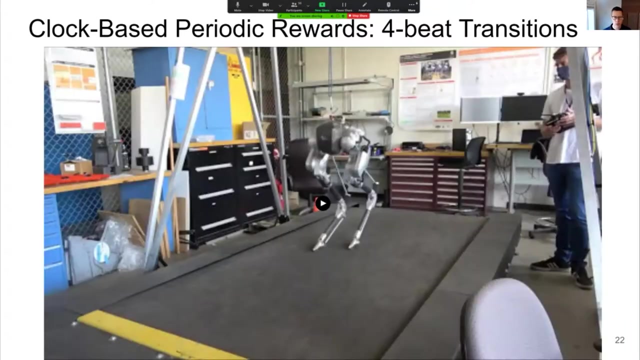 Hop to walk and transition again here, I think. So it is off to the right here, OK, And because it's part of the learning process to do the transitions, it's learned how to do them pretty robustly Now if you kind of increase the freedom of the transitions. 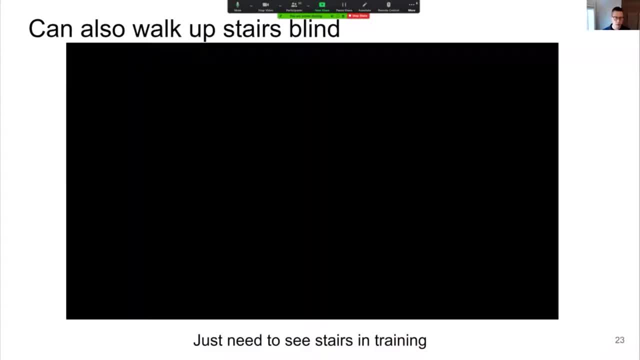 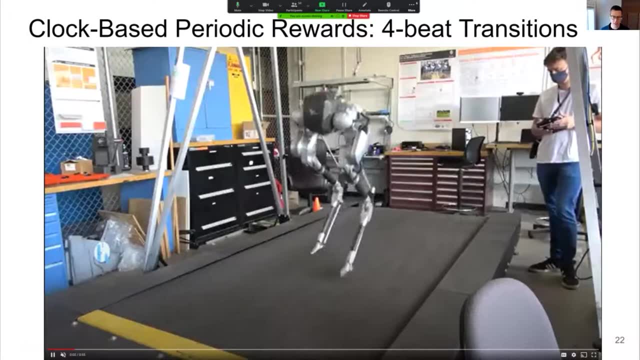 I don't know. It's like changing the discretization of it. Whoops, you can add in skips and gallops and things like that. It doesn't have to just be hop and walk. Now you can do the run, walk, skip all of the other things. 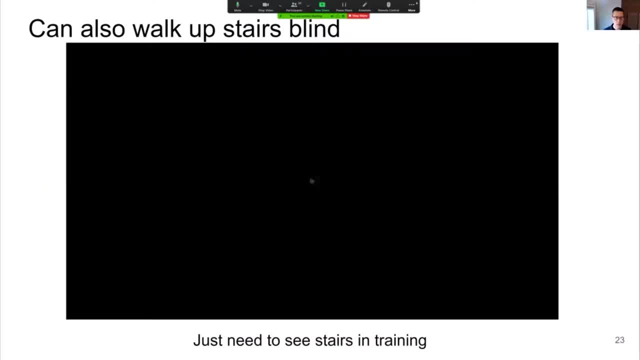 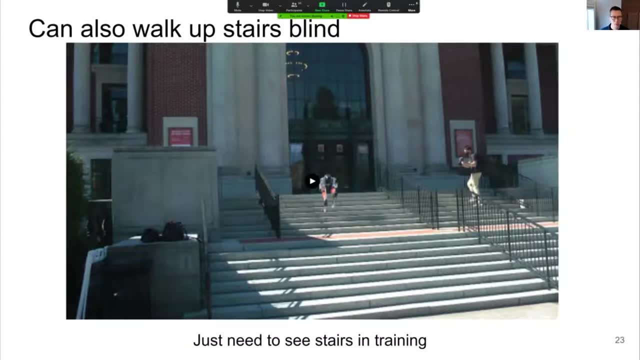 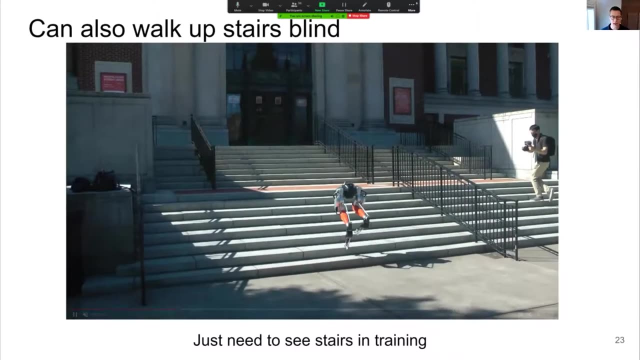 Okay, And then um, finally we. we found that if you train it with stairs, it works. This was, um. we weren't sure how good this would would get, but kind of surprised us. Now it does have a very high stepping gate, because it needs to if it can't see the stairs. 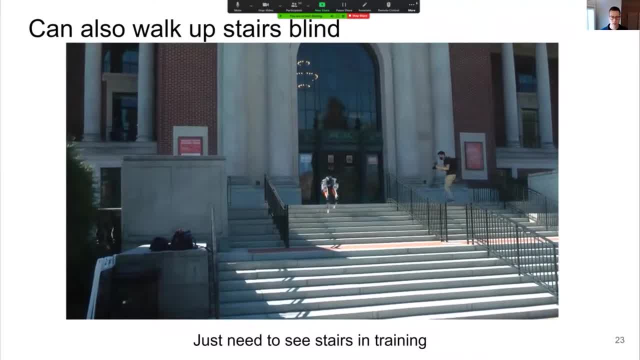 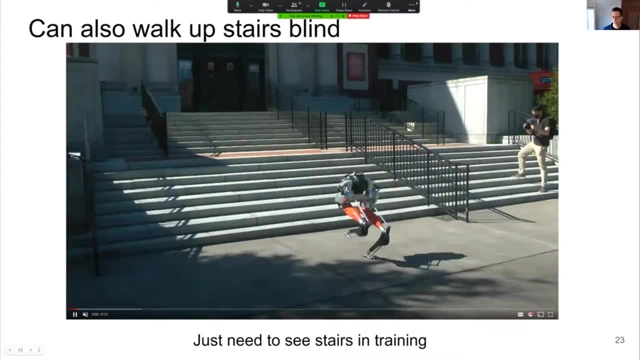 but, uh, you know, up the stairs it goes And in this case you can see one um metric of stability. I remember Chris Uh has coined this, that, uh, the question is, how far away from the robot are the researchers? 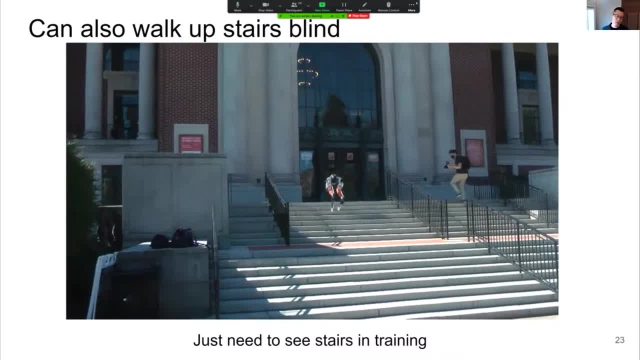 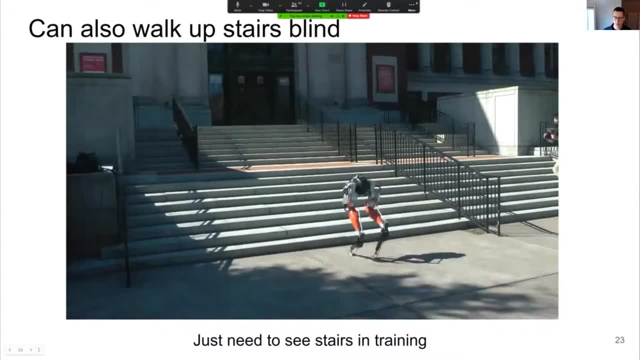 willing to get, And in this case you can see it's got a pretty good stability factor. There's no tether on it and there are no graduate students near it. Um, so we were pretty confident that it would be able to successfully go up these stairs. 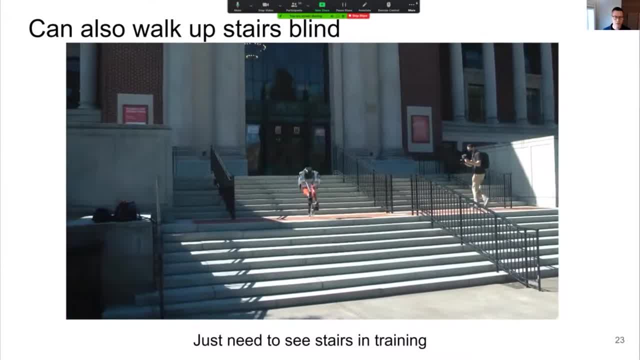 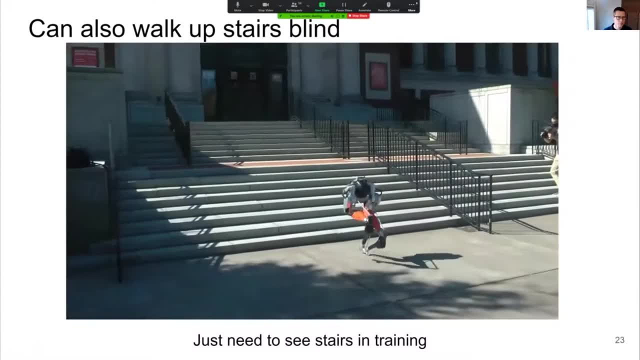 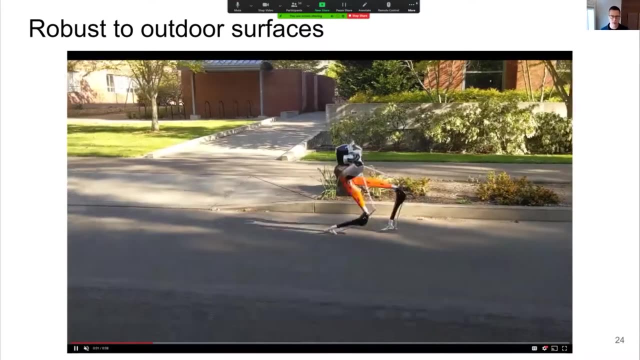 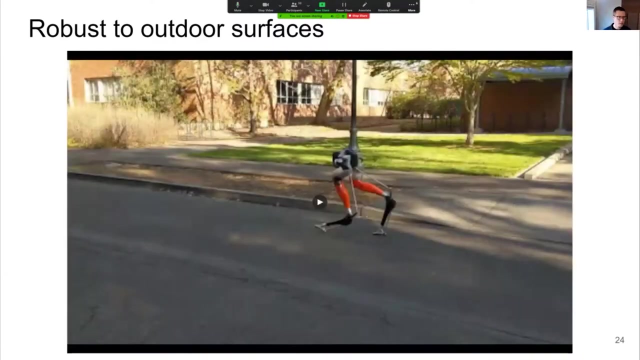 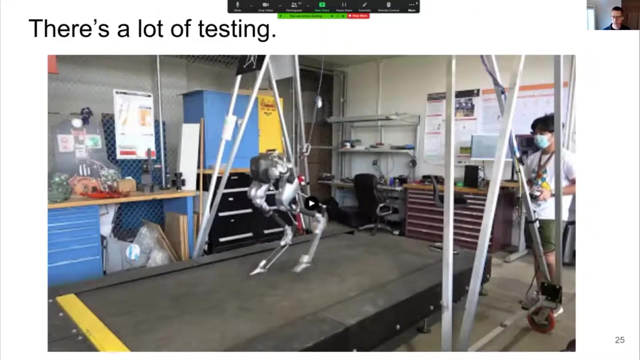 without falling too hard. This is just, uh, a brief clip from running around, uh, part of the 5k. um, it was fine And I think we've got some curbs here we show. okay, here's some bloopers, ton of testing. 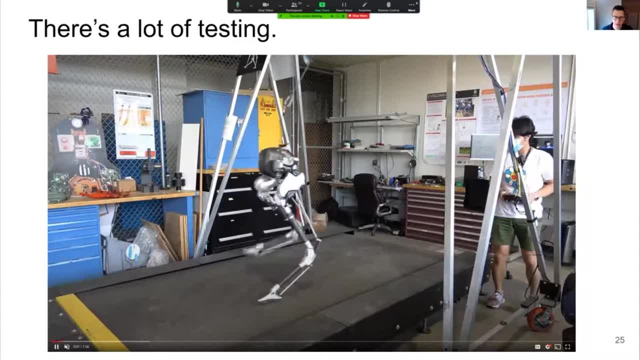 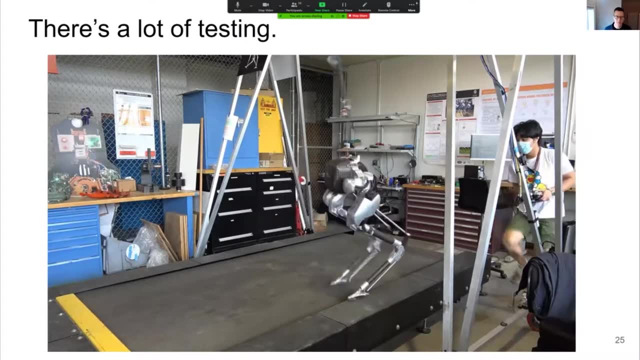 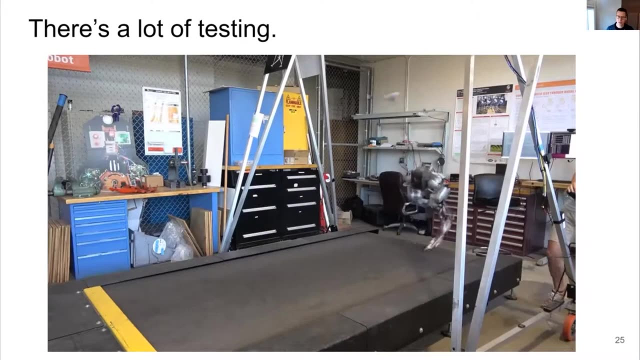 right. Certainly it goes through a lot of learning and simulation falls constantly. but even you know, of course, trying on the robot it does too. Okay, It's been kind of a long year hard to do. all the testing during the pandemic lost to. 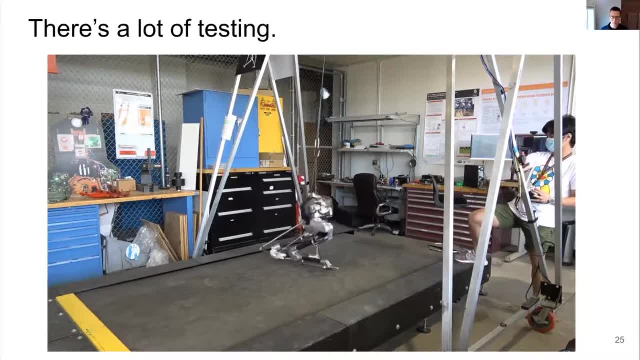 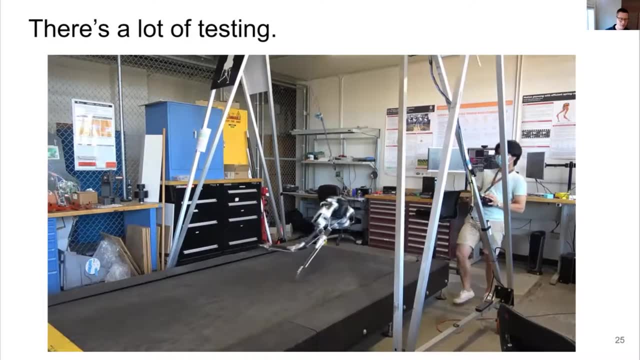 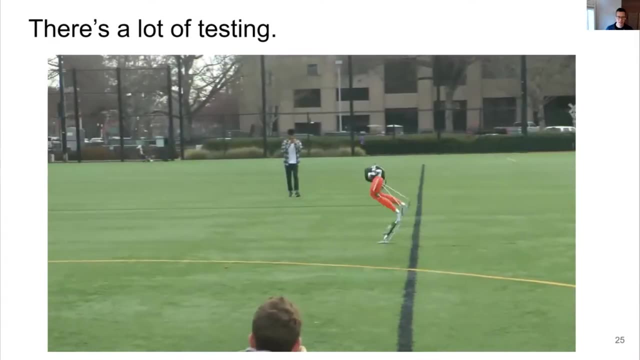 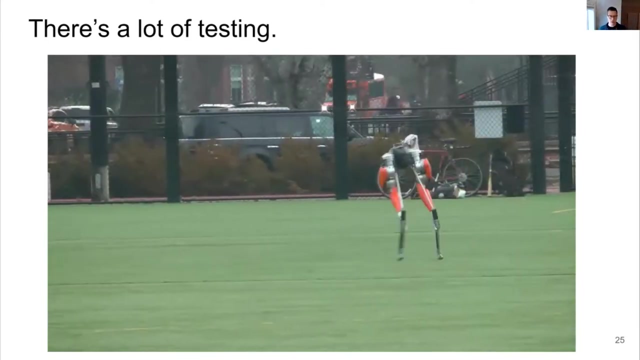 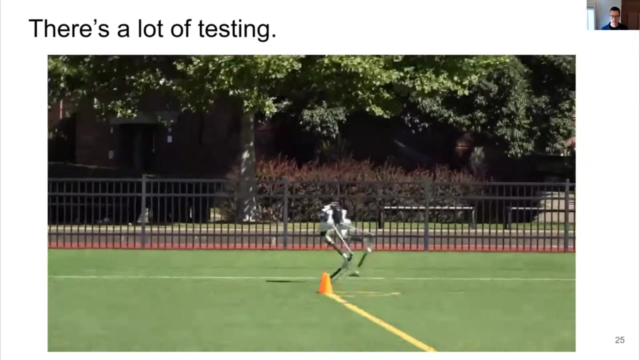 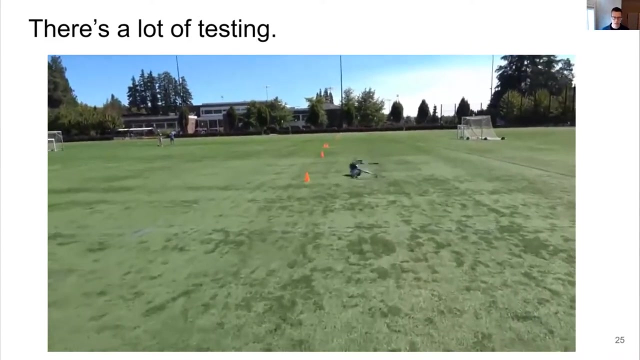 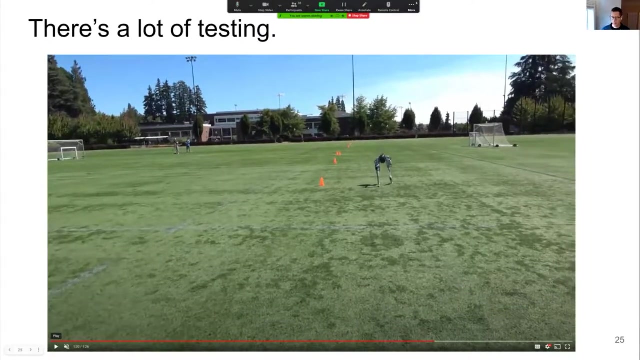 Conrad, there there's a uh treadmill control error. Okay, Kind of got it in a weird stutter step behavior. So this, what happened in that particular example is is actually the uh, the data logging was creating a file that was. 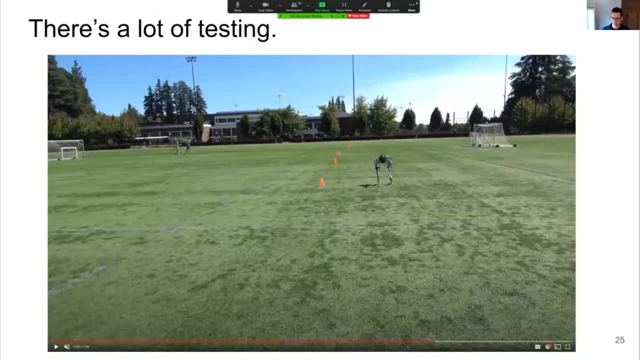 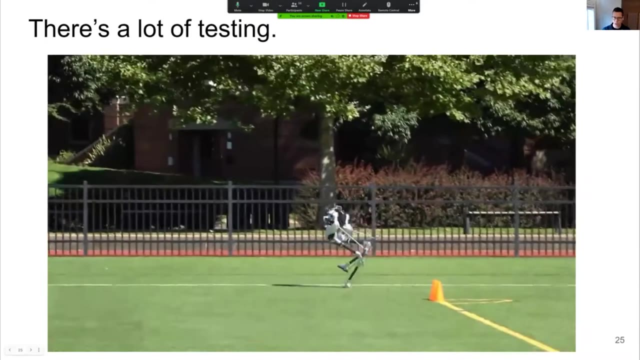 that was too big and when it was writing the data log to the drive it kind of paused all of the control outputs for some number of milliseconds. so all of the motors just kind of paused for a little bit and you can see that the the leg just pauses right there and doesn't put its foot down. 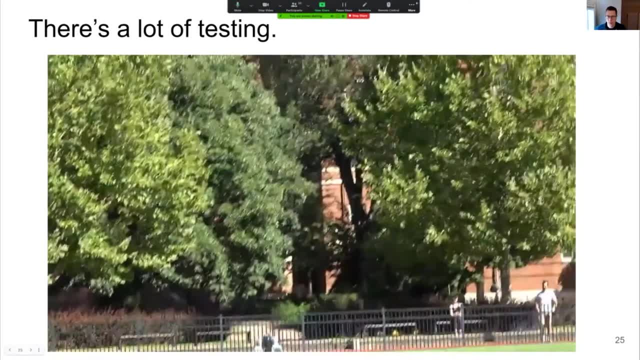 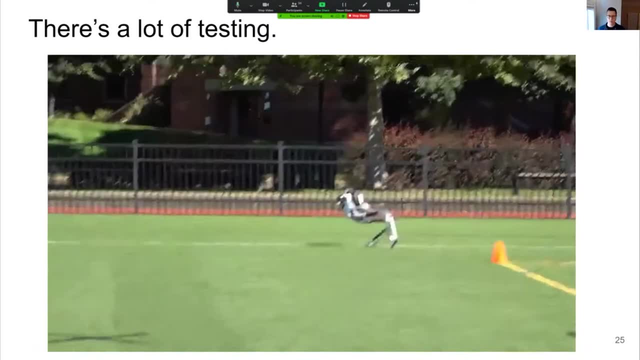 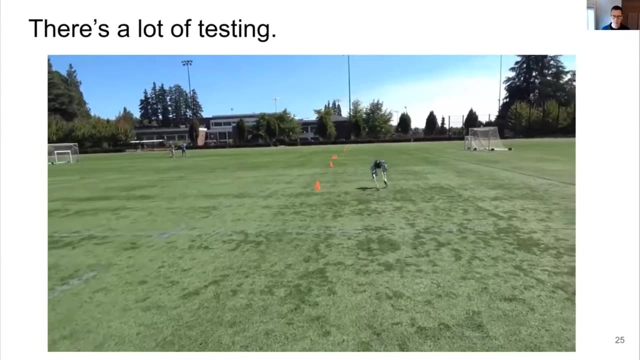 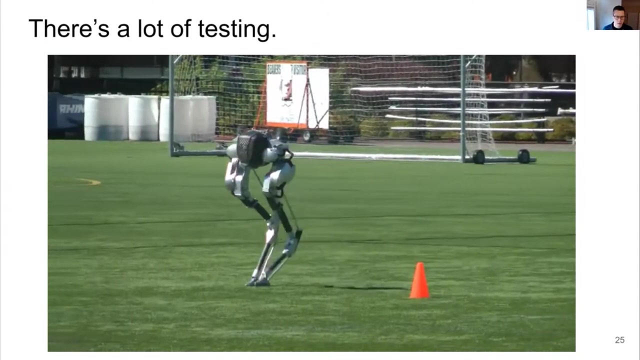 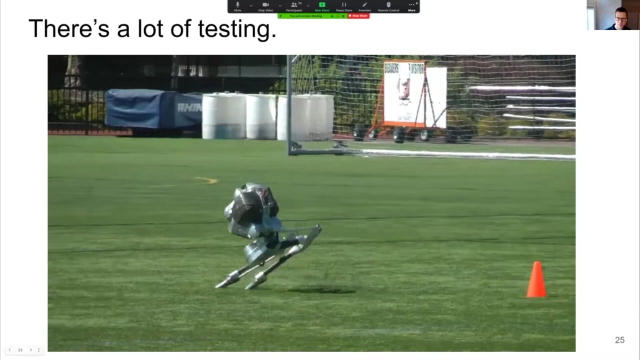 so it was a kind of a hardware hardware malfunction. took a while to debug it. you'll see it right here. pause, and just then you know, wasn't commanding anything for the rest of for the gate. the real-time system wasn't real-time. there it goes. kick up some dirt on the way. 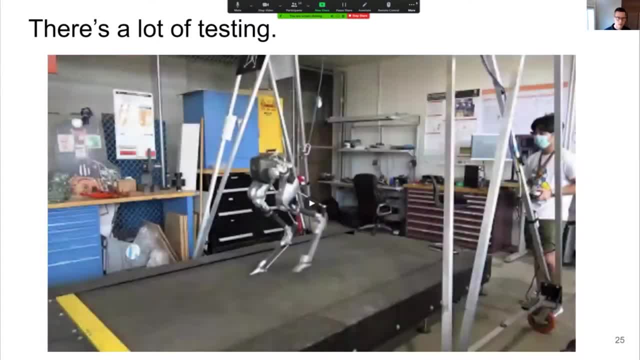 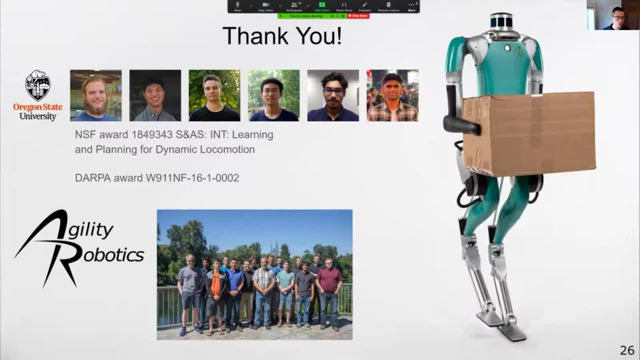 all right. well, that concludes my talk. thank you for listening and i i hope i get a whole bunch of questions. great, thanks a lot, jonathan. again, our audience can ask their question directly or put their question in the chat session, so we can ask them. okay, who goes first? 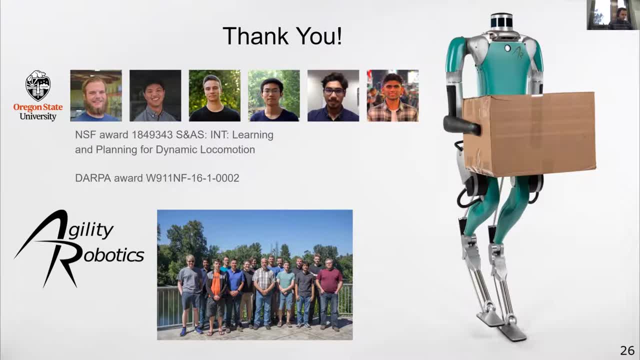 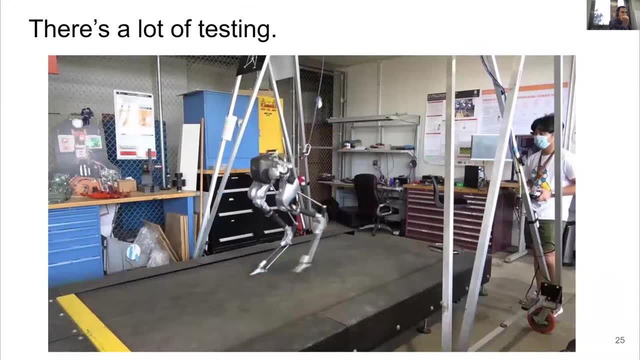 for the first question. i kind of start with the first question here. so in the, in one of your first video, they were showing the cassie on a treadmill and you showed that uh, the, the reduced model, cannot uh come up with the behavior that it it needs to compensate. 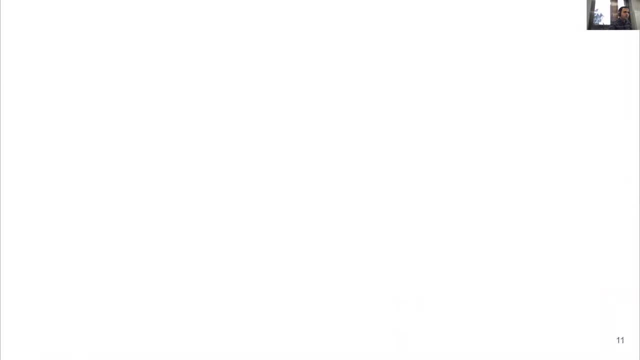 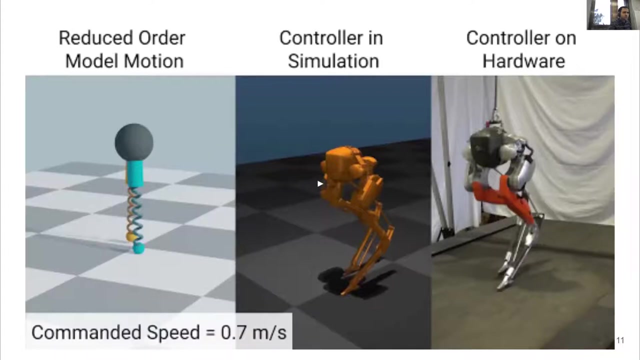 for, uh, for momentum. right, uh, momentum, the compensation for angular momentum. there the lower puts his legs a bit outside, and you say that you use a learning base to compensate or to learn that behavior. so i wonder, if you use a more detailed model like centroidal model, could you use a model-based controller that uses the central model and 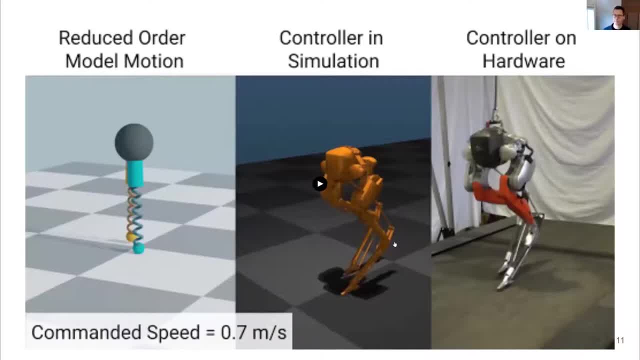 come up with a plan which is reasonable, absolutely. um, you know, we were trying with models as simple as a clock input. that's a model. basically we're still giving information about which foot should be on the ground and when. that's a model. basically we're still giving it information about. 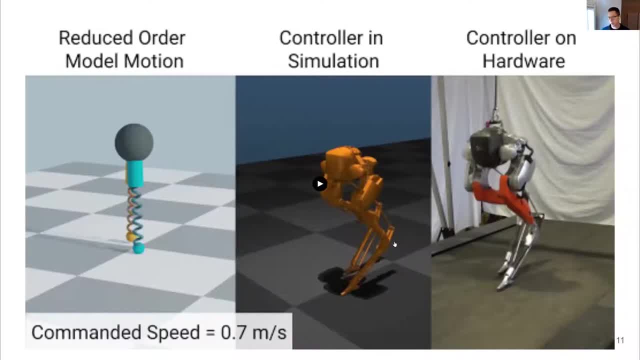 which foot should be on the ground and when that's a model, um, the spring mass model or linear inverted pendulum are reduced. order of varying levels of reduced to give slightly richer inputs to the learning system. i think that having, yeah, the centroidal model and and so on, for whole. 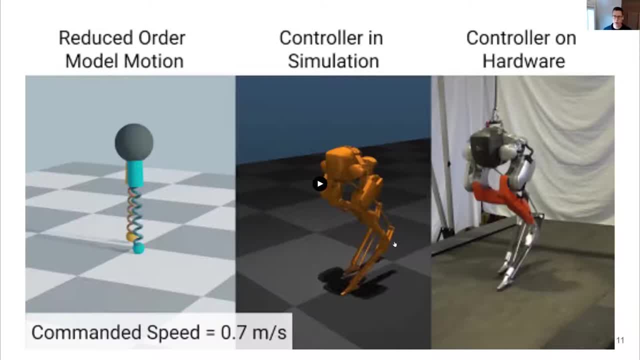 body control is it's? i mean, it's very important. i think that's a very good way to go. and then the question is: can you use learning- you know it's still a reduced order model, right, even the centroidal inertial model and so on- which is going to give you better information about how you should swing? 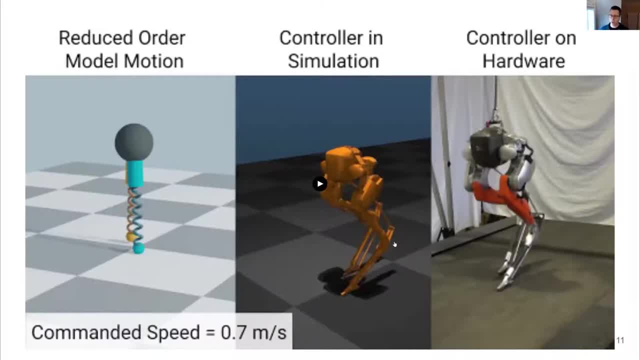 your arms or how you should rotate your legs and things like that. how do you do the whole body behaviors with many, many degrees of freedom and- and that's important because the learning system is going to perform very poorly- with like a 40 degree of freedom- humanoid robot, it's, it's. 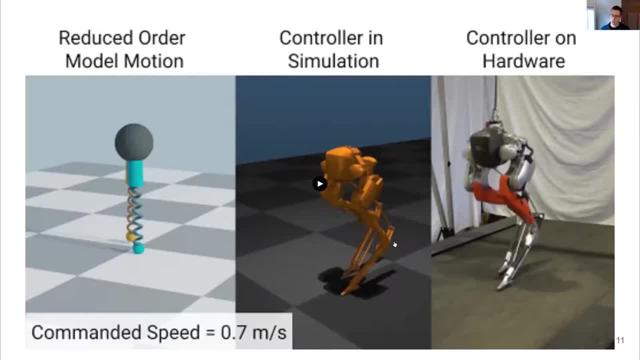 going to be too many variables. um, so if you can instead learn just a piece of it, like the relationship between the inputs to the, you know, outputs from your, your centroidal model, to the, the legs, for example, and then that's just something that's part of the black box that you 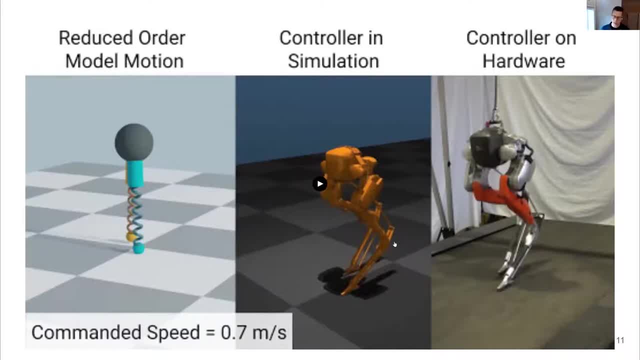 learn, um, but yeah, i think you sprinkle in the the learning throughout a much, much more complex engineered system and decide what your reduced order model is and how you're going to run an optimizer to to send commands to your, your whole machine. okay, i can go for the second arbor until you get ready the question. so my question is a bit more. 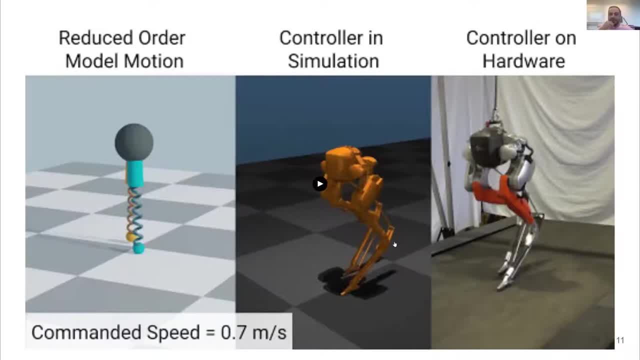 high level. um, you think, when, when you, when we don't have any vision system, you think we need any kind of planning or we can just rely on reactiveness of a learning algorithm based on, i mean, if you don't, if you don't have any information about your environment that you really 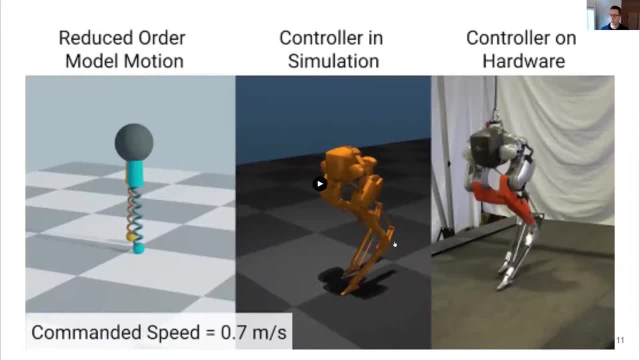 can't do much in terms of planning. so i mean, you know what i'm saying is that do we need to combine a, for instance, reduce order model such that we plan and then we combine with the learning model, such that we can have some kind of best of both worlds, or something like that? yeah, i mean here here's an example, right, 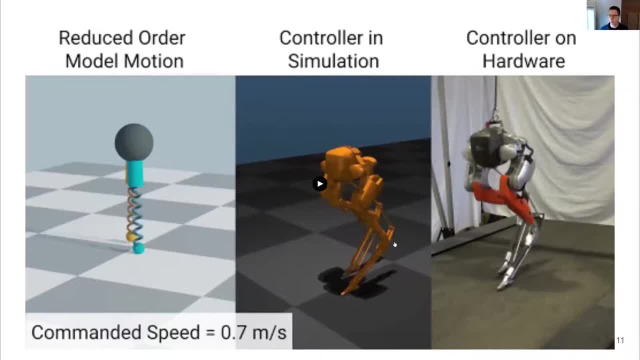 we're working right now on, say, um, yeah, integrating planning and saying you've got, uh, certain places in the world where you can step in, certain places where you can't, and then how do you learn with some sort of planner to to do that? well, and- and we're exploring with, how do you learn? 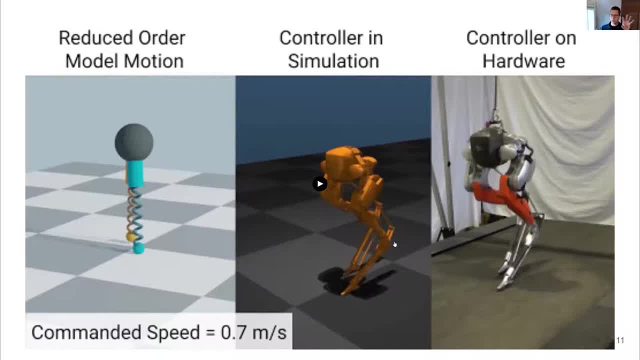 a planner, how do you set up the control hierarchy and have different pieces and sub pieces of learning, so it isn't a giant black box, it's smaller black boxes plus engineered systems sifted in, And it's interesting that if, for example, what you do is you specify the footstep locations that you're going to want, 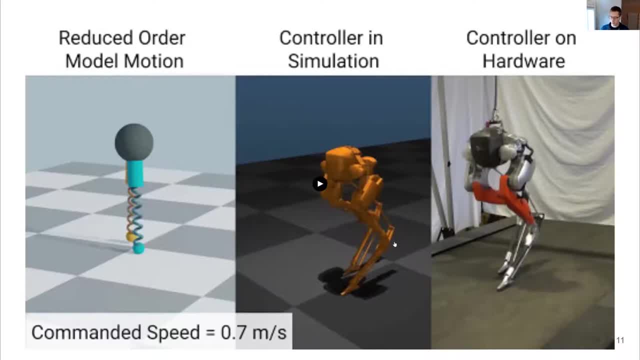 from a CASI robot, then you try to learn a policy that allows it to step on those. It may just not be physically possible for the robot to step in those locations that you've given it If there's semi-arbitrary locations on the ground and the robot just doesn't. 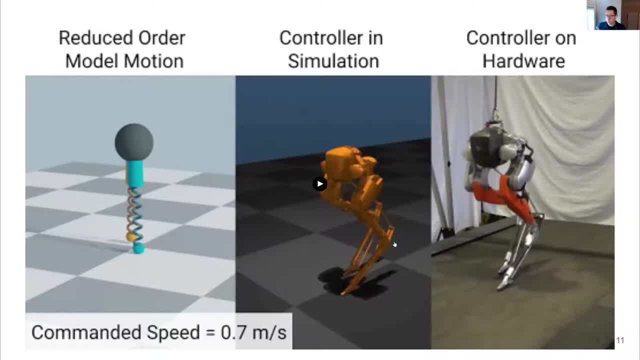 have the control authority from you know the foot placement is here and you want to put its foot there and it can't. it's not going to successfully learn it. So the problem is that the planner then is kind of stepping on the toes of. 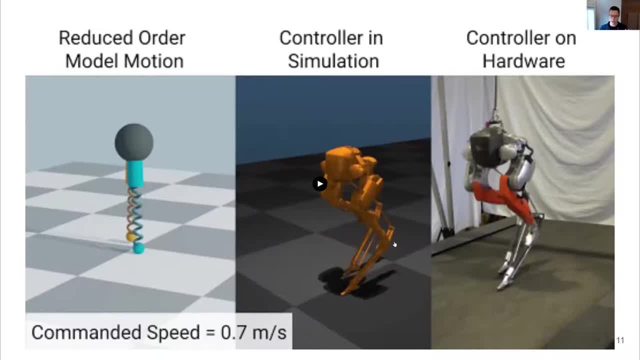 the dynamic policy. They're not integrated well. So you know we do have to find some way to plan through the dynamics. You want the system to. you know, if in two steps you want to be there, you're now going to need to place one foot here. 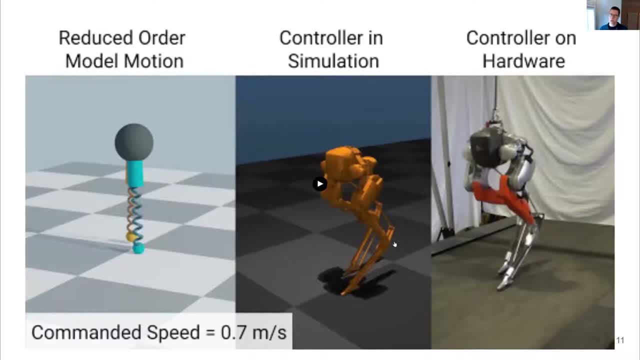 bounce through a certain, you know, set of directions and set it up so that the the next footstep location is also the right place to allow you to balance the machine and balance your robot as you're going. So the full dynamic model and the full dynamical system has to be part of 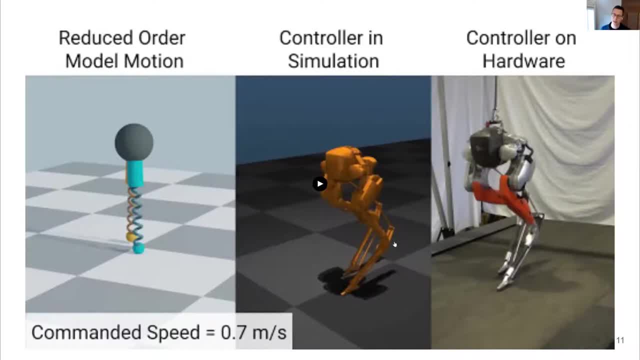 your planning And it's a challenge to understand exactly how to do that. We've done it on reduced order models, You know. we've done it where, if you just have a two or three step look ahead and you know what your environment looks like, you know. 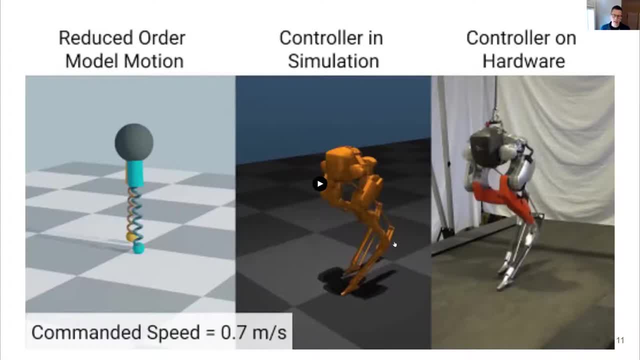 stairs or holes in the ground or whatever, And you have control over the amount of thrusts that you put into your extending your leg and the location of your footstep. It works really, really well on a simple actuated spring mass model in the plane. 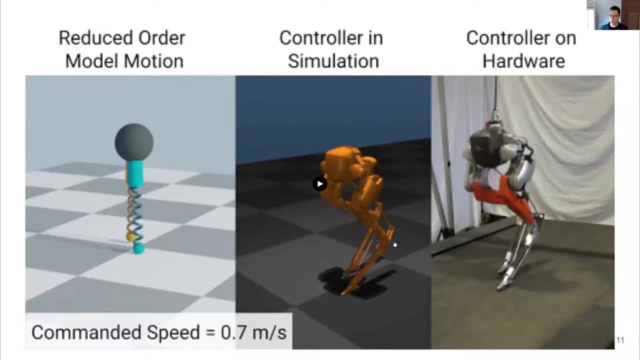 like with a Monte Carlo planner that's just figuring out its way forward And so increasing the complexity of that a little bit, so that it works in 3d, perhaps on a reduced order model, And then figuring out how to put that on a full. 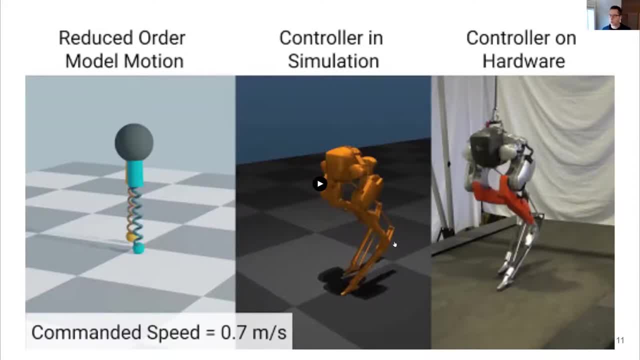 full robotic system. You know where? maybe learning helps us translate from the reduced order model to the to the robot. Yeah, It's going to be a control hierarchy of some sort, but it's going to have to be a pretty capable planner that doesn't give. 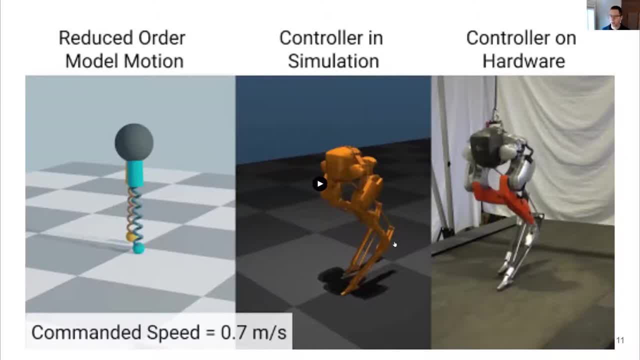 infeasible or dynamics blind plans. Yeah, Thanks, Okay, Ludovic. Yeah, There's questions in the chat for me. Maybe ask the questions in the chat first, but then I can. I can go, Okay, So the 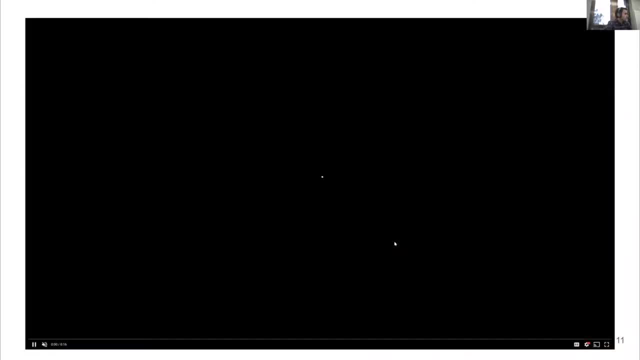 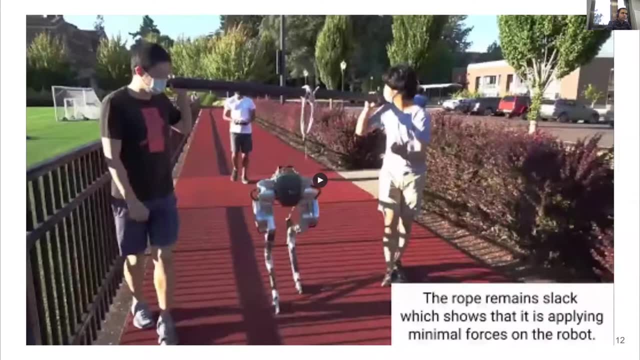 the first question is: for the instance of this gate transition, do you have some preview horizon for the policy to know what's the next coming gate? Let's see. The short answer is: I'm not sure what. have to ask my students about that. 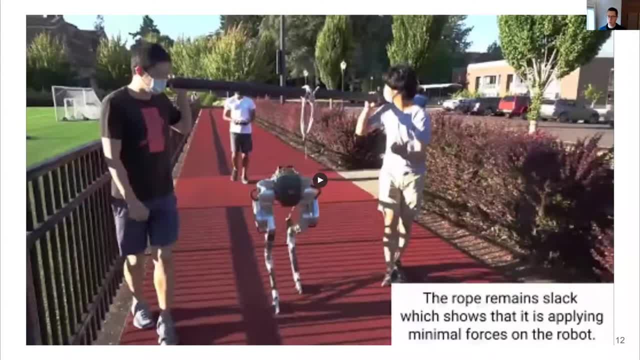 I don't think so, though. I think it's just got kind of a periodic behavior, and you know when they switch to a new behavior. I think it just it waits until the next time there's a transition for that transition to implement. 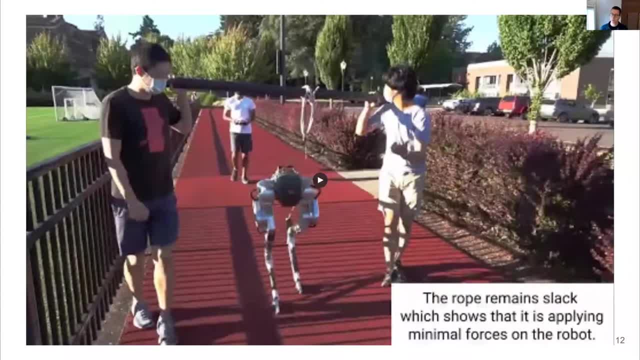 But no, I don't think there's any. there's no planning involved, or no? no, look ahead. There's just an input of the clock cycle And then the system is trained with that clock cycle changing at arbitrary times, And so it can change any time and it's fine. 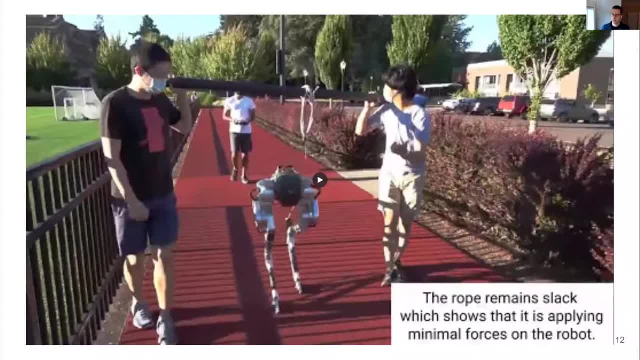 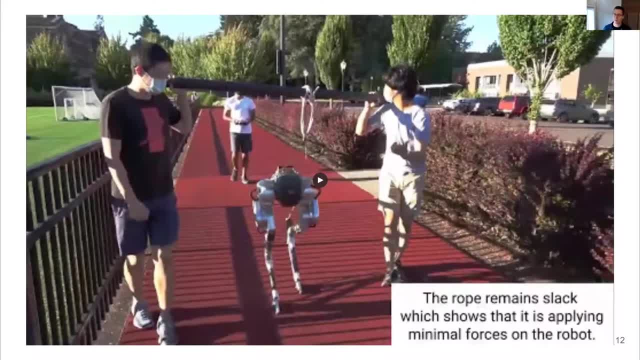 I don't know. I mean, I'm sure it's going to be part of the thing. That's the thing, right, You can't just do this as a black box. You can't say: okay, robot, I want you to learn how to walk across this room. 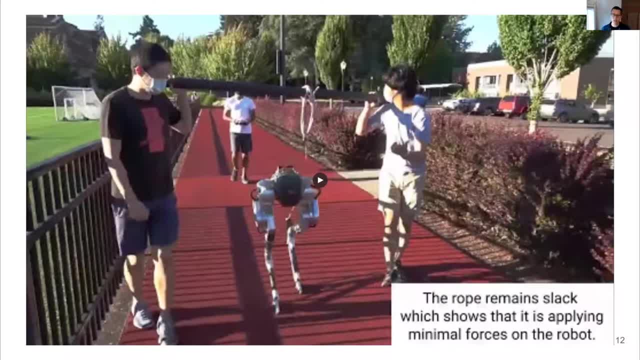 pick up a box, carry it over here and set it down, for many reasons. One reason is there's too many degrees of freedom and too many decisions and things like that. It's there's decision points. The learning seems to work Well for representing a set of dynamics. 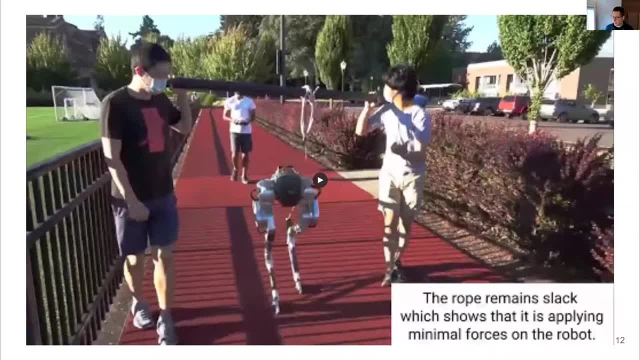 but not for like decisions. But even if it could, it's only going to work in that one situation that you, that you learned it for, And so you have to have a control hierarchy of some sort, with planners, with inputs from the user. 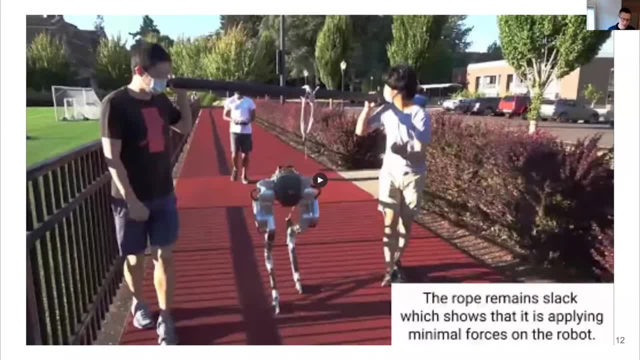 from the world And you're never going to get away from it being an engineered system for the robot for, for, say, digit, the robot, the software, is at least as big of a project as does Finding the hardware, At least, I would say, at agility robotics. 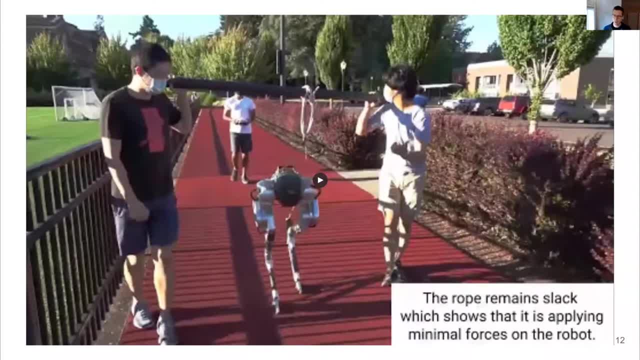 we are transitioning from being primarily a hardware company- to get the dynamics right, To figure out how to implement the engineering of a piece of hardware- to a software company where really the majority of our focus and effort is on the software, the control, the control hierarchy. 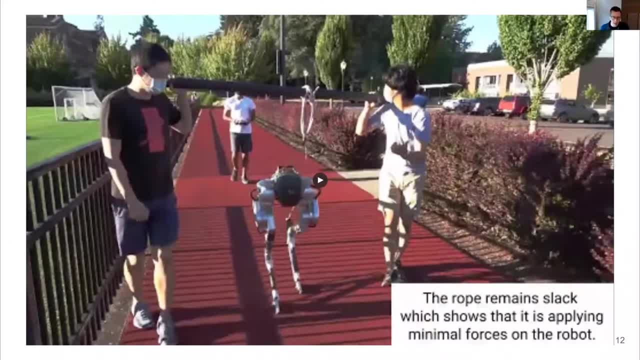 the perception, the integration and the mapping and the user interface and all of those sorts of things. So filling out the control, the control system, is no small thing, Right? The next question is: how do you compare the learned behavior to to the behavior of animals? 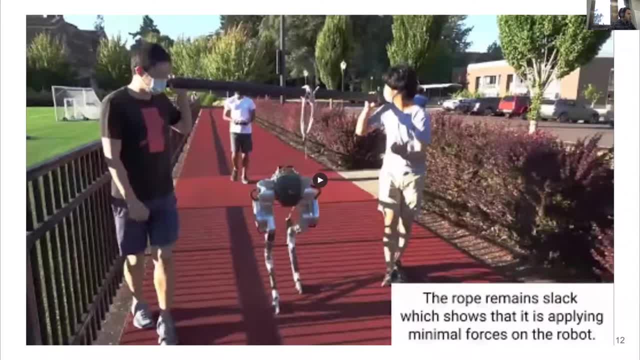 For example, this twisting leg, also for contracting the body rotation. Do you think that animals use the same technique? That's a good question. I don't know if animals use the same technique. I know that all, all bipeds have some way of applying torque to help them with it. 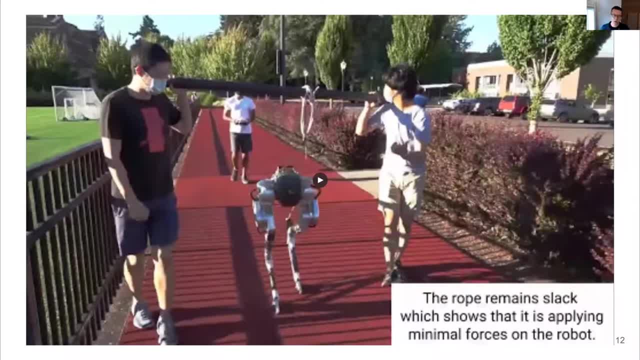 Quadrupeds have a much better time of changing their, their, their yaw. but you know, you look at, say, birds, and one theory of their evolution is that the whole reason they even had wings was to help them be more maneuverable while they're running. 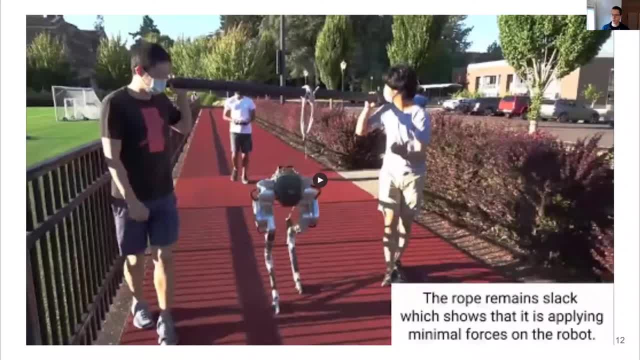 And certainly if you watch an ostrich run. when they are running and they take a turn, they stick a wing out. you know it's a big air break and then they're able to turn a lot more quickly and a lot easier. 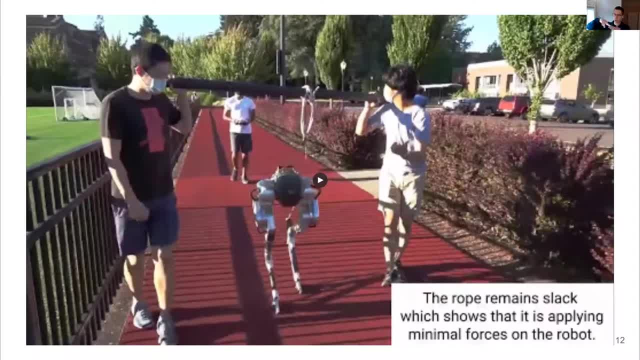 And ostriches really only have this very low inertia tip of their toe that's on the ground all the time to deal with those, those impacts over and over Humans have? I don't know, Humans are recently grounded, hairless monkeys, you know. 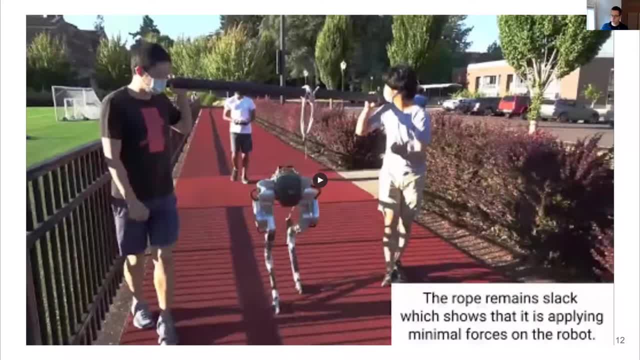 that really kind of have a lot of evolutionary baggage from climbing around in trees, but still- and we're pretty unique in terms of bipeds in the world- Most everything else looks like an ostrich or, you know, a bird of some sort. 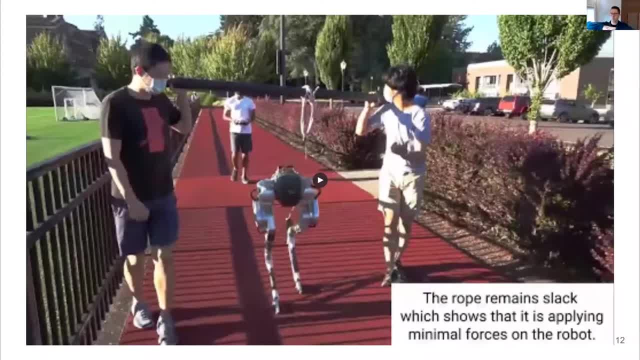 but humans have these great big feet that can play up, be on the ground and be applying, applying torques, plus our arms for inertial actuation. Cassie just doesn't have any of that history. You know it's designed by engineers and we definitely missed a bunch of things. 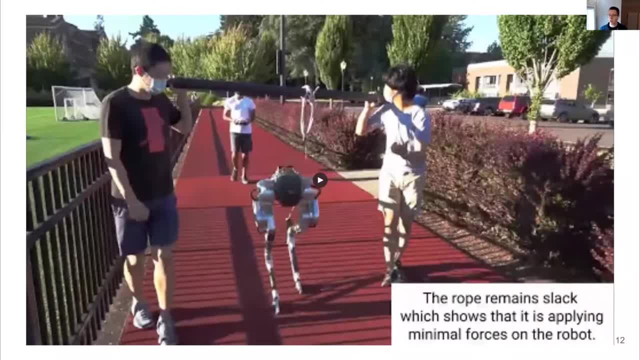 One of them is: you know, the foot's not that great. It's a piece of metal with rubber on the bottom of it, And so it's not going to grip the ground nearly as well as a human foot, And we have no other control authority. 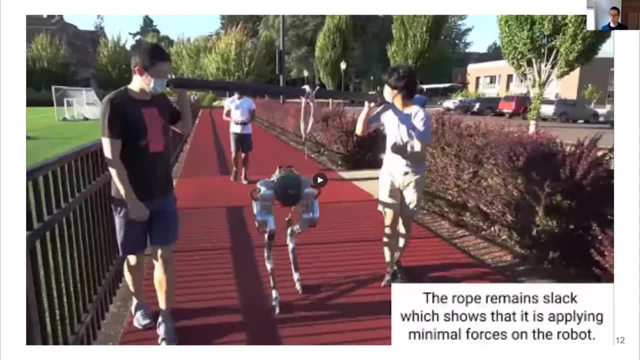 We have no arms, we have no wings, we have no gyro reaction wheels, We have no. you know we we could put quad rotor propeller thrusters on the robot and probably really improve the behavior quite a lot and run faster. 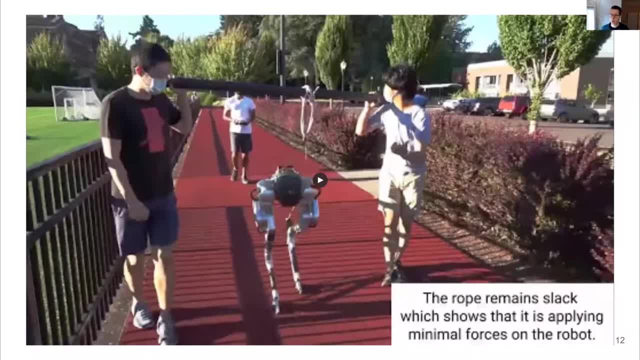 Even if the thrusters do nothing but control the yaw of the robot. I think we could get Cassie to run a lot faster with with like quad rotor thrusters on it. So some of the things that we're going to see like that twisting. 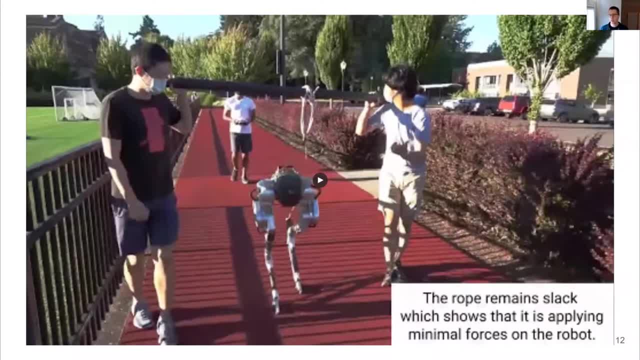 when it puts the foot on the ground may not have a biological counterpart, just because the hardware is very different from, even though we try to get it to meet the same physical principles as an animal, but we don't succeed, And in all cases, 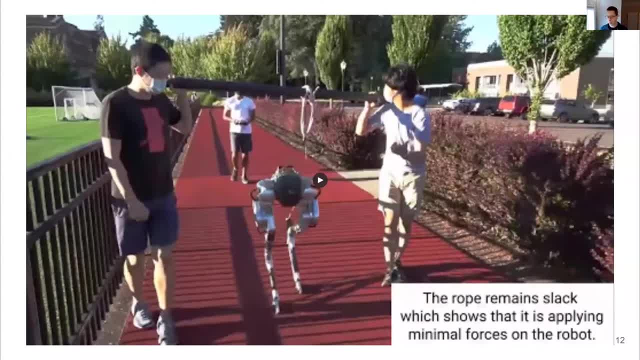 we've got a long ways to go to make it really, really good. I would say that the way we look at it is the same way biomechanics look at an animal. We here's an example. years years ago we were. 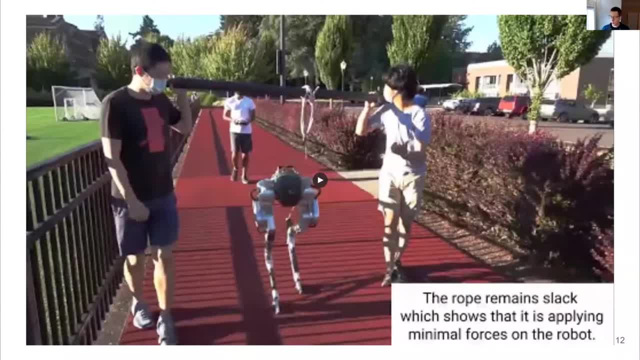 I was working with Monica Daly She's works- She was at the Royal veterinary college at the time and she works with a ground running birds- And we were looking at the policy for swing leg retraction when birds are running off of a drop step and then relating that to spring mass. 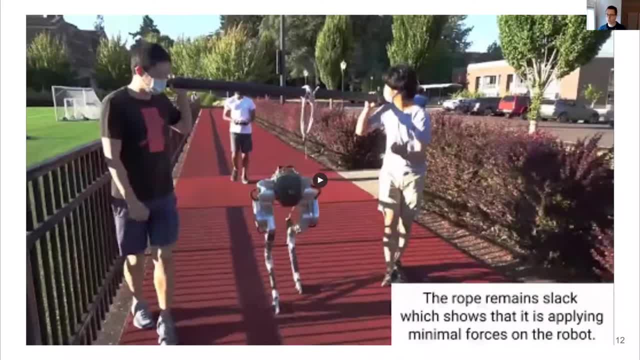 models and trying to understand what's the right policy and what are they prioritizing and what are they looking for. And you can't there's with a control system. you know what you designed it to do. with a learning system, You don't so much. 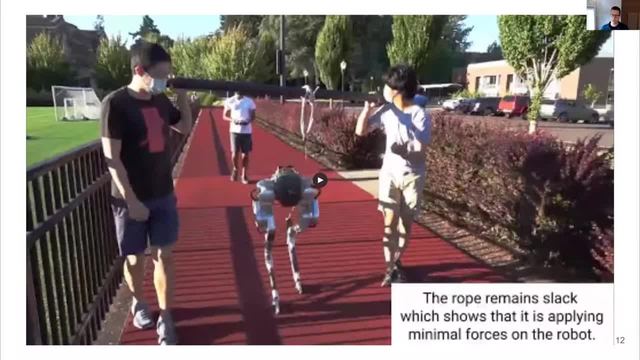 And with a bird of course you don't, you'd have to have your observations, And so with the bird you know, we, we, we can see what the trajectory is. And then we had a bunch of hypotheses that it's trying to remain an 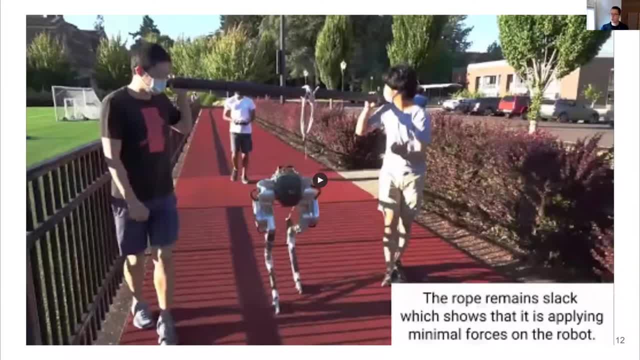 equilibrium gate, where this, as quickly as possible, returns to the original stride frequency, stride length, everything else, or it's minimizing peak torques, or you know what are the things that it's optimizing for. And we found very, very clearly what it's doing is minimizing for peak torques. 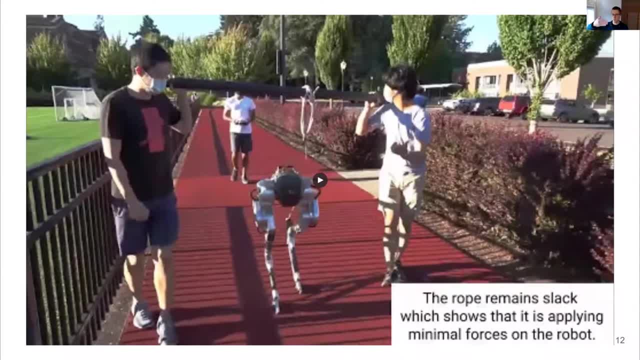 And when we calculated that so we said for a spring mass model at every instant in time as the leg is coming down. if it hits the ground now or now, or now or now, what angle would it need to be for the subsequent stance phase to? 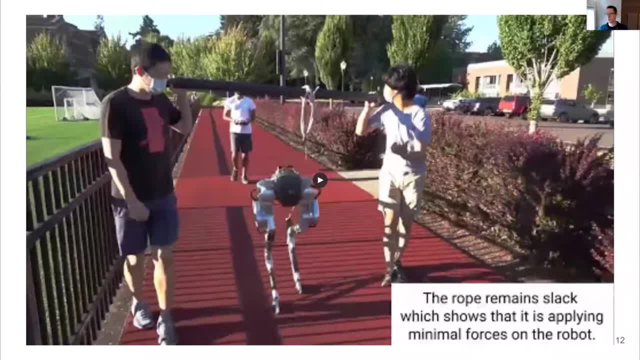 have a peak ground reaction force, the same as what it was before, And then that calculated out a trajectory For what the leg retraction policy should be, So that is called a pre-flex. at any point, If it hits the ground, you're going to get that ground reaction force that you wanted without having 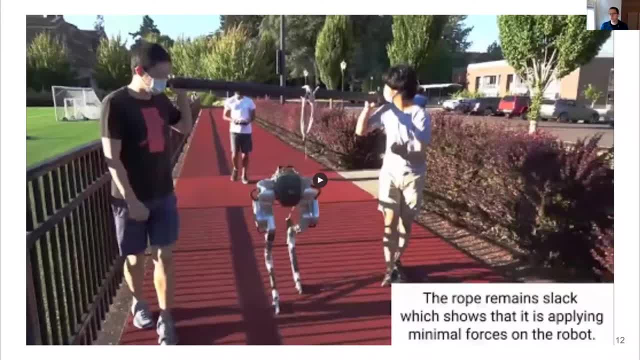 to plan for it without knowing what it's about to be, because you're basically preparing to hit the ground anytime unexpectedly, And we found that that trajectory very closely matched exactly what birds do, And so then that's, you know, that's an important policy that we would like to then implement on a 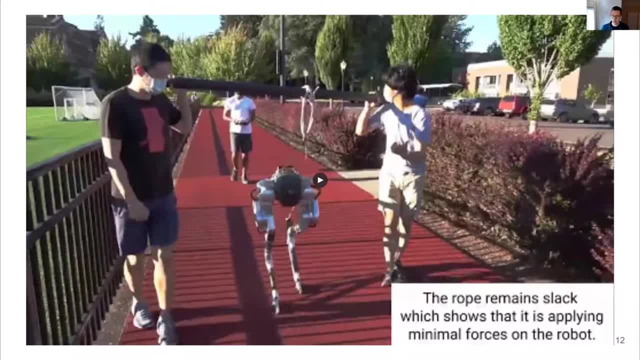 machine. And the way to do it with learning is to say: okay, we know what the priority is. The priority is to minimize torque squared for this particular trajectory and this set of dynamics that you would expect to see. That matters for energy efficiency, that matters for not breaking things. 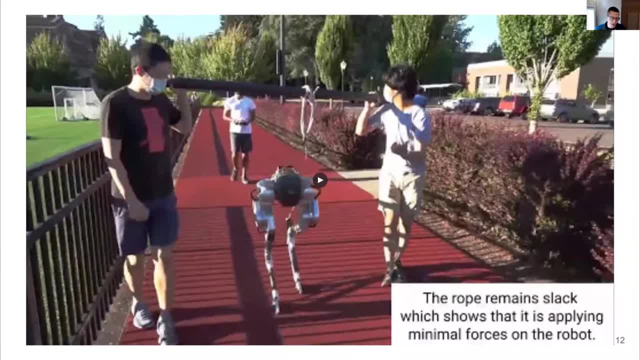 you know and so on, And so I know it's not simple and there's a lot we a lot we still have to learn. but that's kind of how we look at this. What are the fundamental physics? What are the things that really matter about the gate? And what are the things that really matter about the gate? And what are the things that really matter about the gate And what are the things that really matter about the gate. What are the first principles? And we can get a lot of hints from animals. 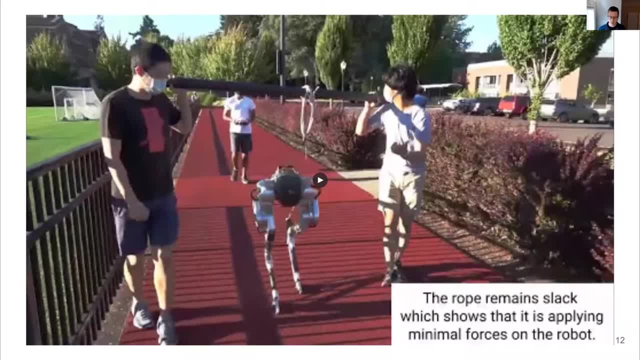 Then we try to create those cost functions and try and describe the problem, which is how, the difference between learning and an engineered system. with an engineered system, You're trying to write down the solution And it's a little bit guess and check, Whereas with a learn system, 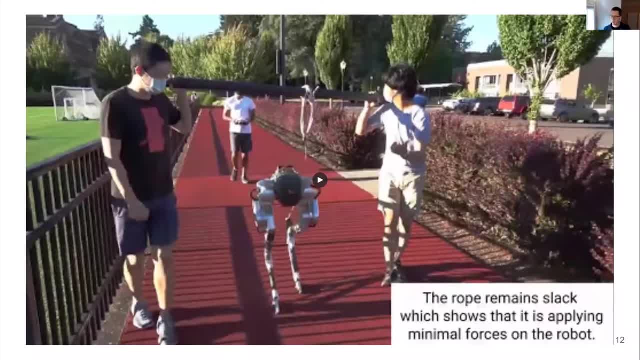 you can write down the problem. you can write down you know, and and what the answer looks like, but you don't get to write down the solution. The learning system has to figure that out. So the next question is: how important is the robot design in order to use a sleep model? 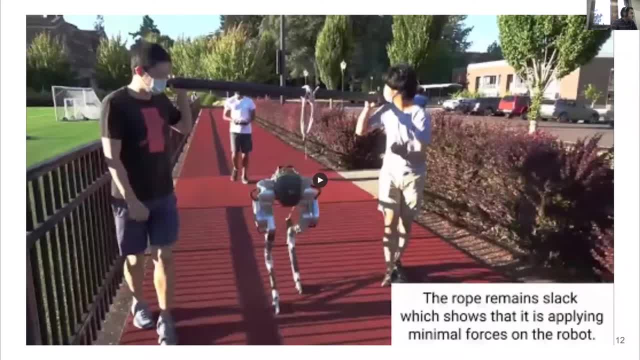 For example, if I use a robot that does not use a sleep inspired design, can I still get similar behavior? Short answer: No, you can't. There's a saying that I like, that a rock cannot fly, no matter what software you write for it. 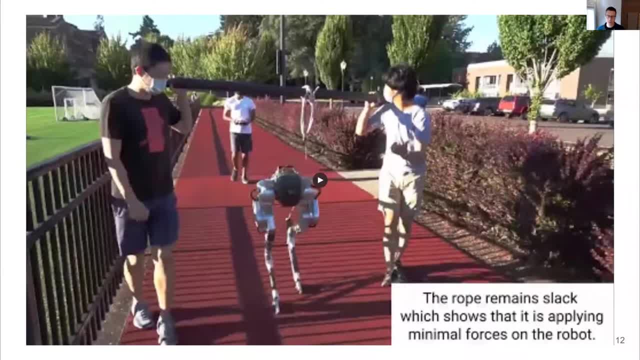 Unless that, you know, the physical hardware is absolutely, absolutely critical and completely necessary component of the dynamics and the behavior of the system. It's, there's no way around it, If you have a, you know, a robot with 200 to one harmonic drives at each joint. 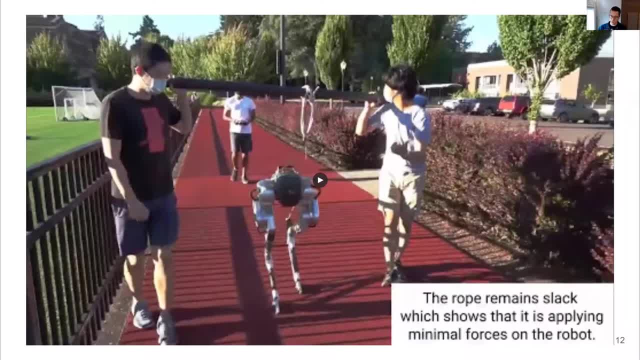 you're going to have a very high reflected inertia when it impacts the ground. And that's just physics And it doesn't matter what software you write, that inertia is going to be there, That impact is going to be there and it will not create. 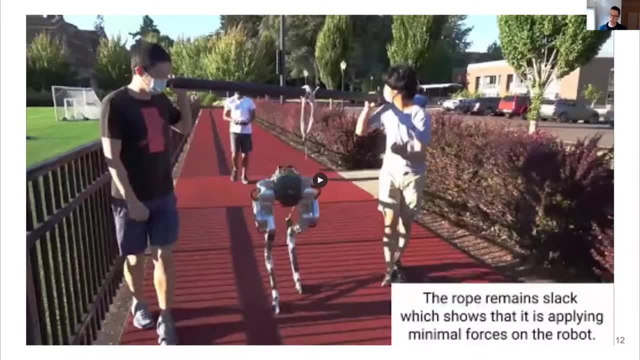 the dynamics or the behavior that you want, if the actuator dynamics are in your way. So now is necessary to first define the behavior that you want and understand that, then design the hardware such that it will be able to achieve that And then design the software that works really well and is an integrated 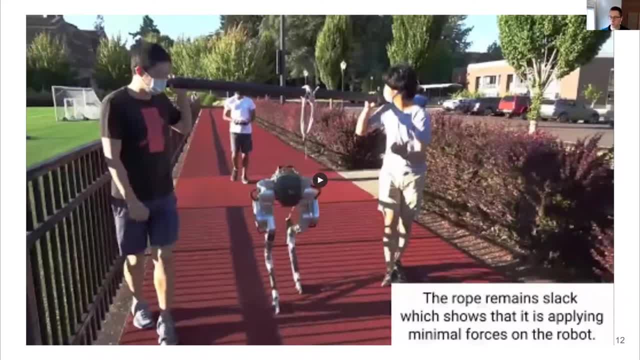 part of the design, with the hardware to create the behaviors. Very good, Ludo, do you want to go with the next question? Sure, Thanks, I really enjoy your thoughts a lot. So I really very much agree with your, with your systems view of designing. 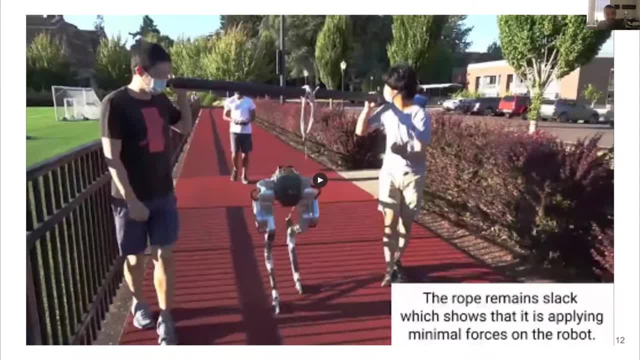 you know controllers of systems for robots in general. But along those lines you said something that struck me during your talk. You said, Oh, this thing works really well, but we never know in advance how well it's going to work. 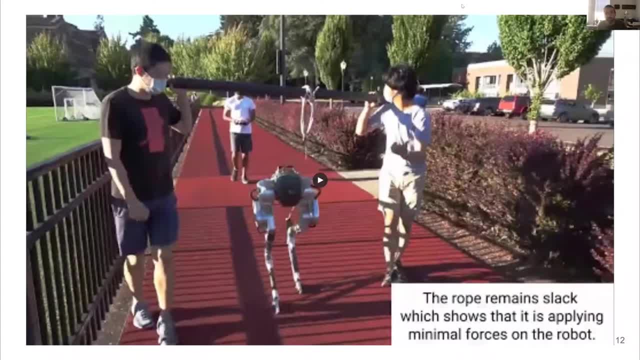 And this kind of struck me. Maybe I think it's really true for many things we try, but it's especially true for a lot of the RL stuff We actually try in my lab as well, And I was wondering if, from the experience that you have, 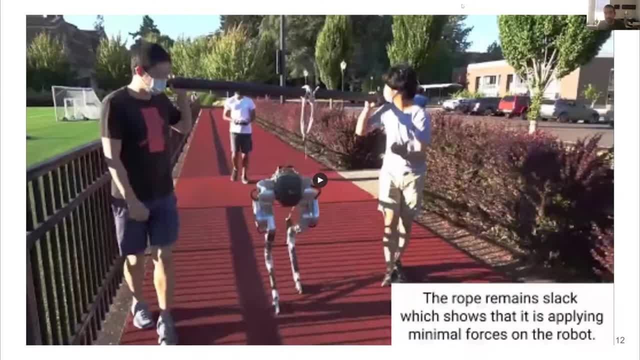 if you can come up with methodologies or you know formalism that allows you to maybe know what is going to work and how it's going to work, And you know. basically we need principles and methodologies and just not just try things around. 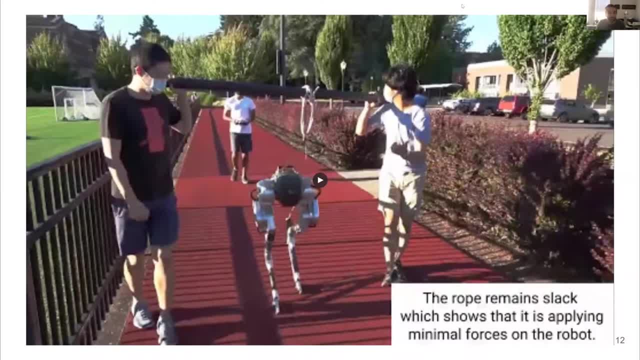 And I was wondering: what's your take home on that? I don't know. That's a hard question. This recent transition in my lab to reinforcement learning- the whole the philosophy from the very beginning has been: we don't want to innovate on algorithms. 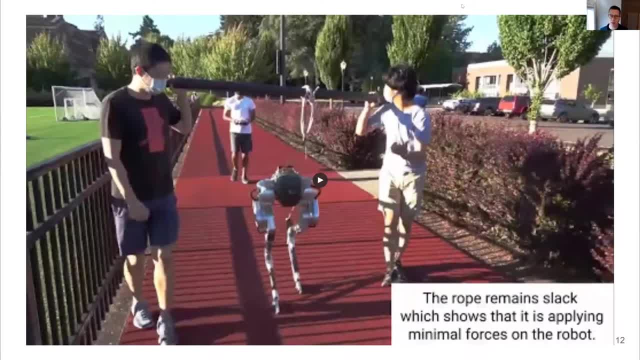 I mean, I'm actually not a computer scientist, right? I'm a mechanical engineer, background in robotics and biomechanics and physics, understanding of dynamics and how, like locomotion works, but we want to use any tool at our disposal. So 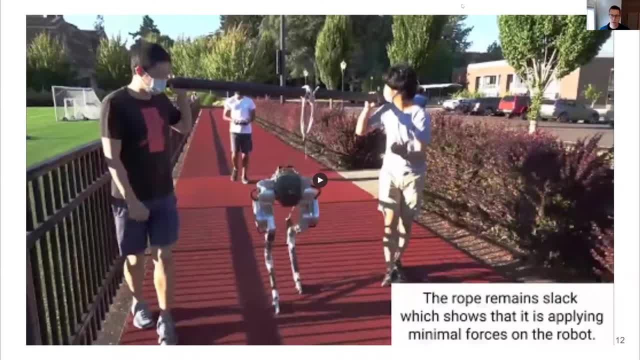 you know, I started a collaboration with Alan Fern, who's an expert in machine learning but doesn't not an expert or any knowledge of like a locomotion. And then we started finding students and recruiting students who had a lot of background in 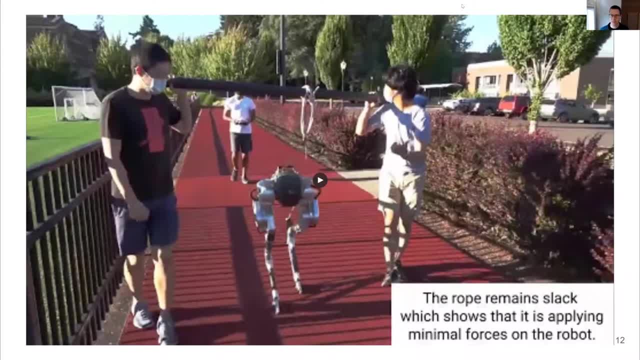 kind of both areas, So that kind of like at the dynamic walking conference. you, you just put classical mechanists, biomechanics people and computer scientists on an Island together and then they're forced to talk. That's what I did with my lab. 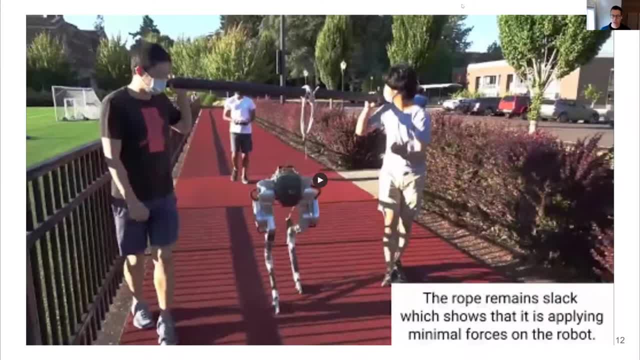 And so, you know, I asked students who were learning reinforcement, learning algorithms and techniques, to start trying things. But we start with the physics of like and locomotion. everybody learned spring mass models and the heuristic controllers and, you know, did a MATLAB simulation of spring mass locomotion and then controlling that. 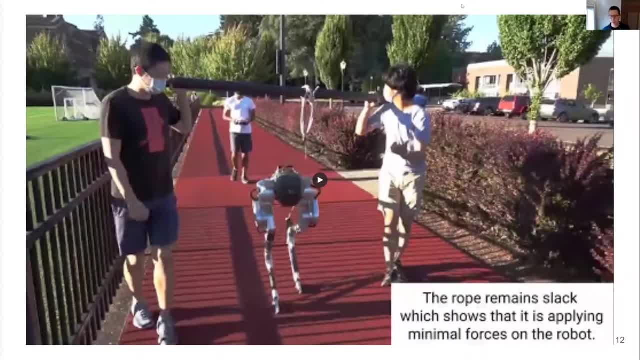 And then we've spent a long time- I don't think successfully yet- We're maybe 75%- there writing, trying to write down a definition of what is the dynamical phenomenon of like a locomotion. Can we define it? Can we list the facts that are true, indisputably, that fully describe what is? 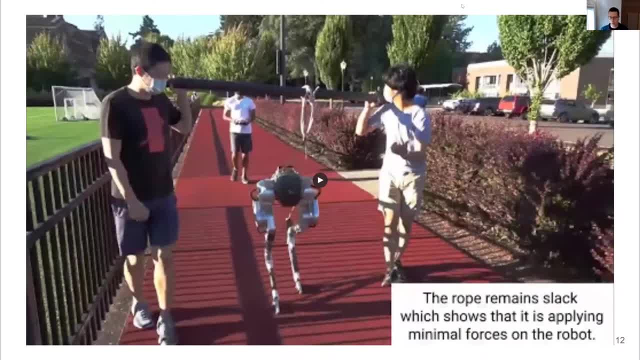 this behavior And the. the exercise then was to to just explore a bunch of kind of known tools with like a locomotion. but we know what the behavior is, We know how animals work, where we've tried to write down what are the fundamentals of like a locomotion. 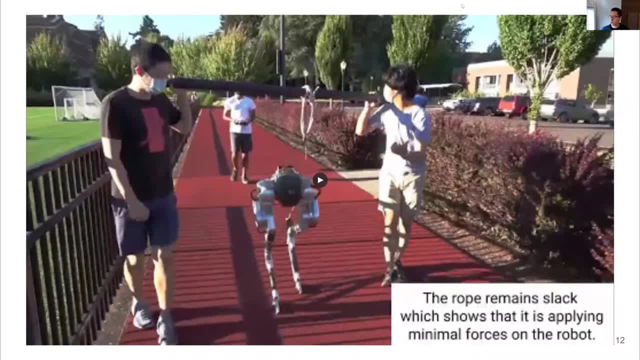 and what does that look like? And the challenge is trying to create the cost functions to describe that. And then I don't know, I've just those are the boundaries we put around it. And then we have, just like in this presentation, 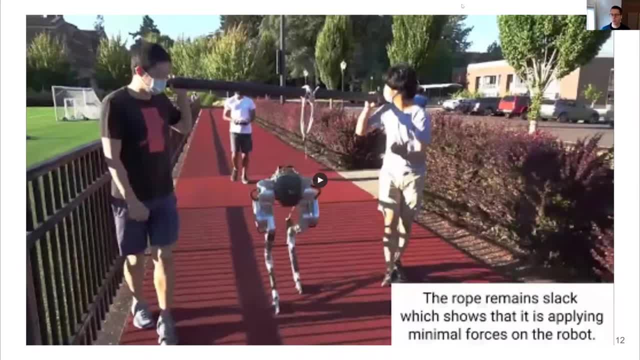 I showed four different directions that we've tried to see which one's going to be fruitful and which ones aren't, and why. And so it's- it's semi open-ended research just to say what's going to work. Let's try these 12 different paths. 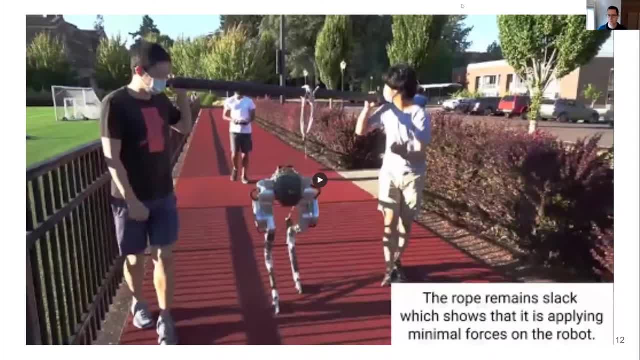 but within bounds, within constraints, And so the stair climbing one is an example where, well, honestly, the first time we were surprised is that we we got something learned in simulation and then it just worked on the robot, And then we looked around and 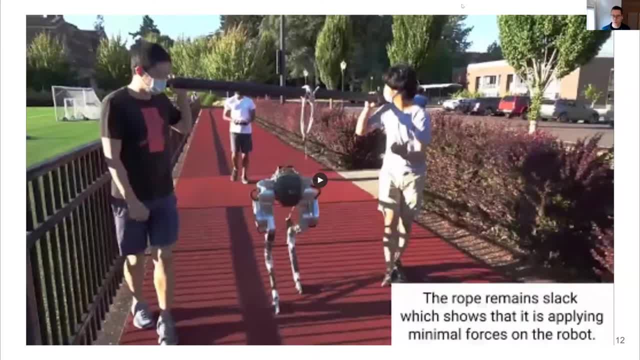 you know, find that SIM to real is typically a massive problem. for some reason It just wasn't for us, And I think that's I think the only reason is because the machine is designed for walking and running. Everything is based around the philosophy of legged locomotion. 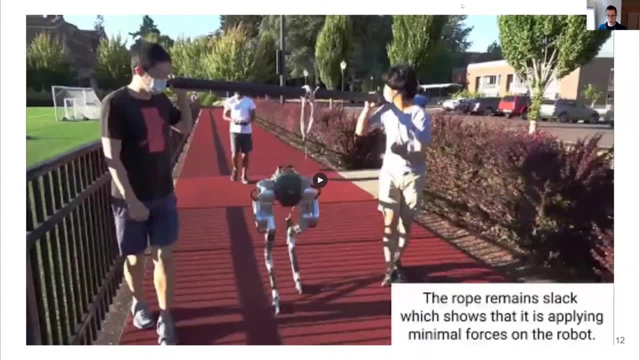 The hypothesis is that that's kind of a self-stable system as it is, and we're getting close to representing that, And so that's what allows it to be really robust when you go from SIM to real. it's not a sensitive system instead of dynamics. 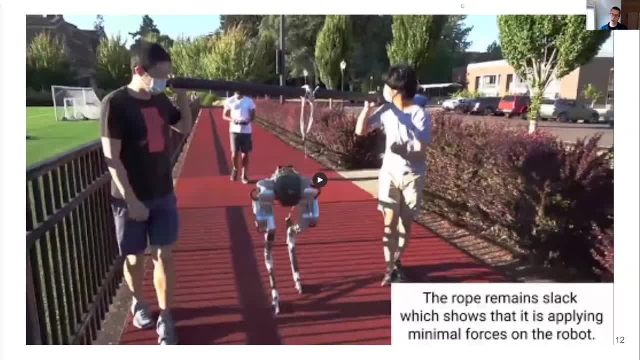 And then the next surprise is going up and downstairs. I did not expect a completely blind learn system to just be able to walk up and down stairs reliably. That's crazy, but it's pretty exciting. So I don't know if that's not a good answer that I'm telling you what we did. 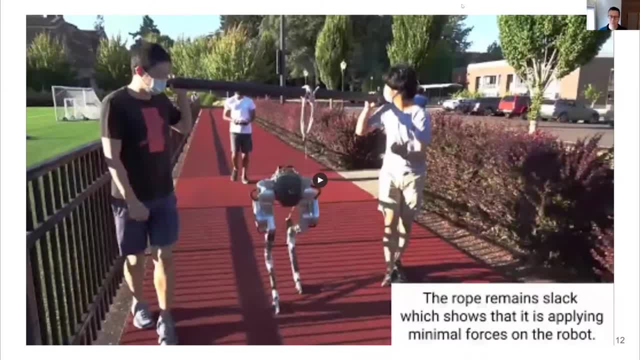 but, um, I don't know. Yeah, I think it makes sense. I mean, it's the same right We try and try to come up with, understand what works and what doesn't work, And I liked the fact that you're constraining that with physical principles. 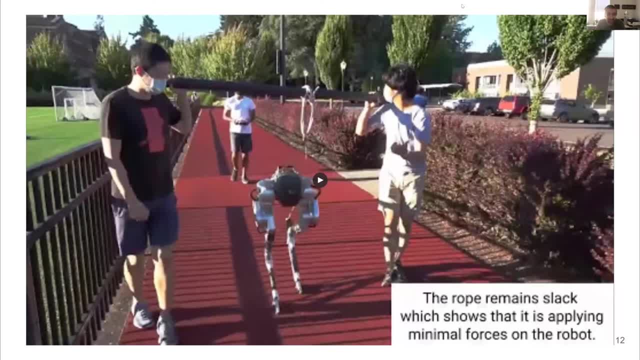 but yeah, thanks, Okay, Uh, I go with. the last question Here Is: uh, it's referring to uh part of your talk that you said that you don't believe we need to follow up uh a specific trajectory. 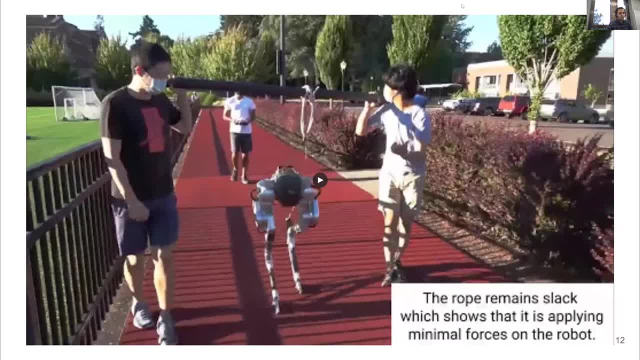 uh for a dynamical system, because if the conditions are different, like the touchdown time, uh, it would not possible to track the trajectory. Now that all of this policies are by by design, are, has it stayed feedback so they can handle possibly this situation? 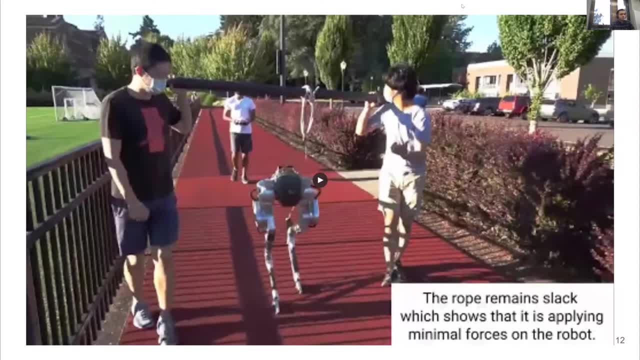 What do you think about the MPC methods? Well, I just think the command shouldn't necessarily be position trajectories. There's lots of other kinds of trajectories. You can command force trajectories. Um, what we did that worked really well. the first time is actually command set point. 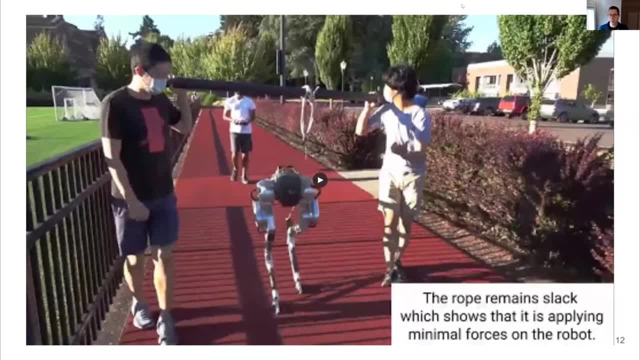 trajectory. So, uh, every joint has, uh uh, a PD gain on it and a set point. And if you actually control both the gain and the set point, you control the stiffness, the damping, and the set point, the virtual set point. for that, 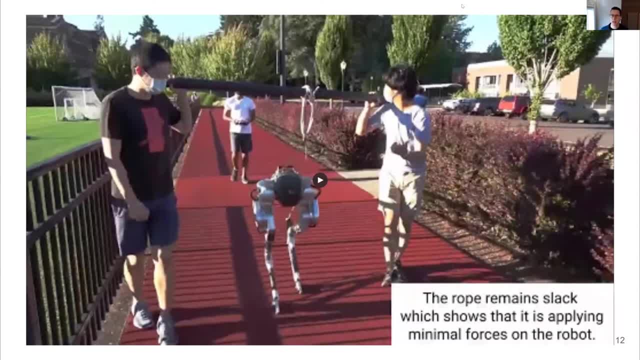 for that joint Um and those gains, the stiffness and the damping, or maybe a little, a little low, you know, not ramped up as stiff as they can get, but a little bit lower. um, you can control the impedance and 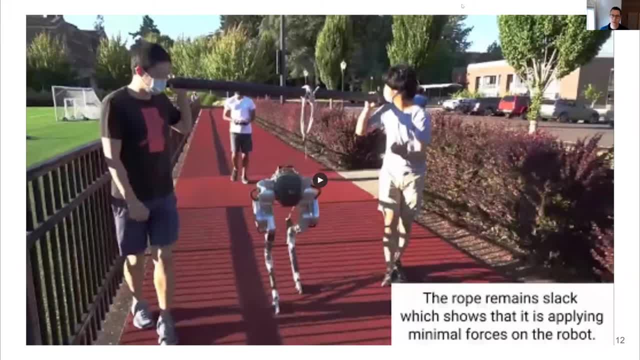 and, uh, much more of a dynamic behavior of that joint. That was very successful. Um, everything kind of boils down to set points and stiffness is anyway um for any real system. whatever you're trying to do, if you've got feed forward forces. 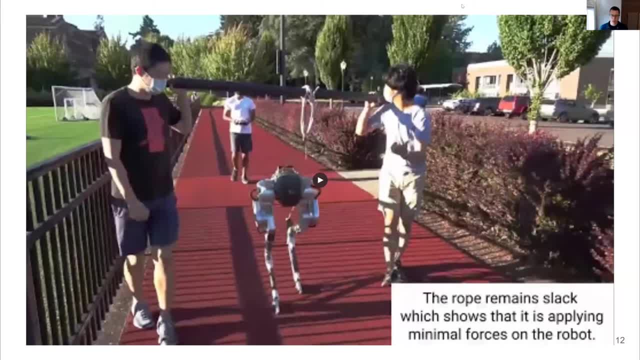 or if you're trying to command positions. fundamentally, all you can do is control. you know the current in your winding, which is the torque Um, and all you can do is measure the error from what you want and then try and. 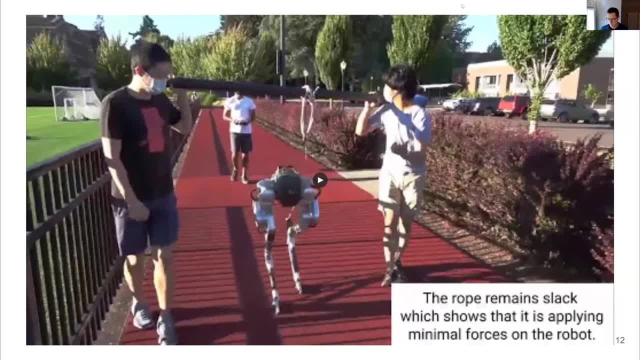 correct for that. So you've got gains and you know um, mathematically it's all becomes equivalent to set points and, uh, stiffness is anyway, Um, so I don't know. Uh, we, we've done some really early studies with. 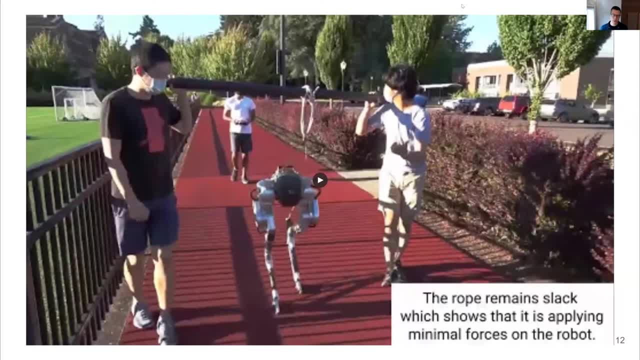 with like a spring mass system where it's a clock based force profile, Um, and that's the command in series with the passive dynamics of of the spring, the physical spring there, And there's some really nice kind of stabilizing properties of that. 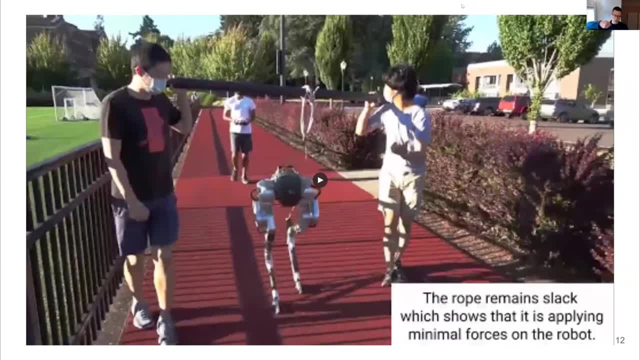 Basically, you're in the air and then you expect to hit the ground right now And your clock says start applying forces, actually not on the ground. There's a hole there- but the result of that is the leg shoots down to the ground as 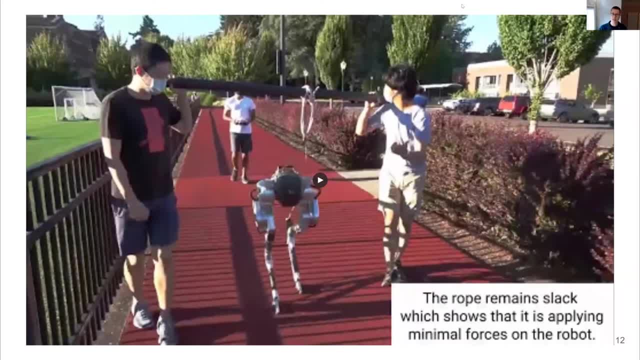 quickly as it can because it wants to apply a force, And so it extends the leg until it does make contact with the ground, And so that's sort of um, a pre-flex that automatically stabilizes the system and applies the force as quickly as you can, without having to have sensed your. 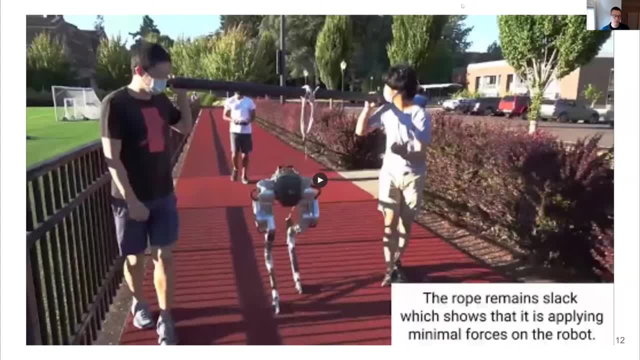 whole environment precisely and accurately. So we've got some video of Cassie as an example, um, where we do have planning on top of all of this and we're going upstairs And so there's like, uh, the plan says there's no camera on it. 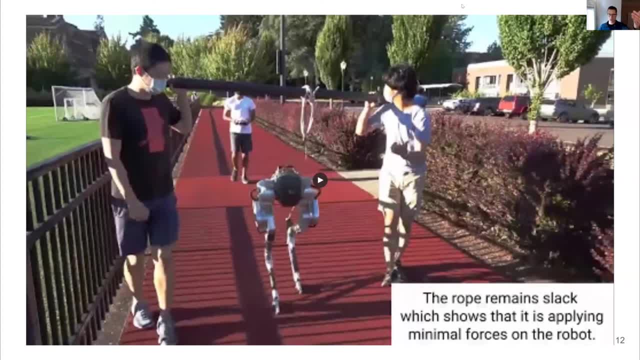 but we started a certain location and it has a CAD model and it expects three steps, but really the the piece of wood in front of it is only two steps, And so the robot goes up to two steps and then tries to take another step. 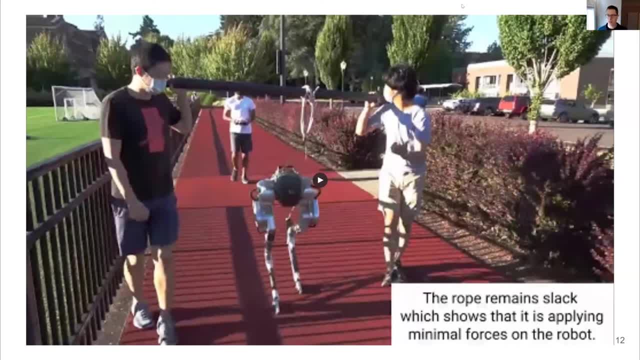 Which isn't there, misses and then just puts his foot down on the ground, And that's a familiar feeling for any person who's going upstairs and misses a step. Um, but if we were commanding position trajectories, you know it would lift its foot up.